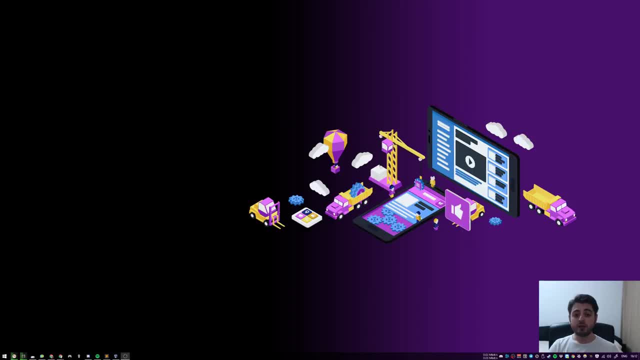 but what about loops? And what do loops have to do with recursion? Well, recursion is a term when a subroutine calls itself, and if it does this multiple times, then you basically have a loop. Now there are a few things that I want to mention before we start with this video. 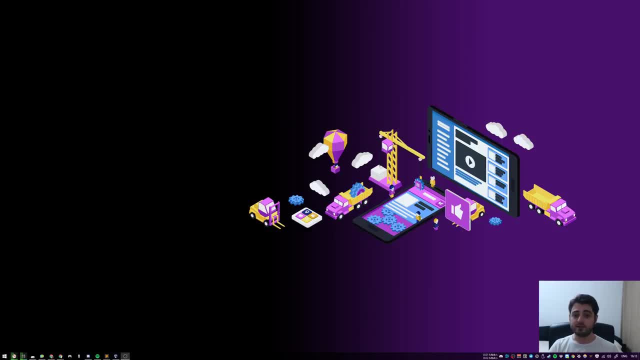 Now, recursion is a very complicated topic and beginners usually hate it, so if you don't understand this video, watch it a few times, okay? And the second thing that I'm going to mention is that it took me more than nine hours to prepare this video, so it might get like really, really. 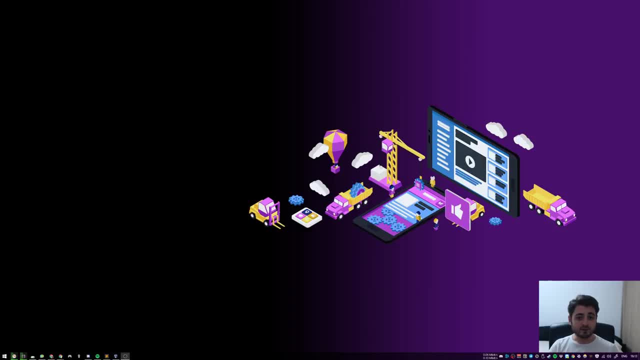 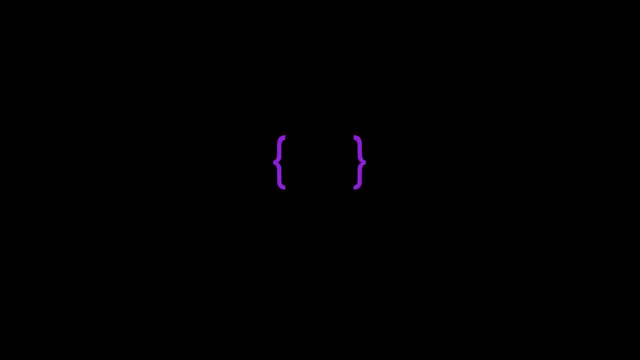 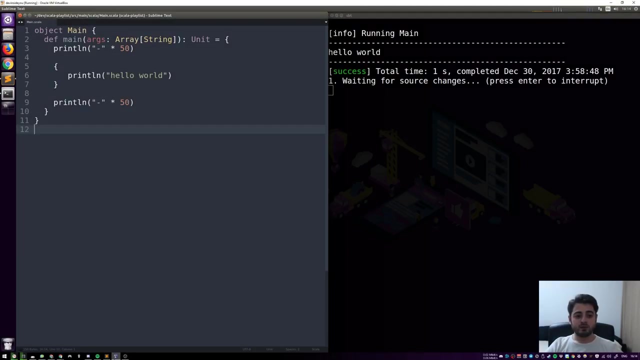 long. So if you see something like part one in the video, then it means that somewhere in the middle of it I had to cut it okay, and upload it separately. As always, we're in Ubuntu and we have Sublime on the left and the Terminal on the right. 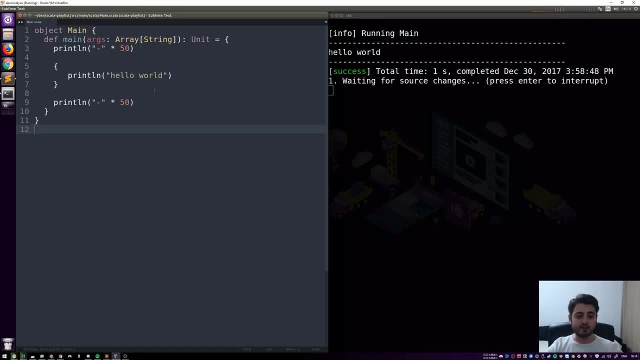 and it's doing this continuous loop where it just runs whatever we have over here. So I just said that recursion is when a subroutine calls itself. So remember, we had that def method equals method. right Now let's just call it and let's see what happens. 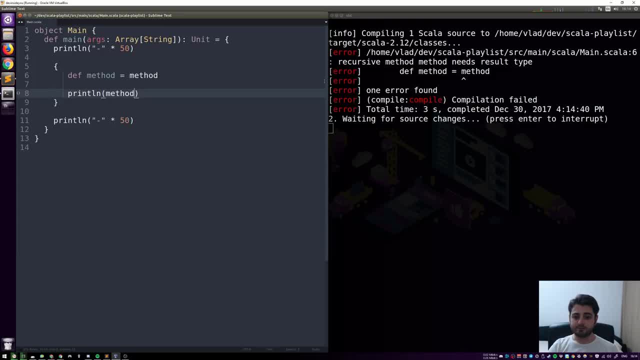 The first thing that should happen is that a scholar will complain. It says recursive method, called method, needs result type. okay, So let's call it method And let's see what happens. Let's specify result type. Let's say that it's going to be a string. okay, So now it's fine. 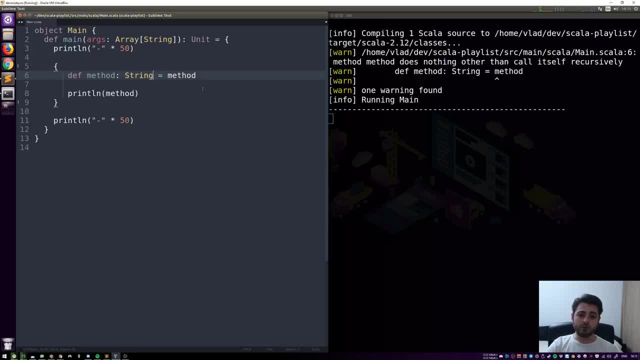 okay. The thing is that a scholar has a so-called local type inference, So in order to figure out the type of this, it needs to know the type of that, right? So it goes in and says, okay, so what's the type of the method? And if you don't specify that it's a string or something else, 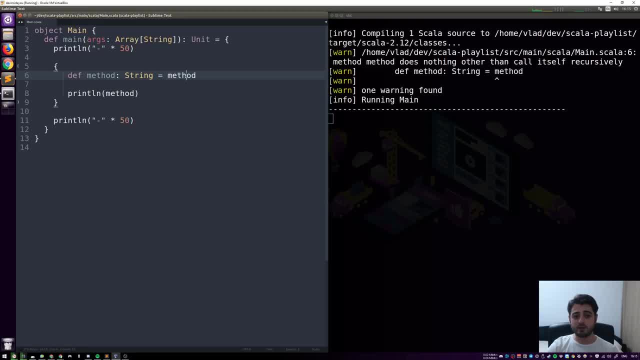 then it basically does not know what this is right, And because it doesn't know what that is, it can't know what this is. So it's in this sort of infinite loop And it can't figure it out. So basically, every time we have a recursive function, 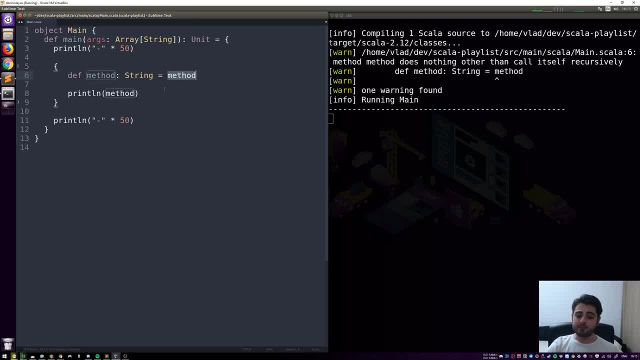 every time we have a recursive function, I'm sorry, then we have to help the compiler out, right? So we have to specify the type, okay. Now I need you to notice that what we see over here is this first print line, right? But we don't see this second print line. And it's happening. 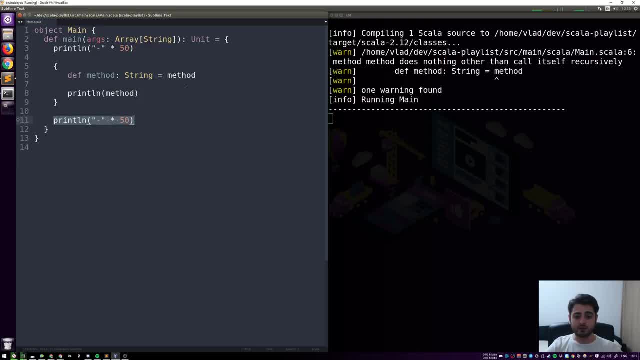 because the compiler is sort of stuck right. So, sorry, not the compiler, not the compiler. So the JVM is sort of stuck, calling the same method over and, over, and, over and over again. So this is what's known as an infinite loop, And you can always. 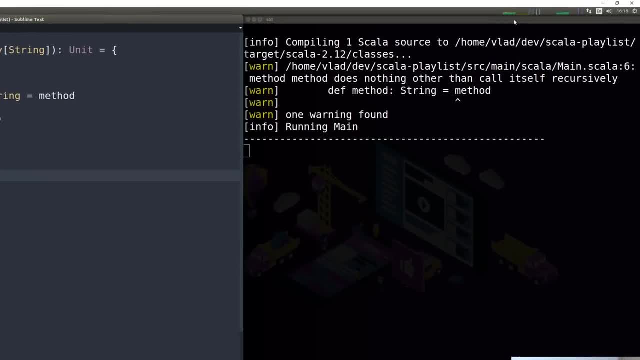 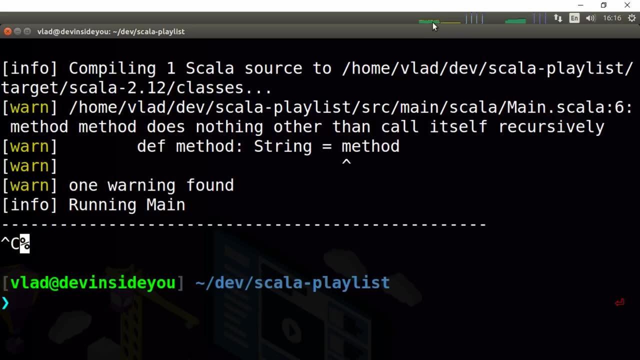 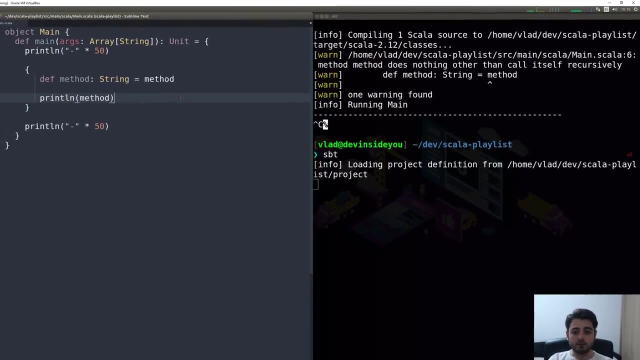 notice an infinite loop based on the CPU, right? So this is my CPU and it's running right now, right? So if I just kill SPT, you should see this thing going down. See, it's going down. So let me start SPT again, okay, And notice also that, because it got stuck over here, 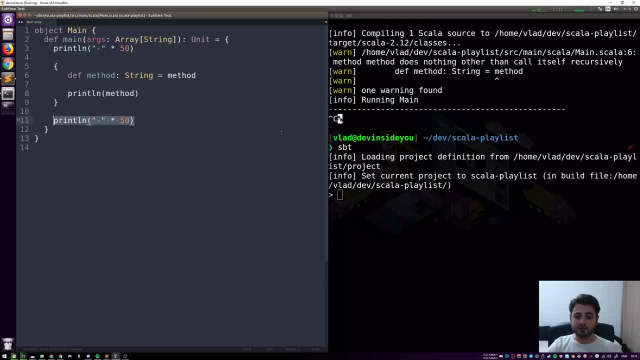 it never got over here, right, So it never showed the second line of hyphens. okay, So before we continue, I'm going to produce a situation like this- sometimes right, Quite- a few times in this video, sometimes on purpose, sometimes not on purpose, And I don't want to kill SPT every time. 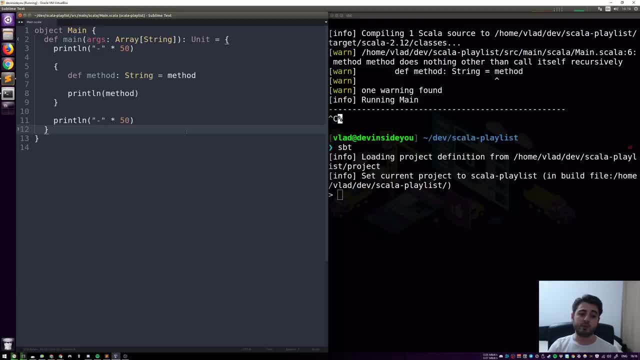 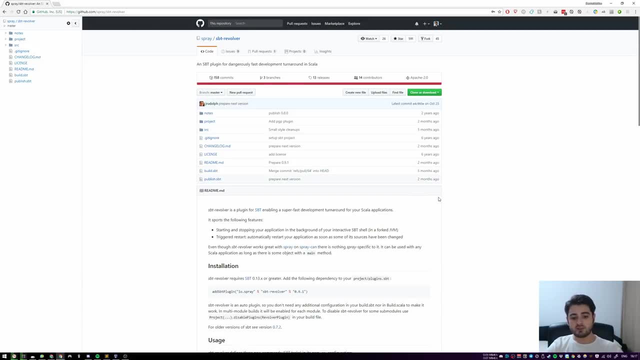 And therefore there's a very awesome plugin called SPT Revolver that we're going to be using. So if we go to this URL, githubcom, slash spray, slash SPT Revolver, and then we'll see this plugin right, And the way we install it is by having a file called. 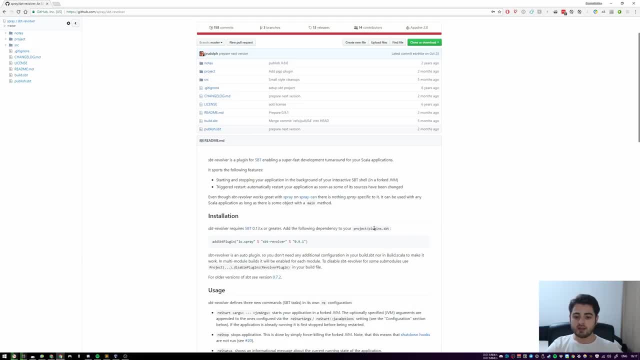 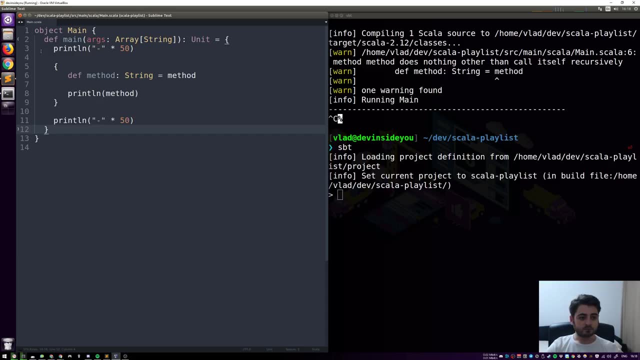 pluginsspt in the project subfolder And in fact it doesn't have to be called plugins, has to have an extension of spd. so let's do this. first let's go back to sublime. let's see our project structure and in fact it already has a folder called project and it contains only one. 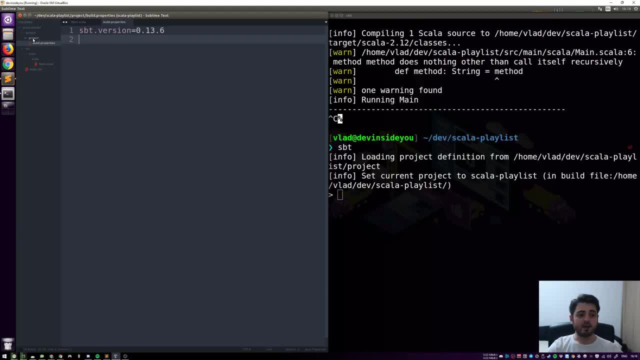 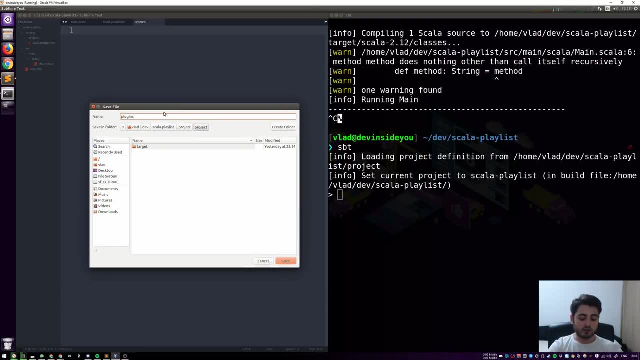 file called buildproperties, where we specify the version of spt itself. so let's create another file and let's call it plugins. what's happening? pluginsspt. now, as i already said, it doesn't have to be called plugins, it's just that the extension has to absolutely be dot spt and it. 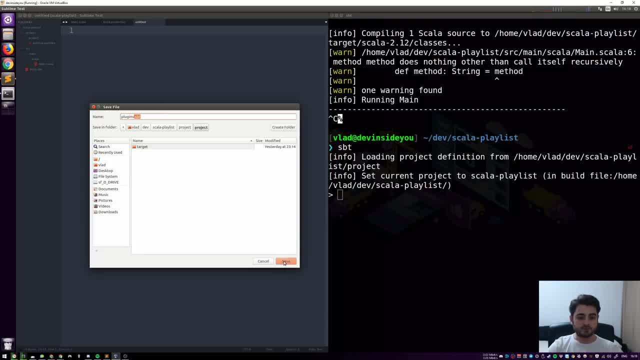 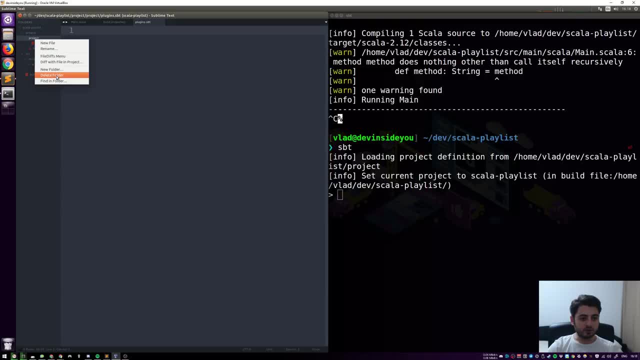 has to be in this project folder, right? uh, notice that uh, spt, when it's running, it also creates, uh, this empty sub folder. uh, we can, we can remove it, right, so, uh, so that you just see, see it a little bit better. um, oh sorry, did i remove the wrong one? oh no, i didn't remove the. 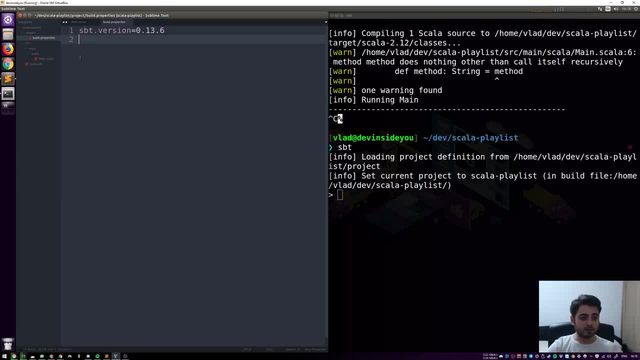 wrong one. i just created the file in the wrong one. okay, so let's close it. okay, so hold on. project new file: uh pluginsspt. all right, so it needs to be in this, in this project folder, right, but as soon as we um, as soon as we uh reload uh spt, which is basically the same thing as 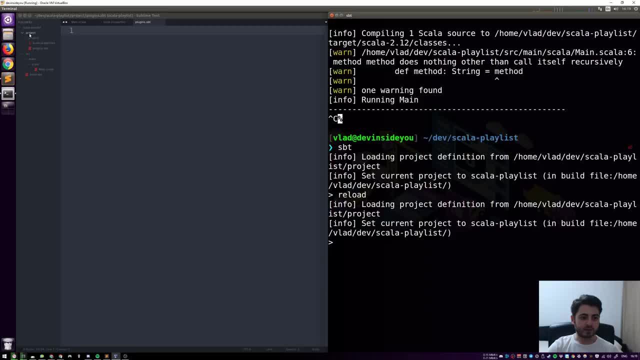 restarting spt. it's just going to keep creating this, um, this empty project folder over here. see, it's empty, right, so just just ignore it for now. okay, so, um, the idea over here is that you create a bunch of dot spt files and, uh, one is one of them is going to be for plugins and the configuration. 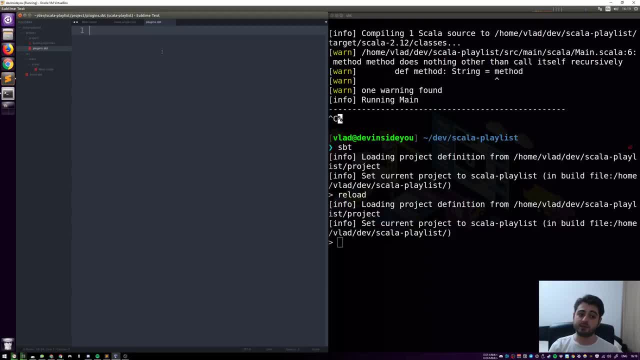 of the plug-ins and the configuration of the plug-ins and the configuration of the plugins and plugins. the other one is going to be for the settings for the compiler, for example, the other one is going to be for the settings for the jvm and so on, so you can call them however you like. 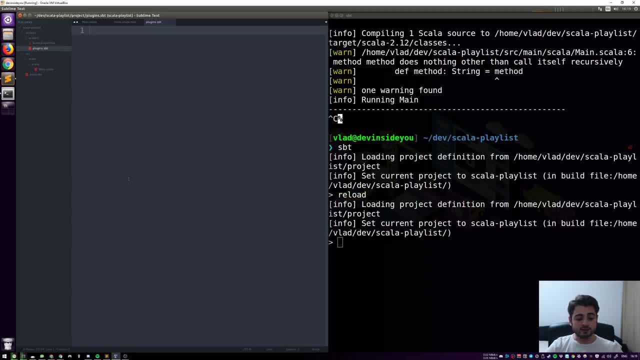 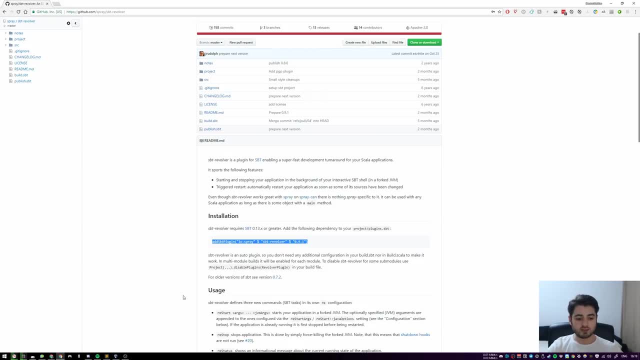 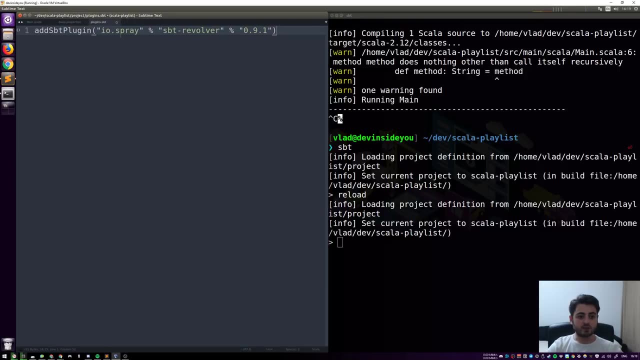 it just said they have to have the extension of dot, spt. right. so let's go, let's go back to the page and let's just copy: uh, this, so this is all that we need to do. we need to copy this line and we need to put it into this pluginspt file right now. let me collapse it like this. so this is all. 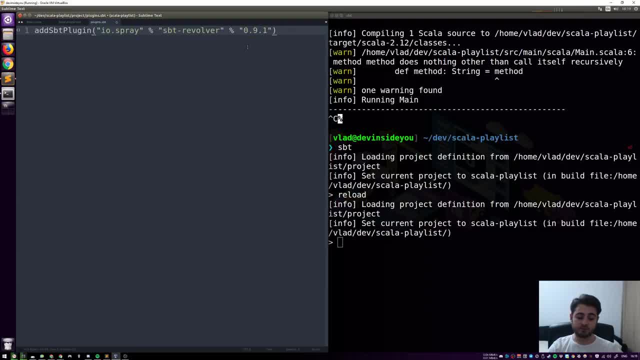 that it says: right so, uh, there's a way for um, for spt to find, uh, to find things online, and spt is just going to download it. now, you're not going to see that it's downloading it for me, right so? but if you say reload, it's going to notice that that now it actually needs this plugin. 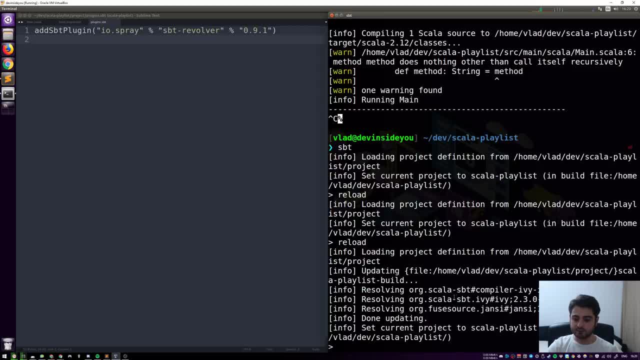 uh, you're not going to see that. it uh, you see that it's try, it tries to find it right, it tries to resolve it somewhere. um, no, you actually don't see it. so the thing is that i already have it, so i already have it, so my spt already downloaded, uh, while i was preparing for this video. so, uh, anyway, 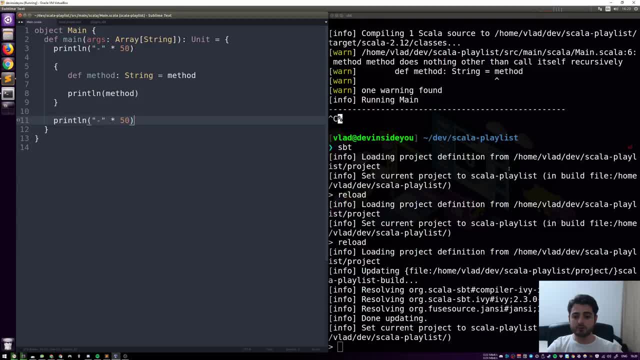 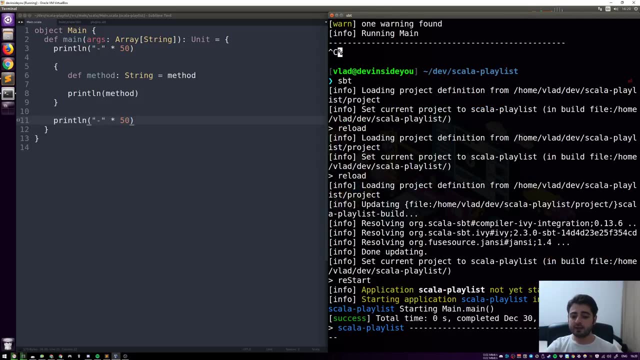 uh, let's go back to our uh, to our file. so, um, what, what spt revolver is doing? it's giving us a few more commands instead of- instead of saying run right, or instead of saying tilde, run, it's going. uh, it's giving us the command called restart. then restart is basically like: run right, uh, but if your application 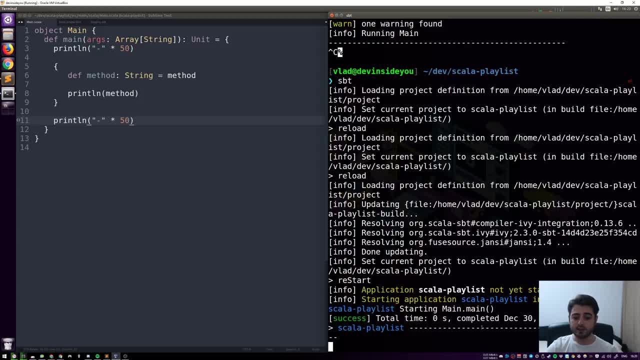 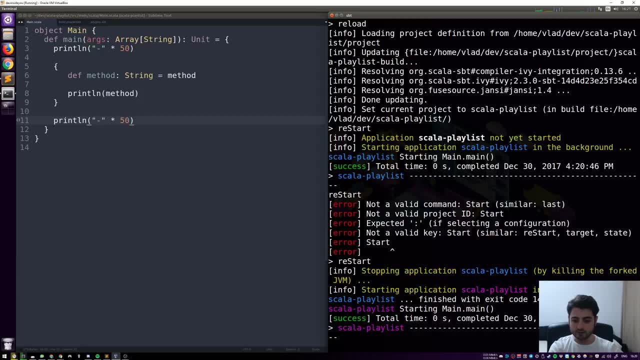 is already running and uh, and it's stuck in an endless loop. for example, right, you can just type it again. you can just say, um, re, restart. right, hold up, restart. there we go. and now what it did is so you? in the beginning it just said, okay, application scholar playlist not yet started. and now it 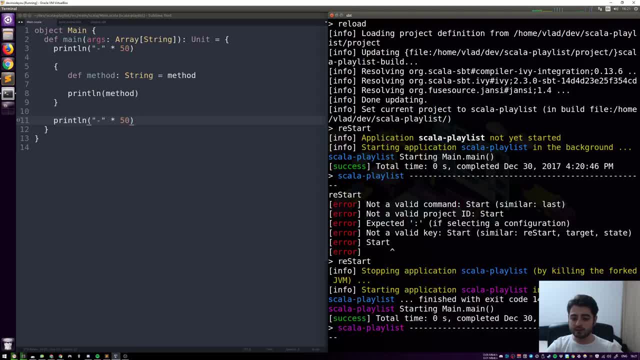 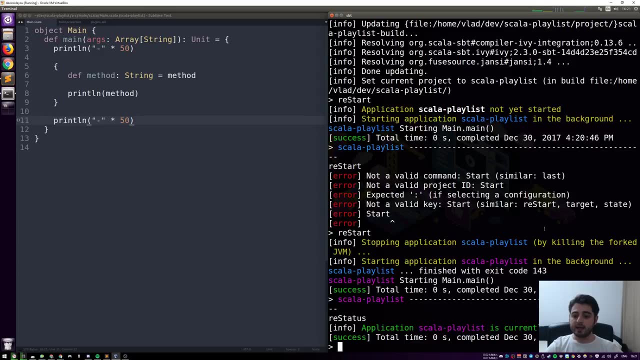 started the application in the background and now, the second time we typed in restart, it stopped the application and then started it again. okay, and we can also always see uh the status right, so it says it's it's currently running. as you can see, uh, based on my cpu, it's always running right and we. 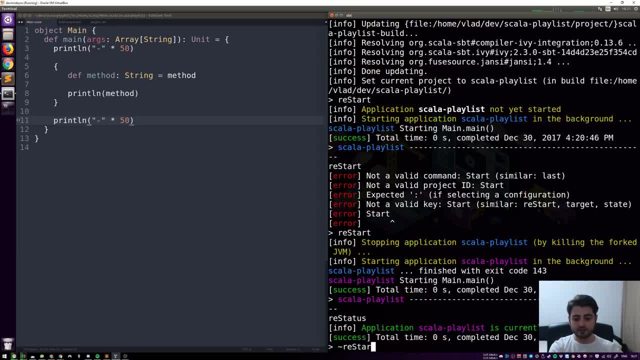 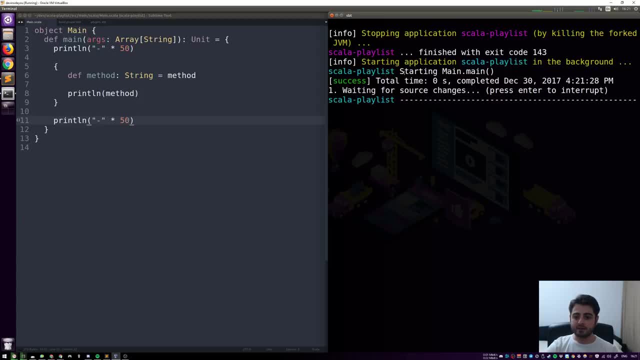 can also do uh, tilde restart, and we're gonna have a similar behavior as we, as we had, as we had before was rerun now, um, i don't like the fact that it uses like so many colors because, uh, what it's designed for is to to have uh, multiple applications running at the same time and talking to each other. it was designed. 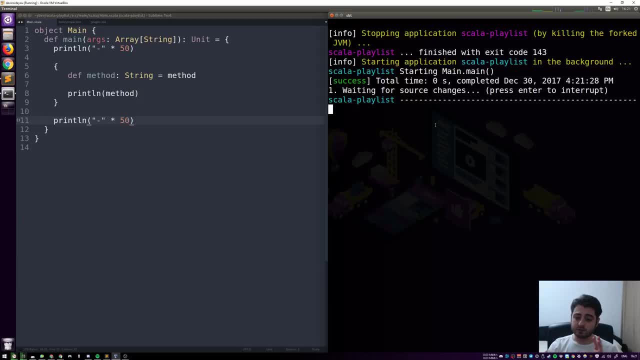 for a project called spray uh, which is an http uh client and server api, uh. so, uh, it was probably used for tests and for very hot, very, very fast, uh, very fast development. so, uh, what we're gonna do is we're not gonna have that, so we don't need all of these colors. so, if we go to our um, to our build file, uh, 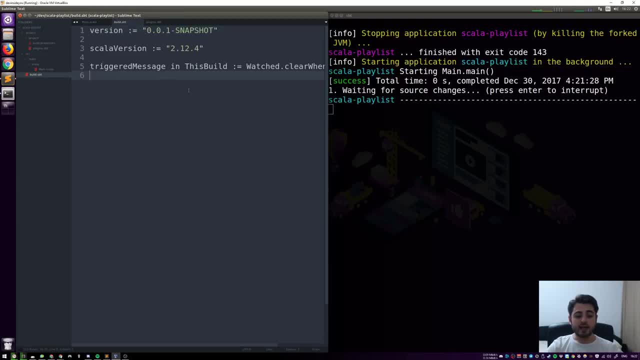 not the pluginsspt- to actually our buildspt. and if we add a line, uh, like this, let me just copy it over: our e-colors, um, colon equals revolve with no colors. i'm sorry, i just copied something wrong. so this is: this is all we need, right? so if we just do restop here, right, and we just reload spt, then 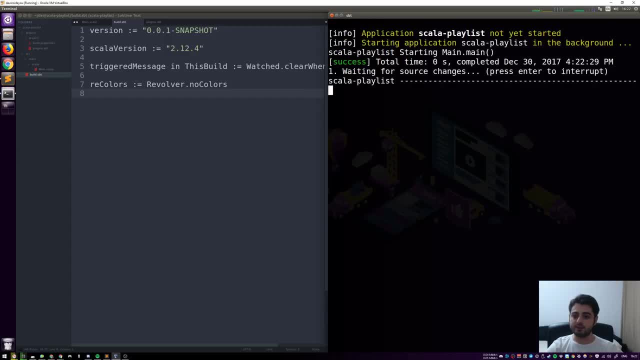 the next time we're going to restart, it's just going to use less colors. so we're still going to use the yellow color over here, right? so we're just going to use the yellow color over here, right? but every time we save and it's just going to restart it, everything else is going to be white. 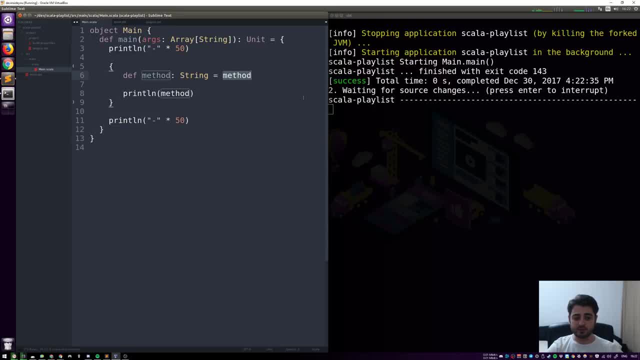 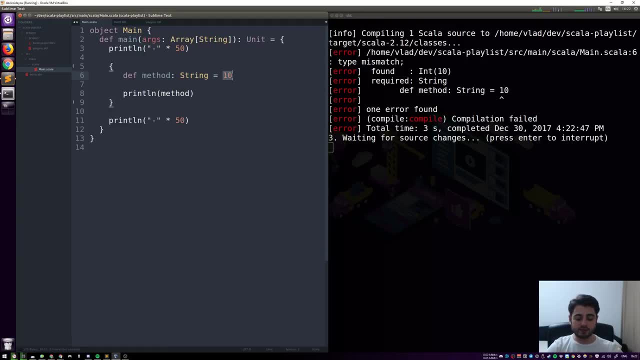 okay, so, um, the other cool thing is that we can also just say 10 here, right, and it's just going to kill it and it's going to run it, and uh, because now there's no, uh, there's no endless loop. i'm sorry, it needs a string. whoops, how did i do that? need the string 10, right, so now i'm just gonna. 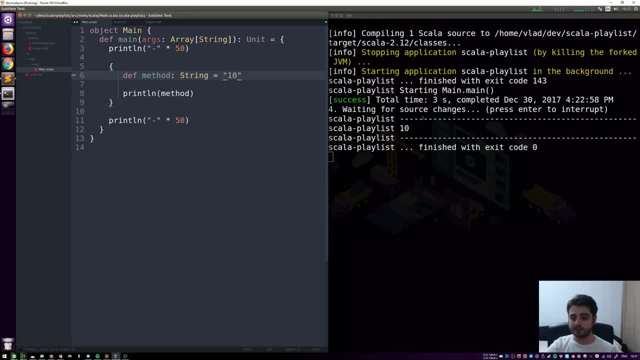 rerun. uh, and everything's gonna be fine and it's gonna look like this: so a bunch of hyphens, 10 happens and it finished with exit code zero, right, um? so the next thing that we're going to do is we're going to have a bit less hyphens. 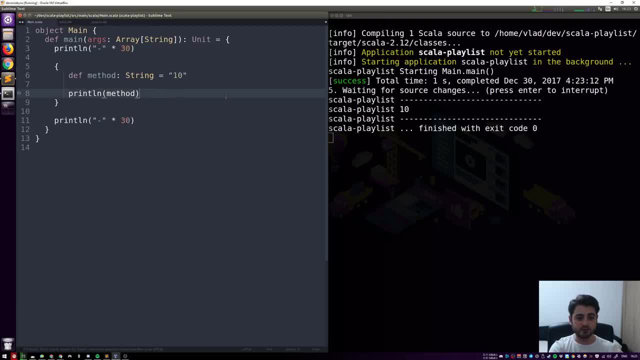 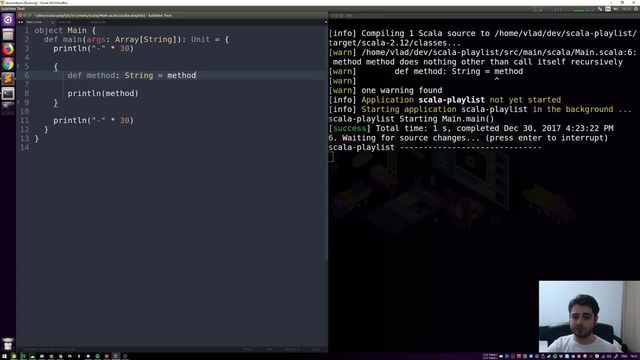 right, so let's have 30 happens, right, and also we don't. we don't really need that, okay, right so? so this is what we want to have, and let's go back to recursion. let's let's call this method again, right? so the next thing that that we're going to have is, um, the compiler tries to help, to help us out, right. 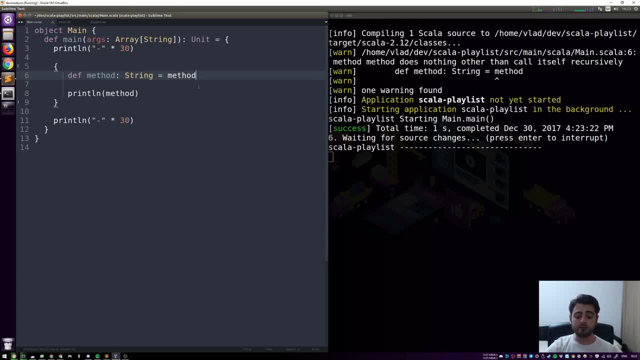 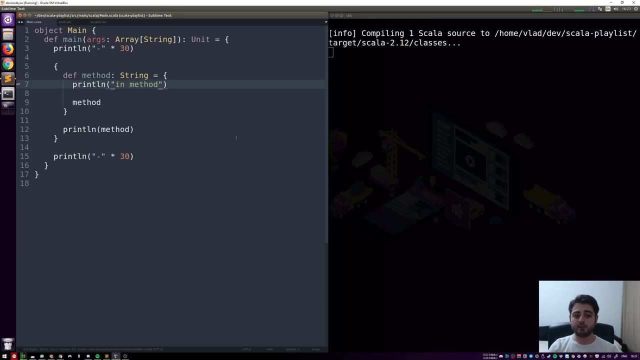 it says method, method does nothing other than call it recursive. we've already seen that before. so, uh, let's do this. um, why is it? why is it indented like that? that's what i want to have, okay, so we also want to have a print line and method. okay, so now what we should see if we should see this print line all the time. 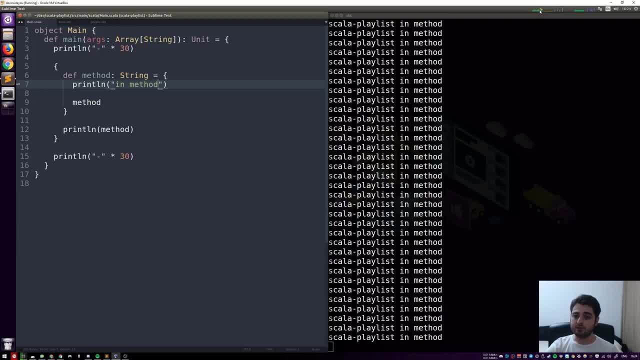 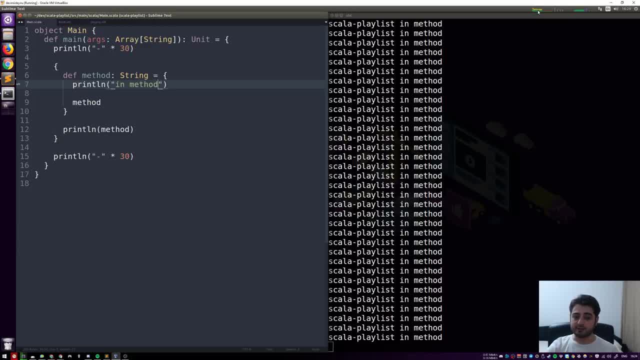 all the time, okay, so, uh, this is also why it, it, it um requires that much cpu. so i don't want to have that right, but i also don't want to have a warning. so what i'm going to do is i'm just going to have a vowel over here. wow, leave me alone. equals true. 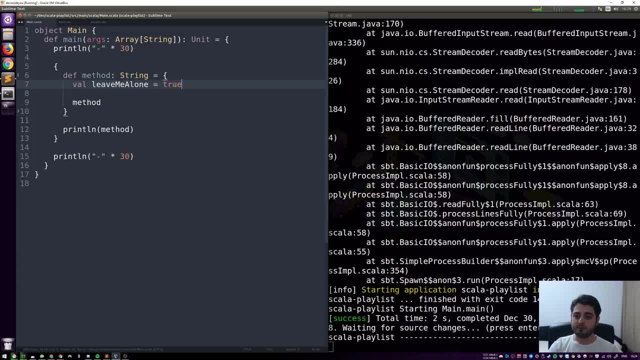 okay, so now i don't see the seal, the print line. okay, my cpu is sort of a little bit more down, okay, and um, yeah, and the application is running over here. um, let me save that. so you see, you see this nasty output because it has to kill the application, and, um, in a weird way. okay, 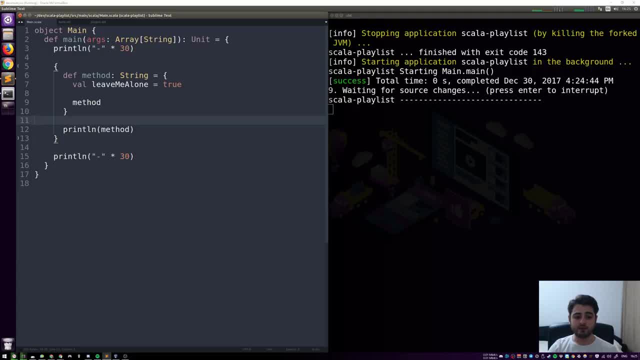 uh, and you can see the cpu is running over here. so just a few notes about uh spt revolver before we, before we continue. so it's called like this because it's designed for very fast development. you know fast as a revolver and uh, what it's doing is um it, it forks a, a jvm uh in the inside of. 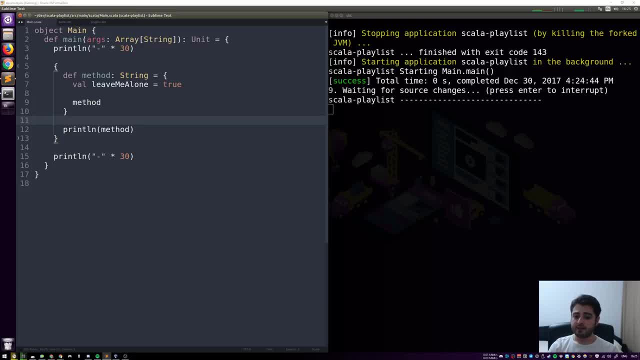 inside of spt. so, uh, what it's doing is it creates like a separate process and it monitors it. so there are a bunch of things uh running and uh, every time we, we make a change, it just it just kills the other, the other jvm, and creates a new one. so, uh, we don't, we don't have to control cp. 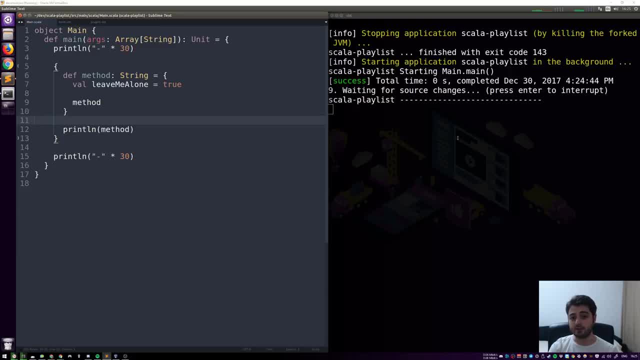 and then kill the whole spt. so this is, this is how it works, right, so it forks the. the term is forking, right, so it forks a jvm. all right, so we obviously don't want to have an infinite loop, right? so, uh, what's causing the infinite loop? well, we always call method, right? so what we want to have is that. 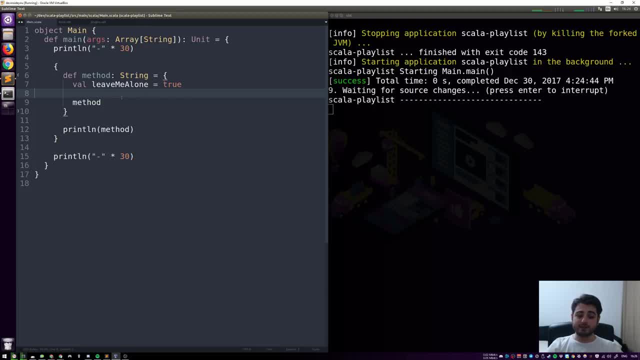 sometimes, uh, we don't want to call method and sometimes we just, we just want to be done right, so we want to have something like: um, if something, uh, then call the method, um, otherwise just to say done right. and so what's happening right now is something like this: right, so it's true, it just it. 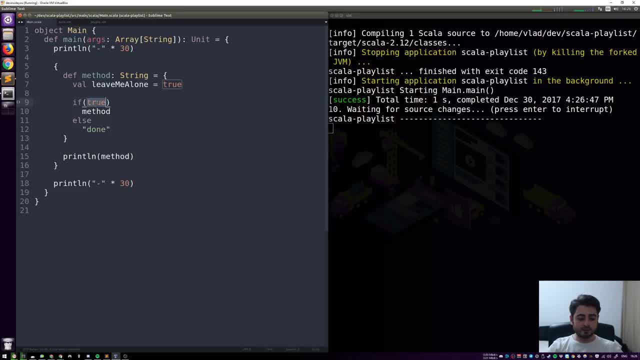 just keeps calling itself right, uh, but sometimes we want it to be false right and we want to stop calling itself right. we just want to. we just want to return that as as over here. so, um, how we're going to do this? well, we need some sort of external force. in my example, we're just going to 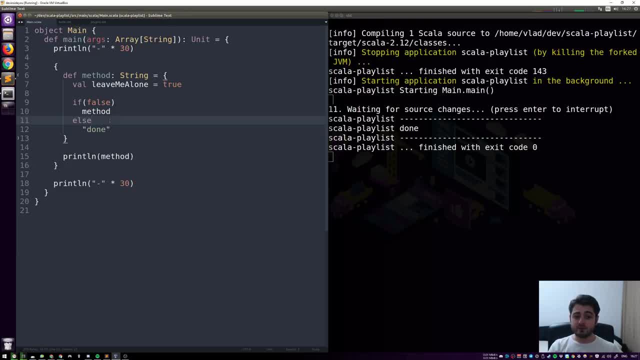 use. we're just going to use the current time, right? so, uh, when a few seconds are going to pass, just just just stop calling itself okay. so, uh, skylar is fully compatible with java and uh, the way you the current time in java, uh, since recently uh is, is like this. so we're just gonna say: get current. 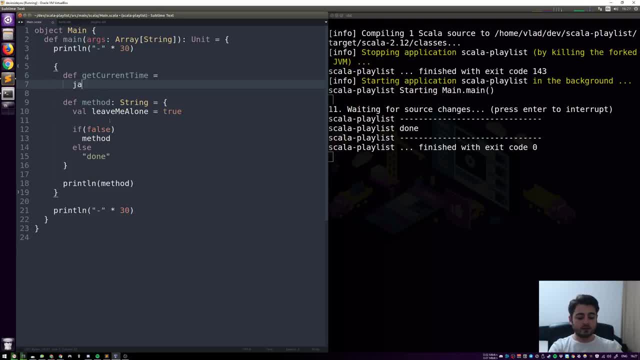 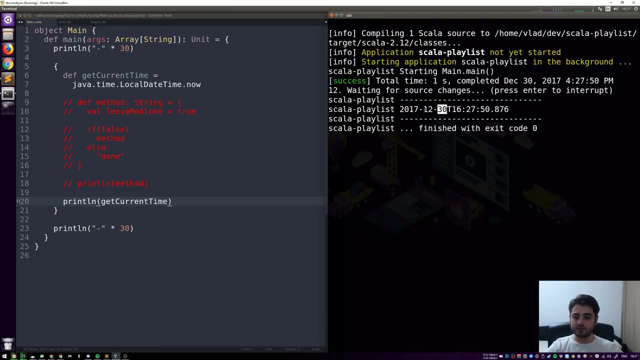 time equals java time, local date time. dot now and in fact, before we continue, let's just, let's just play with this a little bit. um, let's just not do that, okay. uh, let's just print out: get current time. let's see, all right, so this is the current time. so it's a third use of the. 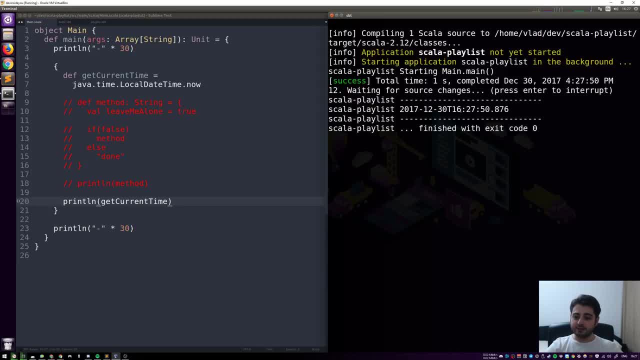 second and the day of right. so as an example, let's say it's uh, 9, all the socialness, second through, okay, the second one total is seven days now and it should go up. we'll give it a little bit more of that. so here's our correction call, as us keep it apart a little bit, but, um, we're. 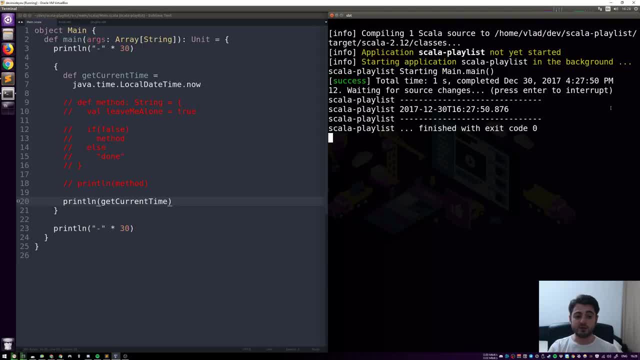 just gonna keep Roman's an octopus, so we'll give just this that, and it should do what this always does, remember, it's a little bit more time than is the record time, so what we want is just to call it under a single moment. okay, and now all you have to do is just sort of run until g and then. 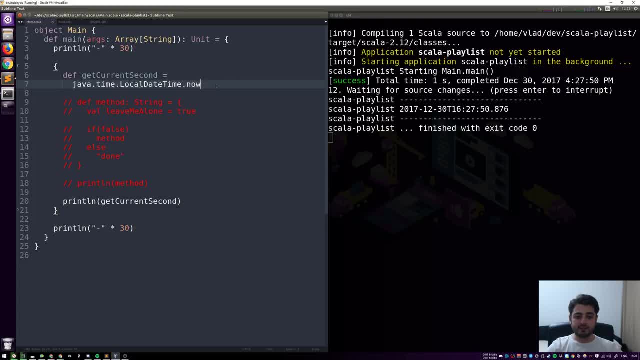 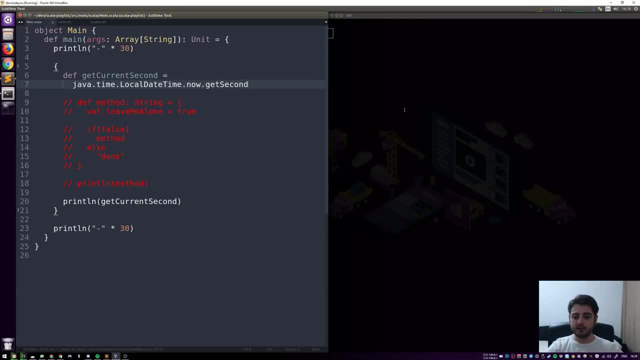 this will do an authorizedолет Building method. yes, tomorrow is a new year's, he is, tomorrow is a, And over here we're just going to say getSecond And let's print it out. So we just see 39, and I'm going to run it again. 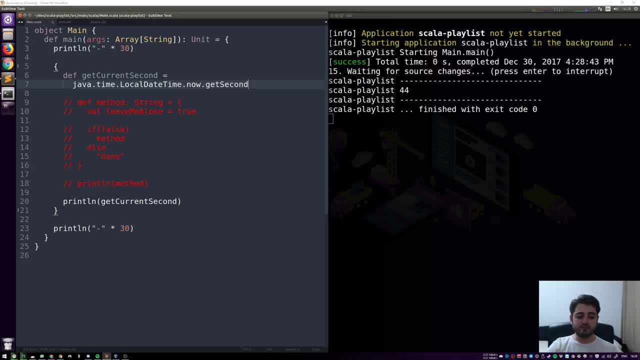 We see 42,. I'm going to run it again. We see 44.. A bit later in the video we're going to talk about threads And remember I mentioned that thing. I don't remember in which video. actually. 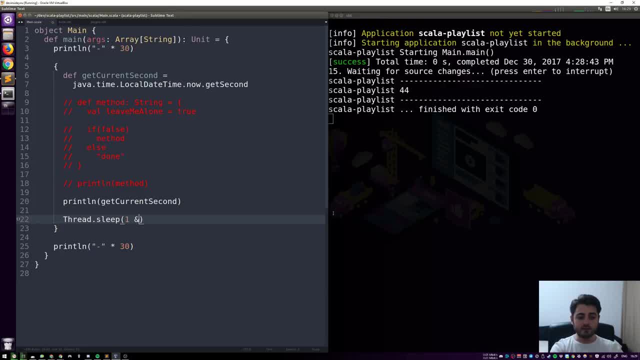 But you can sort of pause the current thread for a while, and for how long you give it in milliseconds. So if you're going to stop it for a second and just kind of print it out again, right, I'm just going to stop it for a second again. 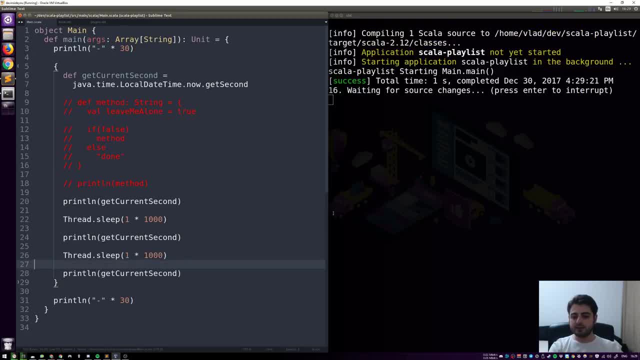 I'm just going to print it out again. right? Then we should see a print line every second. right, We see 21,, 22,, 23.. Now, if we didn't have that right, CPU is much faster than doing one instruction per second, right. 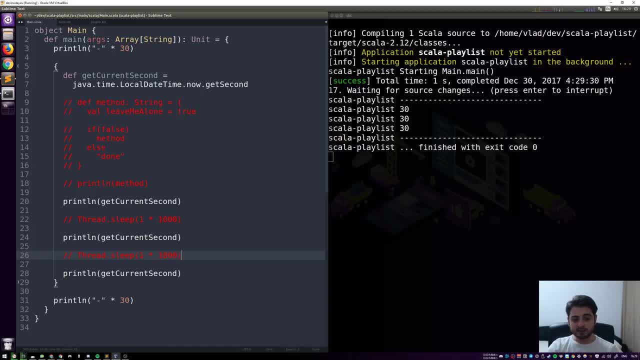 So it does millions and millions of instructions per second right. So we see the same second printed out a few times, even though it's a def right, Even though we're getting it all the time, it's a new value, okay. 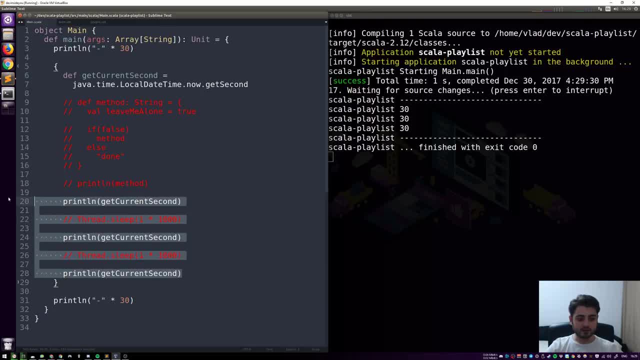 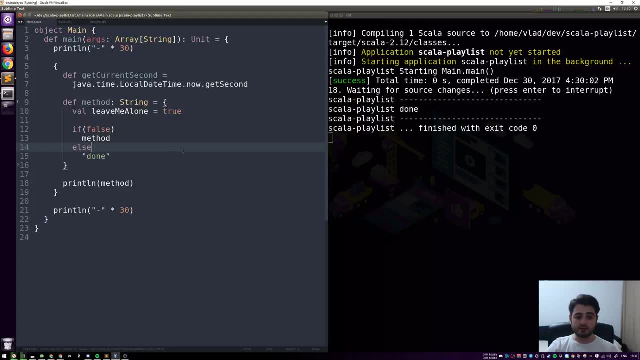 Let's revert all that. So we don't need this whole getCurrentSecond, We just need our example. okay, This thing, okay. So we're back to the endless loop, but we're not, because we're not using getCurrentSecond thing. okay. 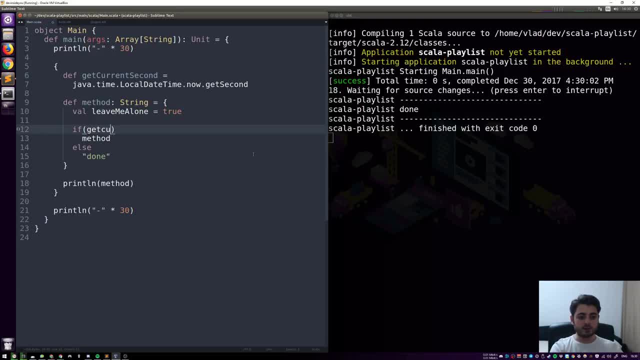 So let's actually use it. So the way we use it is in the if expression we're going to say if the rest division by five, right. So this symbol, this percentage symbol, is a common operator used in programming for the module operation. 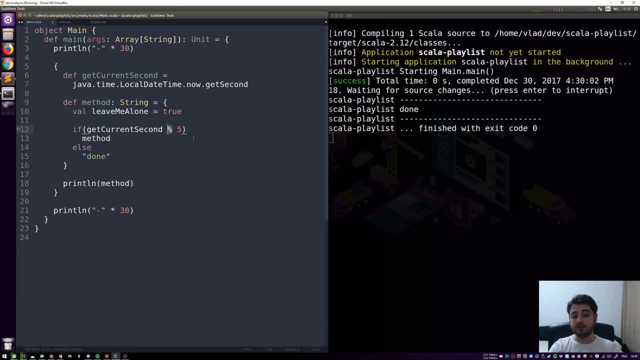 And module operation is the division, so it's a function of that rest, so it gives you the rest, right. So if this is not equal to zero, then it means then we're somewhere between zero and five, right? Somewhere between five and 10,, somewhere between 10 and 15, right? 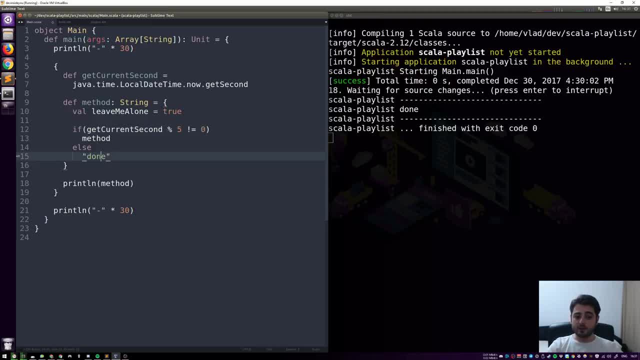 So if we're there, then just keep calling the method. Otherwise, just say that we're done and let's see what's going to happen, right? So first of all, we don't really need this thing anymore, because more things are already happening, right? 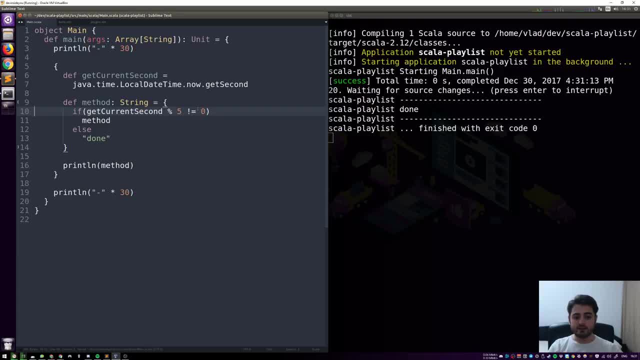 So we're seeing it's waiting, waiting, waiting, waiting and then done. right, And now again waiting, waiting, waiting, waiting and now done. So let's actually have a println. Let's have a println over here. 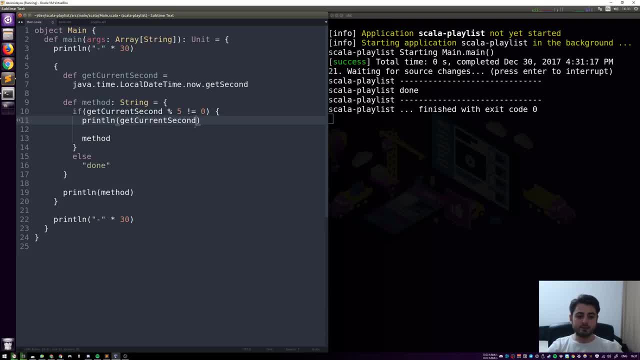 Let's have a println getCurrentSecond. And because it's a DAF right, even though it's really really fast, I actually want to have it in a vowel. So let's freeze the current second right. Let's have: vowelCurrentSecond equals getCurrentSecond. 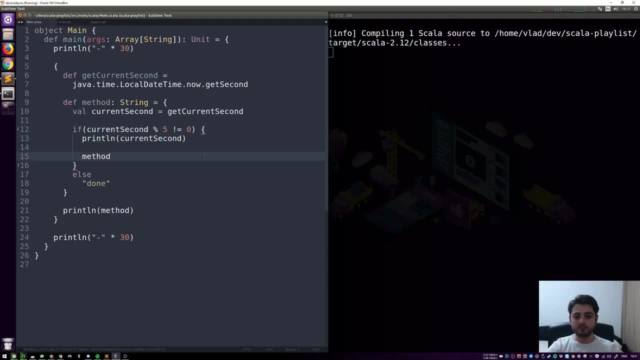 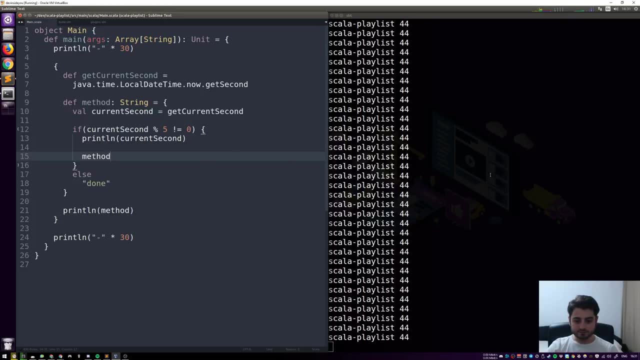 and let's just use that one instead, right? So what we're going to see now is we have the same second printed out quite a few times, right? And then it should stop. There we go, there we go. So we had 43, we've seen it like a bunch of times. 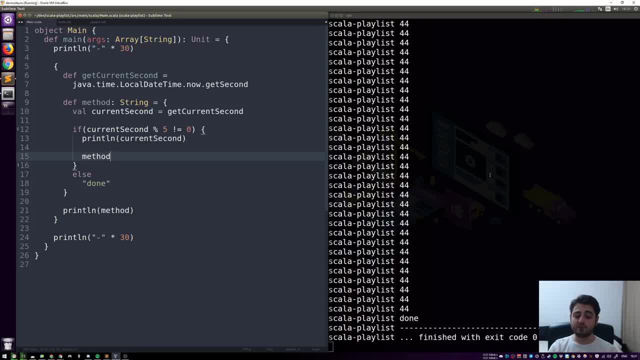 and then we've seen 44 a bunch of times and now when it came to 45, it stopped. okay, It's done. Now, this is an example that I chose just for educational purposes. Usually, when you use recursion, you don't want to just do randomly stop, you know. 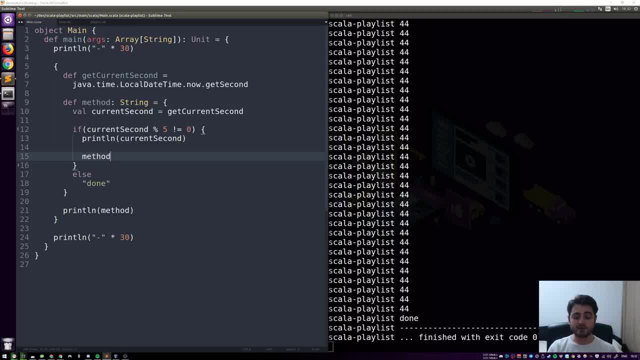 You want to have a full control of stopping. So what we're going to have is we're going to manage this state ourselves, right? So somewhere somewhere over here, right, Even though it's deaf, somewhere over there there is a var. 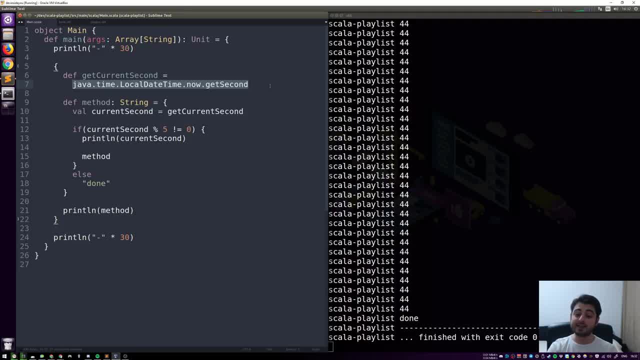 that keeps track of the current second. In fact it's happening on a different thread. You know we paused the current thread like a few seconds ago and on a different thread things were happening. We're going to talk about threads a bit later in the video. 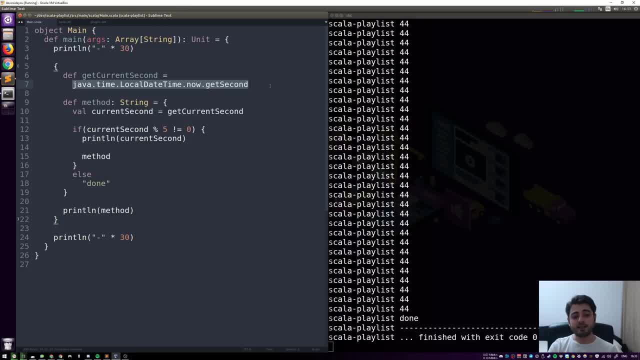 so don't worry if you don't understand what I just said, right? But basically something else was taking care of managing this state for us, right? So in our example, in the next example, we're going to do it ourselves. 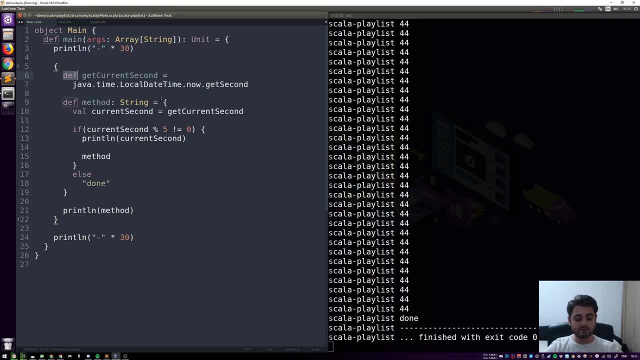 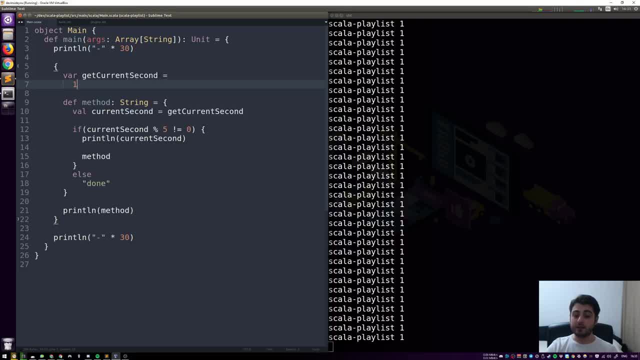 Because we forgot to actually manage this state, because you know nothing on a different thread is changing this var, So we're going to have to change this var And the way we change the var is by doing this: Get current second plus 1.. 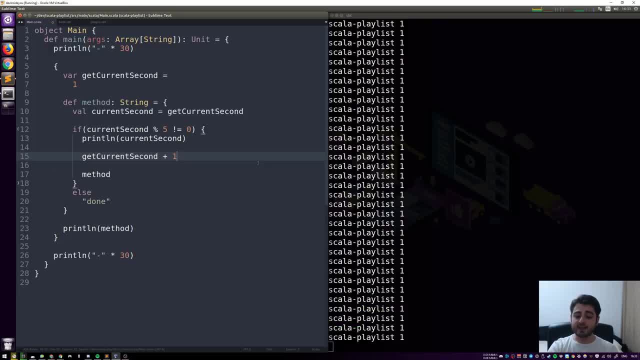 And this is a common mistake that beginners are doing- because in fact it didn't change anything. because, well, we added 1 to the get current second, but we didn't change the var right, So we also need to change the var. 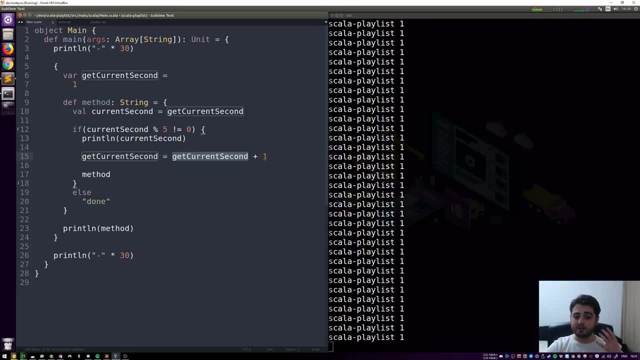 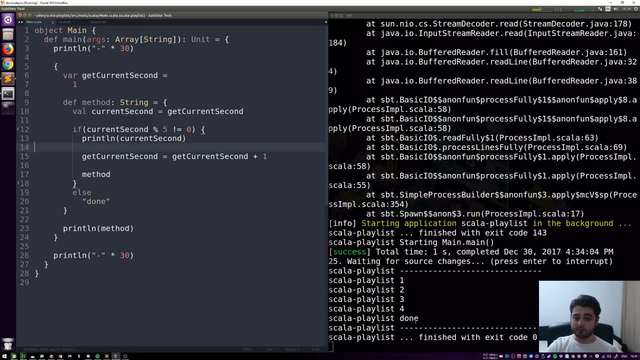 We need to do: get current second equals whatever the value of get current second currently is plus 1,. okay, So now it should actually do 1,, 2,, 3,, 4, and then printout done. Also, note that there is a shorter syntax for this. 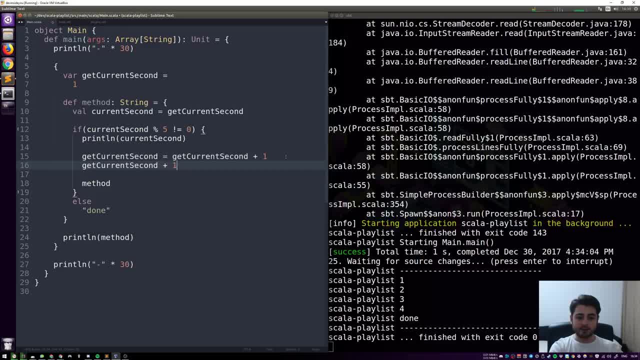 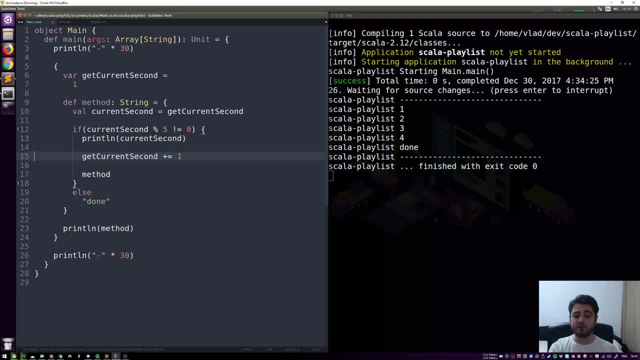 So, instead of saying that and having a mistake like that, we can just add an equals sign over here, and it's going to do exactly the same thing as over here, right? So this is what we're actually going to have. So this is a very common syntax. 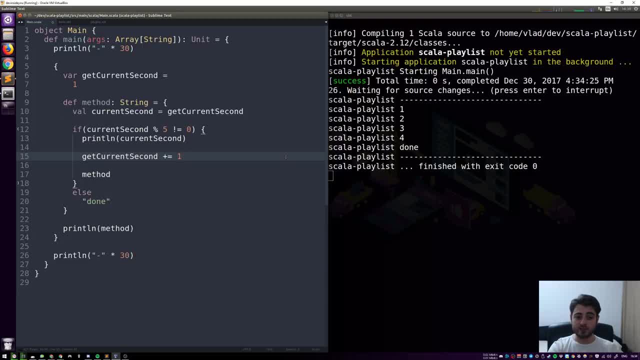 And, in fact, some languages like C++- and this is where the name comes from- is they do this plus, plus, And this is where the name C++ is coming right. Okay, but in Scala this is not possible, by the way, right? 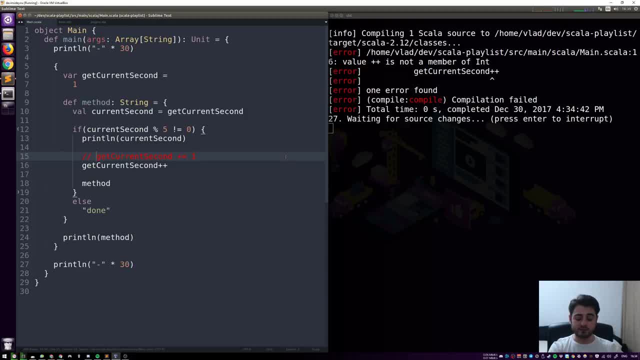 So this is not going to compile. Let's see this. Yeah, so it's not a member of an integer. okay, So let's have that. Everything is working again. So if we start with 1, then it's going to be done, right. 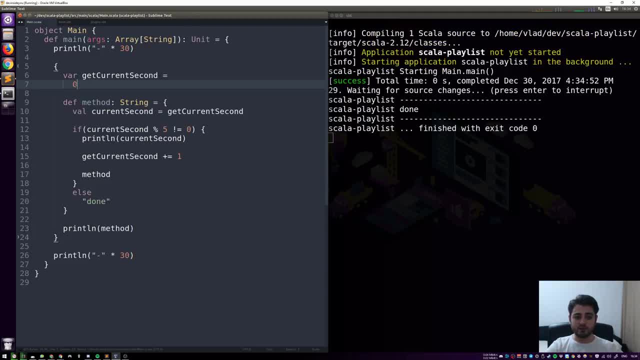 But if you're going to give it a 0, then it's just going to go straight to done. If you're going to give it a 5, it's going to go straight to done. If you're going to give it a 10, it's going to go straight to done, right. 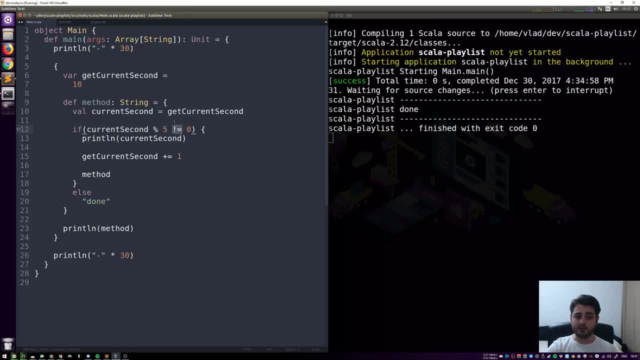 Because of this thing, We're going to talk, by the way, about this and about that in the next video. I believe it's the next video, yeah, So let's go back to 1 and go back to our regular example. all right, 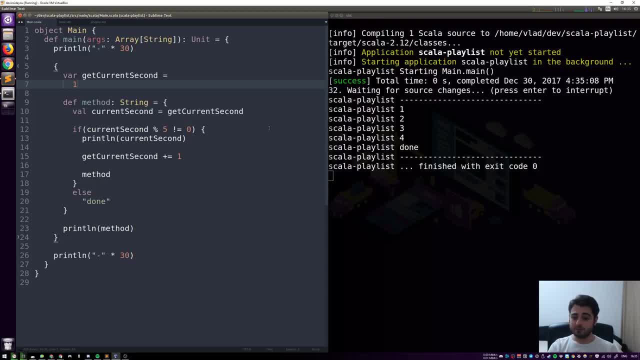 You got a lab revolver. I got to say SPT revolver is awesome. You know endless loops and whatnot. It just freaking works. It doesn't die. It's cool, All right. so let's look at what we have here. 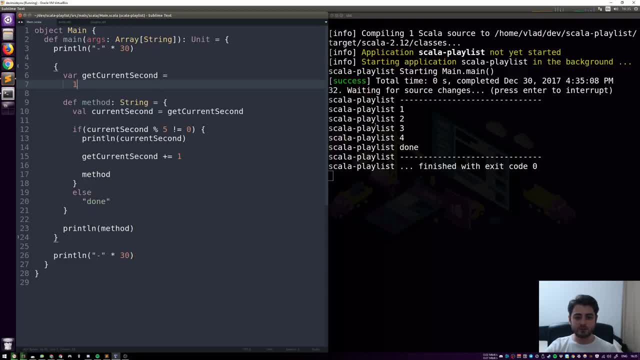 So, first of all, we don't have seconds anymore, right? So in fact, what we're doing is we're sort of counting the iterations right, Like how many times did we call ourselves right? So let's rename this into get current iteration right. 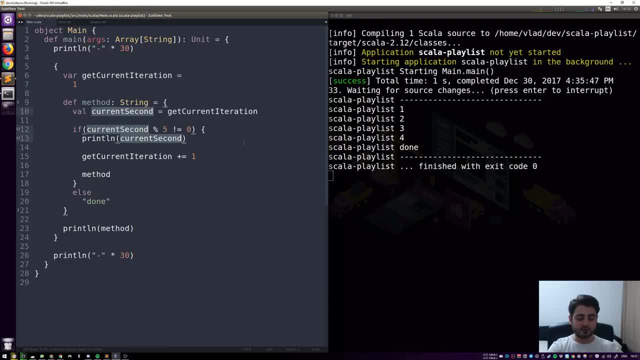 Same thing, And now that thing is not called current second, It's called current iteration, right, And also notice that because we have full control of this var right, So it's not a def anymore And some other thread changes it behind our backs. 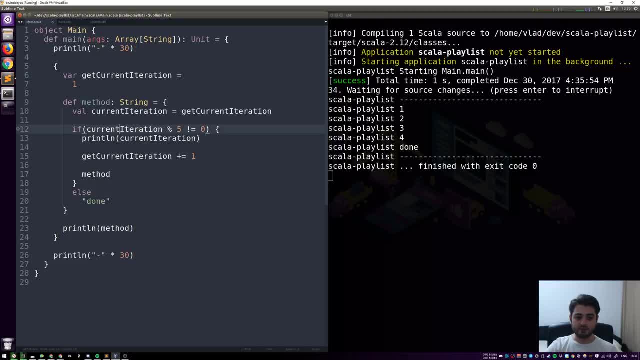 It's a var, so we have full control of it. So there's no need to get it, because we're using it twice, right? So there's sort of no need to freeze it, right? So what we're going to do is this is actually not get current iteration. 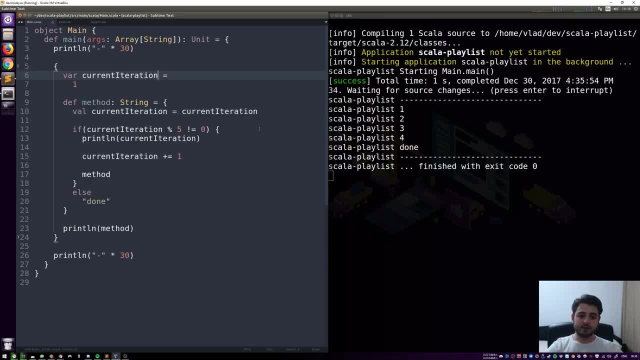 This is actually current iteration. And now over here we're saying, okay, current iteration is current iteration, So we just don't really need it, So we're just going to remove it, all right. So this is what we have. 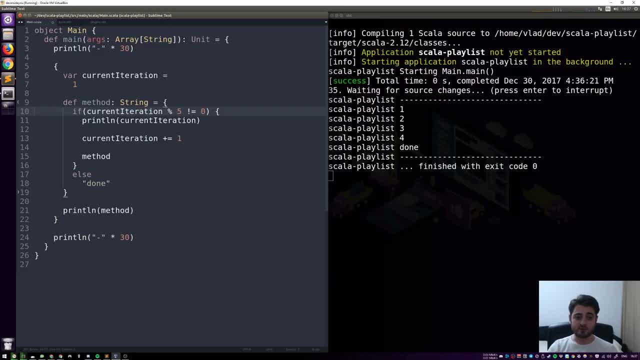 The next thing that I want to do is I want to have different versions of the same algorithm, right? So I want to have different code that is doing exactly the same thing- This is also called refactoring, by the way- So I want to have method two and show you a different implementation of this. 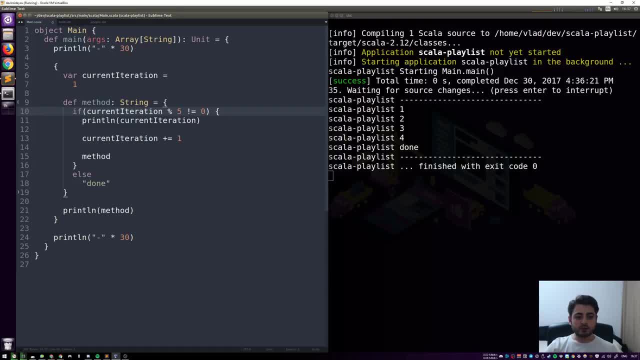 But before we do that, we should keep this var as close as possible. all right? So vars and managing state is as complicated as it is, So let's keep a close eye on it. right, So let's keep it closer. However- and, by the way, let me align that okay. 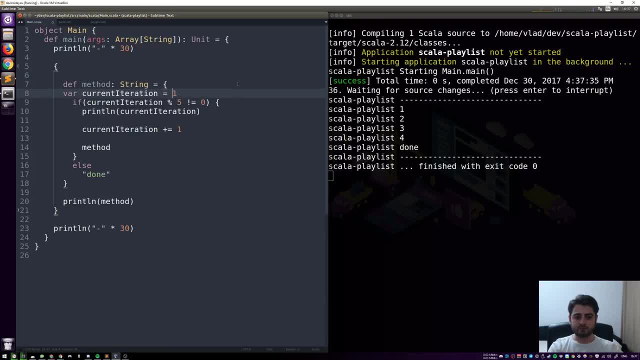 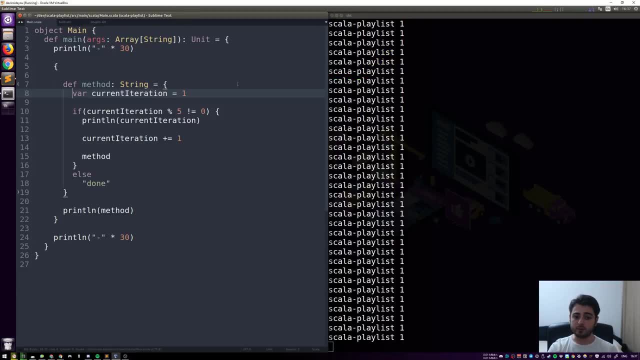 However, we can't just put it in over here, right So? because this basically ruins everything, right? So we're going to have a deeper discussion a bit later in the video about what exactly is happening behind the scenes, But we can't have it over there. 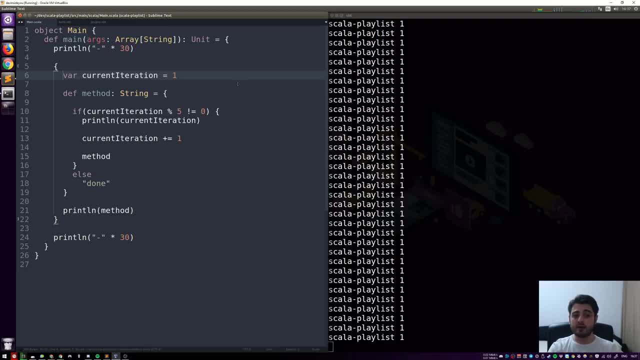 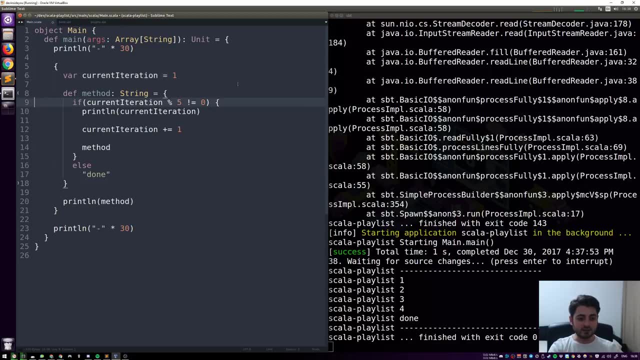 So what are we going to do then? How are we going to solve this problem? Well, when in doubt, just have another scope around, okay? So, first of all, I see an empty line here that I need, okay. So what we're going to do is the first thing that we're going to do is, instead of having a method here, right? 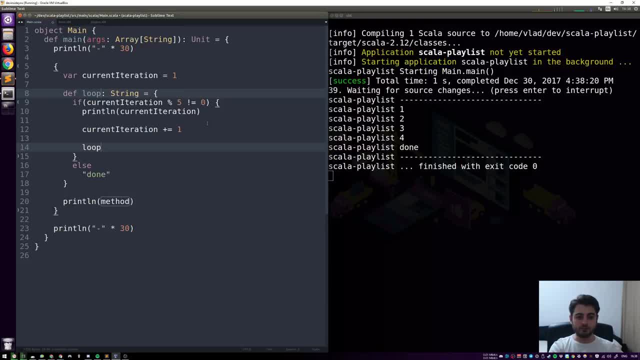 We're going to call it loop. We're just going to call it loop, okay. And what we're going to do now is we're going to leave the print line alone, but we're going to take all of this right And we're just going to surround it with another scope, okay. 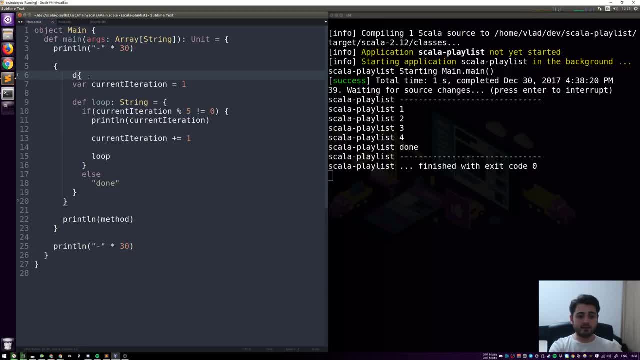 So it's going to be close here And what we're going to have here is def method, right, as we had before. So we just have a scope around and it's going to be like this, right? So now everything looks the same, sort of right. 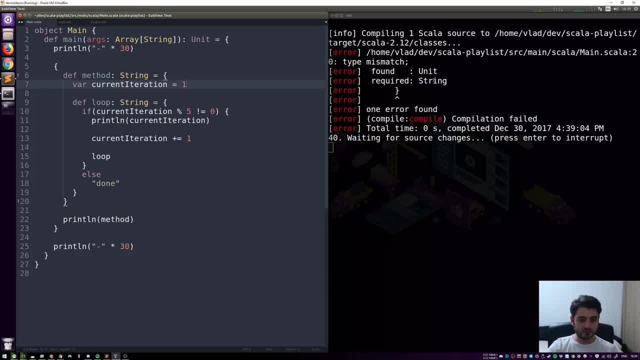 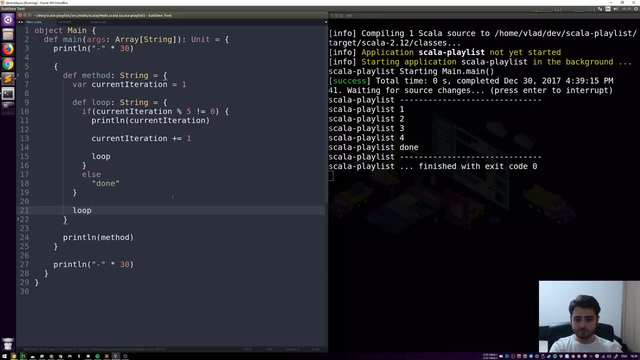 What did I forget? Found unit Required structure String. Oh yeah, We have to also call loop over here. There we go right. So now we have the same thing. So if it's 0, it's going to be just done. 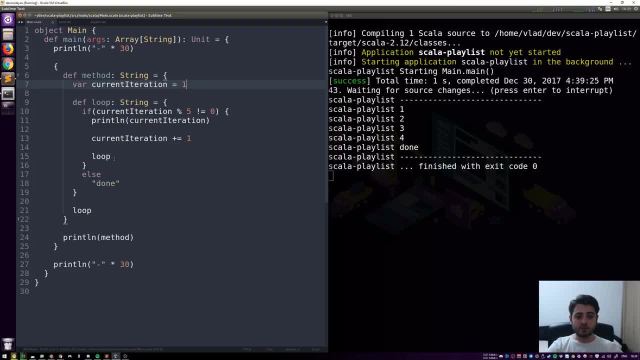 And if it's going to be 1, then it's going to do the same thing. So all we did was we renamed method to loop and we just had another scope around it, And now this scope is a method right, So we're still calling method. 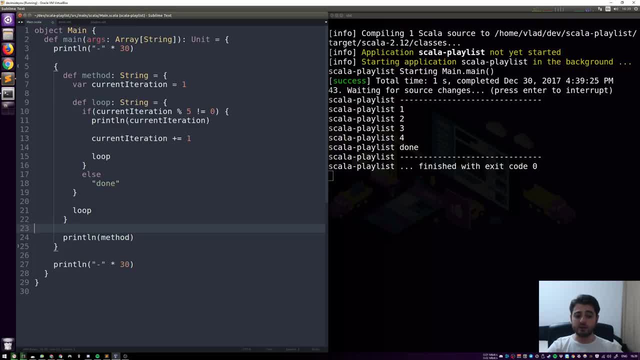 And, by the way, notice that now method is not calling itself, Loop is calling itself. okay, And because of that we don't need the return type. Now, I'm going to leave the return type there, right? But just so you know, right, you don't need the type. 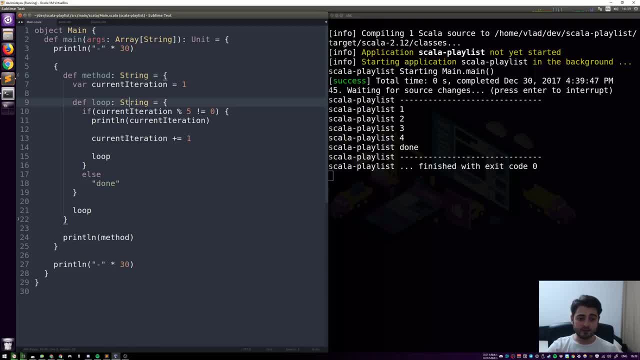 So now Scala is capable of reconstructing the type. However, over here it's not right, because this is still a recursive method. okay, All right, so now we can have the next implementation of method. okay, So what we're going to have here is- I'm just going to copy that: 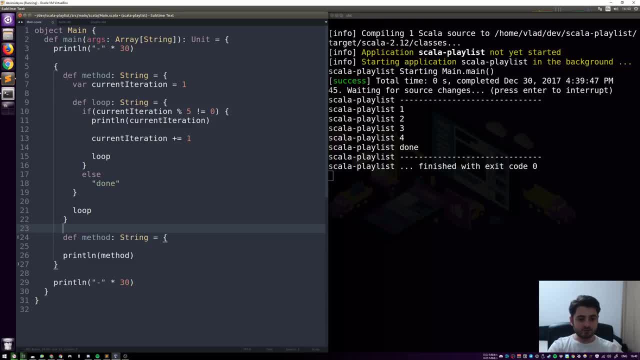 In fact, I'm not going to copy that, I'm just going to duplicate it and bring it down over here, right? So what we want to have is we want to have method 2, right, That somehow produces a string, right? 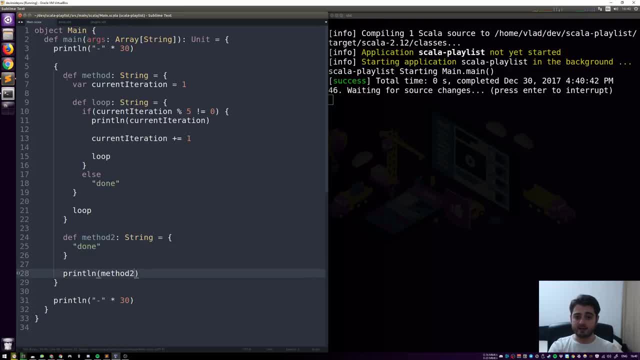 And we're just going to call method 2, okay, This is what we want to have right And how we're going to do it. is you learned in the previous episode about subroutines right? About a different way of binding, right? 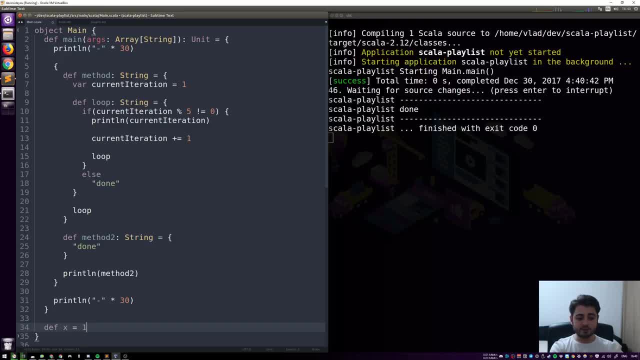 So before we knew just that x equals 10 and we know that the value of 10 is bound to x, And now we also learned that we can also have a parameter right, a parameter of a subroutine, which is a different binding right. 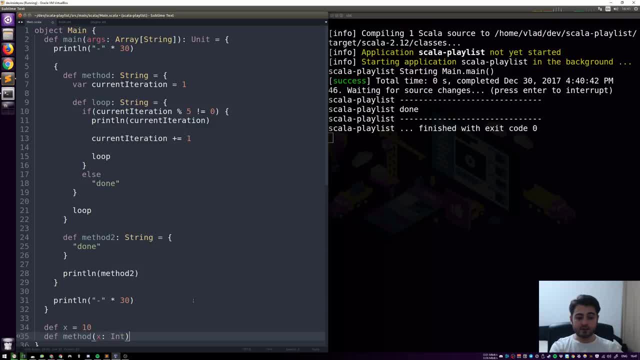 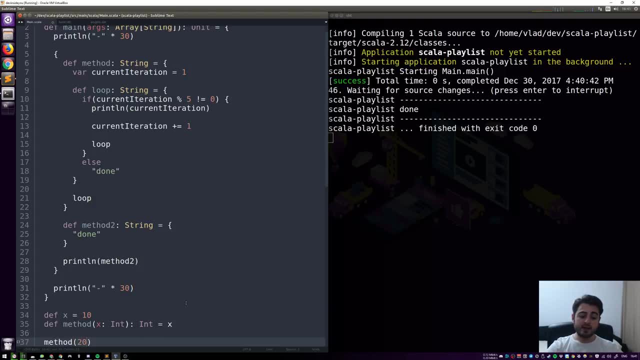 So we have the method and it takes an int, right? So whenever it doesn't matter what it's doing, right? So later, when we call method with- I don't know, with 20, then this 20 is also bound to that x, right? 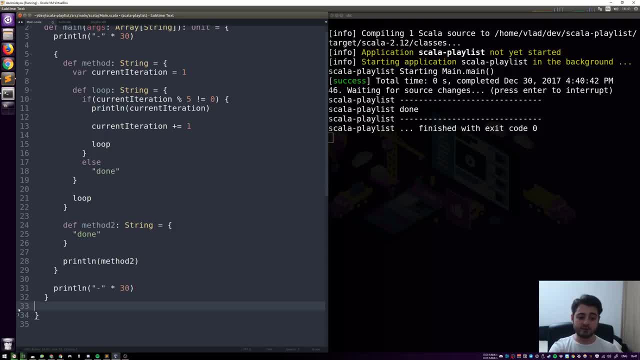 So this is a different way of binding, And this is exactly what we're going to do over here. So the method 2 is going to look very similar to method 1, right, In fact, maybe let's just call it method 1.. 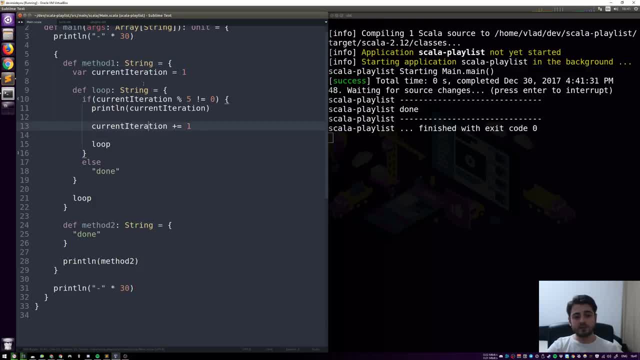 Yeah, we're going to have method 1 and we're going to have method 2.. So method 2 is going to be very, very similar, But instead of binding of this variable right Like this, we're just going to have a parameter for loop. 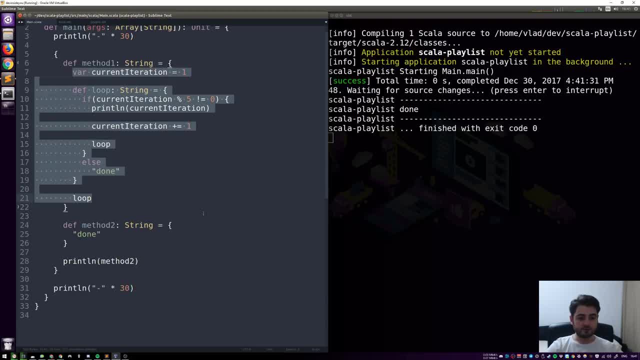 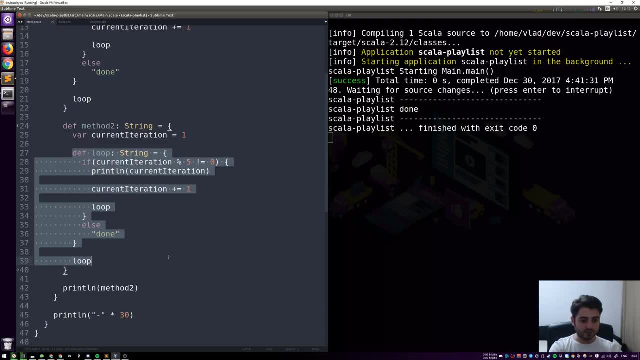 In fact, let me just copy everything from here, right, And put it over here, right. So now they look the same. I'm not sure why I sublimated that. There we go. So now they look the same. So method 2 and method 1, they're doing the same thing, okay. 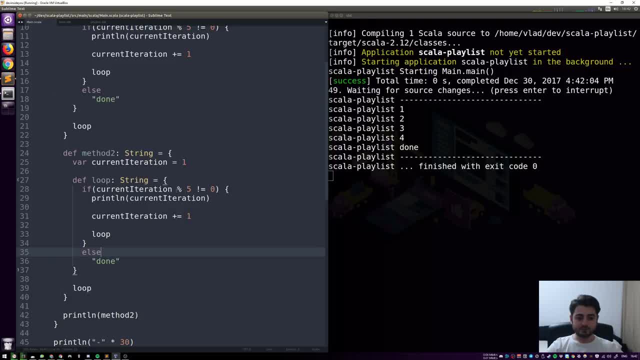 But the code also looks the same. So what we're going to do now is look at this. So, instead of having this, current iteration equals 1, we're going to call, we're going to put a 1 over here, right? 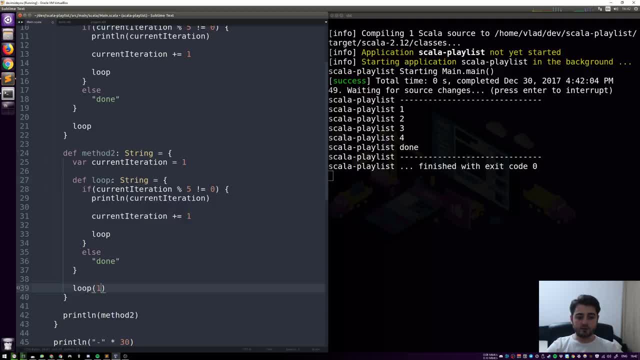 Into loop right And therefore loop is going to need this parameter right. So we're going to put a parameter list over here, right, We're going to put the current iteration over here And we're going to have to say that it's an integer right. 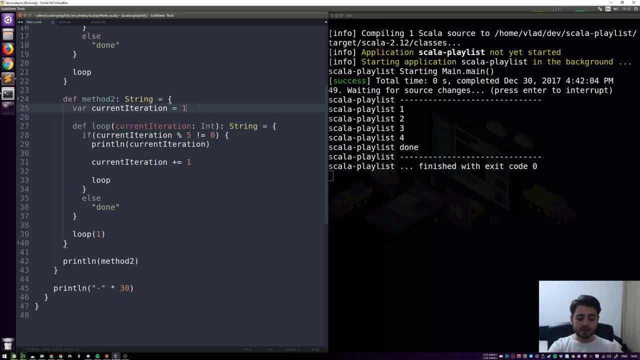 And we're not going to have this thing right. And because we don't have this thing, we can't increment this. By the way, the parameters that are going into subroutine: there they're vowels automatically, so we can't do that. 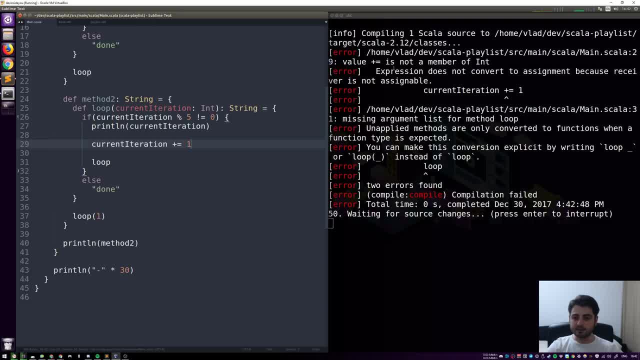 In fact, if we do that, maybe the compiler is going to tell us: yeah, it's going to say expression doesn't convert to assignment because the receiver is not assignable right. So it's a vowel right. But we actually don't need that. 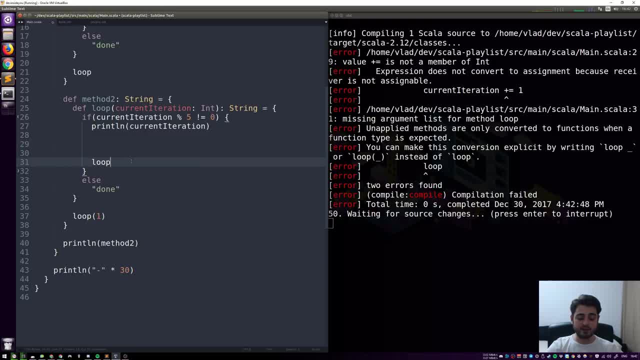 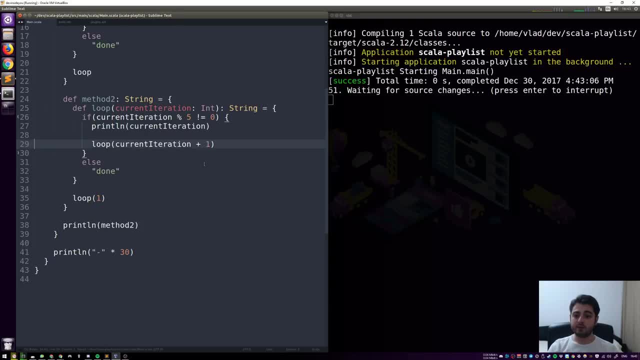 We actually don't need the whole thing, because this whole thing is going to go in as a parameter to loop without the equal sign, obviously right, And we're just going to have that. And there we go, the same thing: 1,, 2,, 3,, 4.. 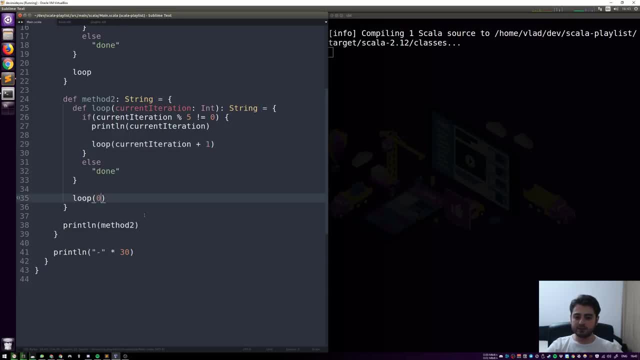 And if we start with a 0, it's going to be just done. We're just going to start with a 5.. It's going to be just done, And so let's revert it back to 1.. So now I'm going to scroll up so that you see both of them on the same screen, right? 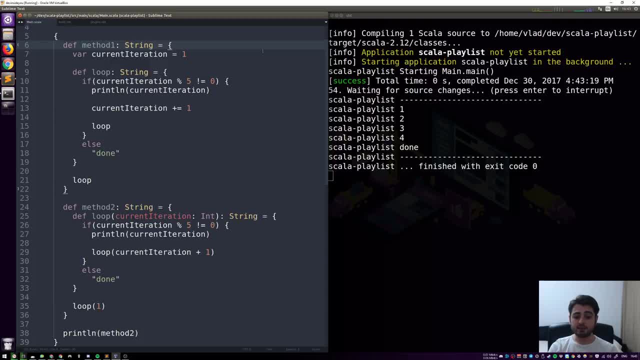 So that you can compare them And take a look at it right. Pause the video, take a look at it. Play with this on your local computer, because otherwise you're just going to forget it. okay, It's really important that you understand this whole thing. 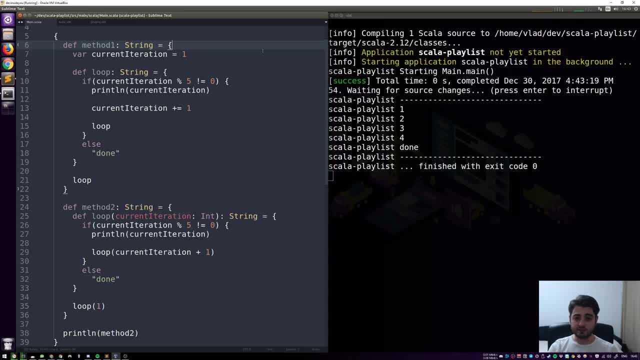 So take your time to understand it. Recursion is a very complicated topic. Beginners really really hate it. The next part of this video is what is actually happening behind the scene, And this is where this thread thing is coming in. So remember, just a few minutes ago we did this threadsleep thing. 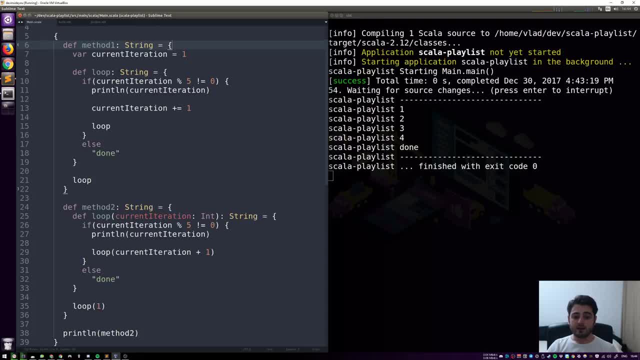 So what is happening is that when a program is running, you have a process, right, And if you have two programs running, then you have two processes right. But inside of a process, what is happening inside of every program? you have this thread, right. 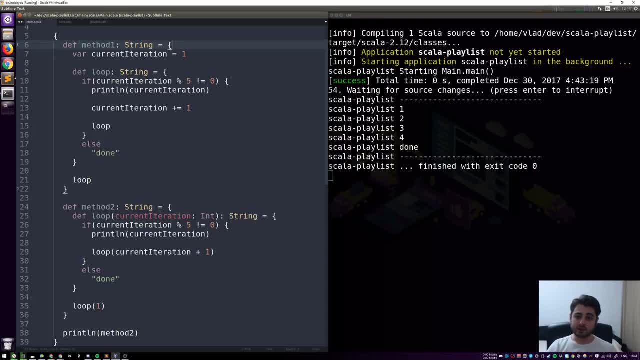 And this thread is just running subroutines, one at a time, right, And if you have multiple threads, then a program can do sort of multiple things at the same time. It sort of looks like it. In fact. let me go into Windows over here. 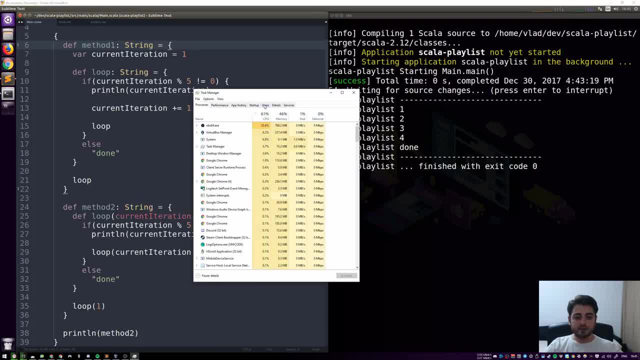 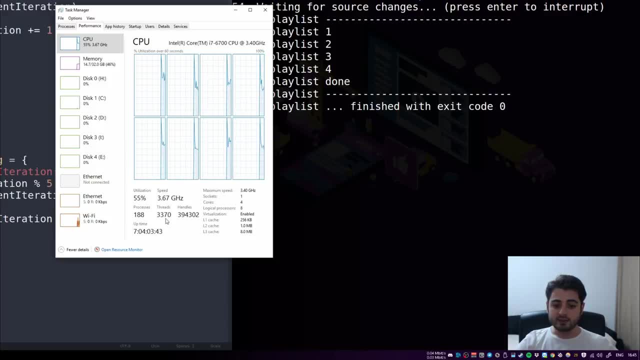 I'm just going to say Task Manager- right, And I'm going to go to, I believe, Performance right And over here we see okay, so I have 190 applications running 190 processes And this is how many threads I have right. 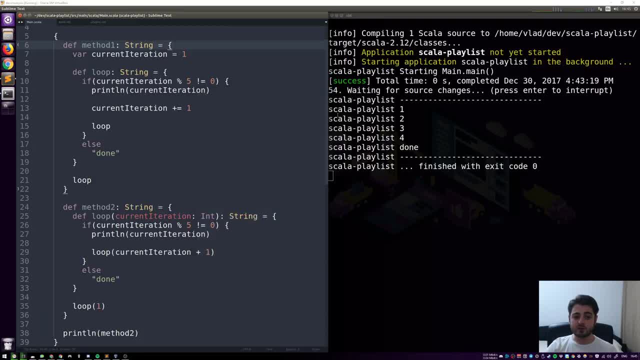 Anyway, this is just a bit of a side track. So in order to understand what a thread is in fact, we're not going to talk about threads too much, We're going to talk about what is inside of the thread. So inside of every thread, there is a thing called a stack. 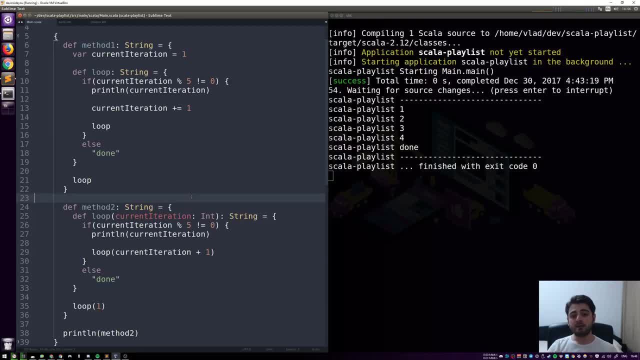 And all we need to understand for today is how a stack works. Now, a stack is just a synonym for a pile. So imagine if you have your table and on your table you have a pile of papers, right? So if you're looking for papers, you can just look like crazy and take one from the middle, right? 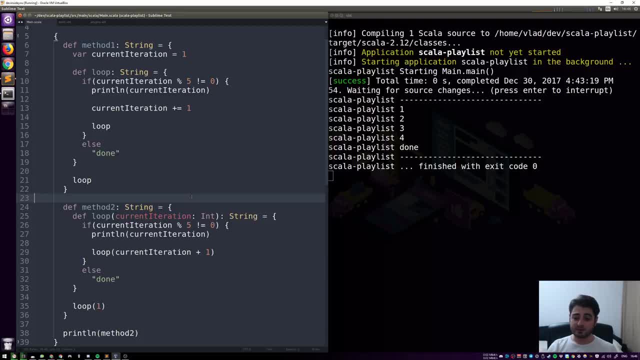 And also, if you're putting something in this pile, you can just take a paper and sharpen it And you can start with somewhere in the middle, right, But the fastest way to take something from this pile is to take something from the top. 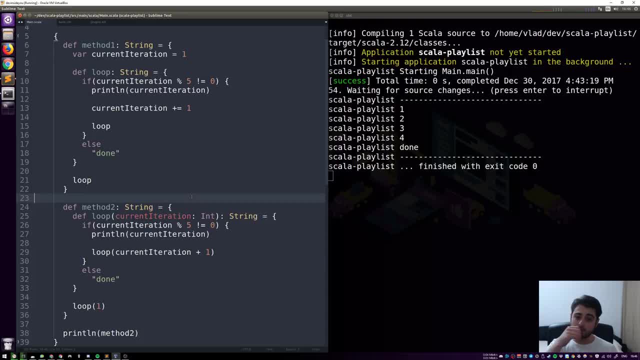 And also the fastest way to put something on the pile is to put it on the top right. So in computer science, when people are talking about a stack, they're talking about a very, very specific behavior. So it's not like in real life where you can just shove something in the middle. 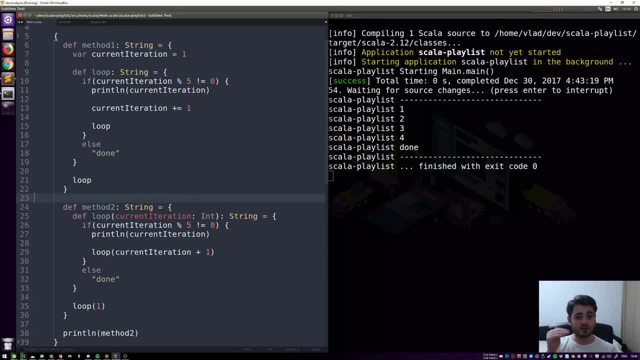 In computer science a stack is something that you can only put things on top And also you can only take things from the top. okay, And in computer science it's called: when you're putting something on the stack, you're saying you're pushing it on the stack. 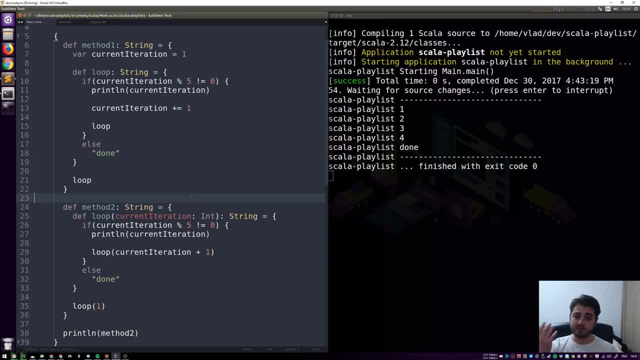 Sorry, And when you're taking something from the stack you're saying: you pop the stack right, So you push and you pop. It is also sometimes referred to as a lightful or lethal data structure And it stands for last in, first out, because the last element that you put on the top. 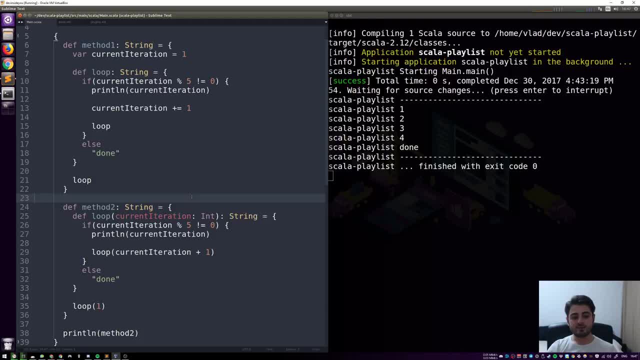 is going to be the first one that you're going to pop. So what does this have to do with programming and what does it have to do with Scala? Well, there are many ways of implementing subroutines, But the most common way is to implement it as a stack machine. 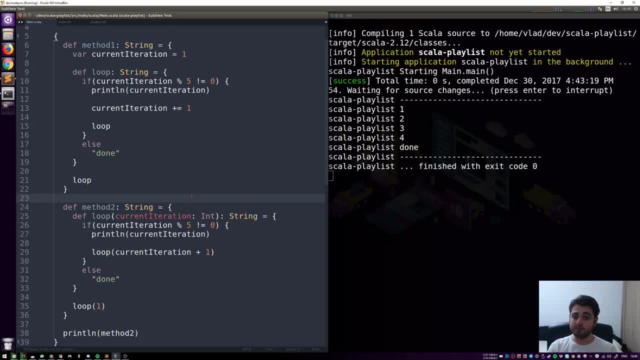 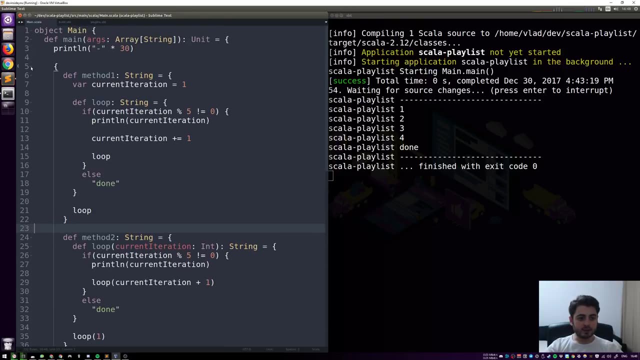 So instead of having actual registers, like a typical CPU, would have the JVM and Java and Scala. they have a stack of subroutines, right? And I'm going to draw you a little picture of what is actually happening, right? So let me collapse that thing for a bit, right? 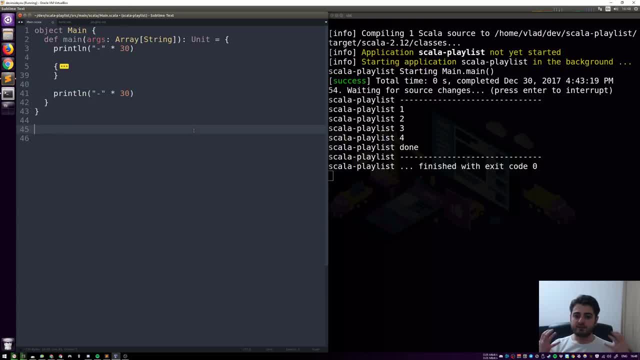 So in every stack frame- right They're called frames- You have the subroutine. So when an application is running, the stack sort of grows and shrinks and grows and shrinks, right. So let's see it for this application, just for a little bit. 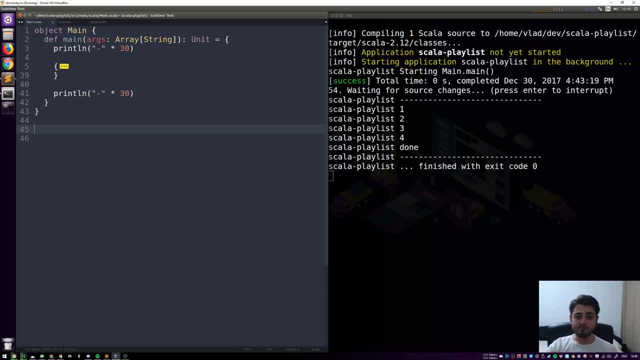 So the first thing that is happening is that this main gets pushed on the stack. So I'm just going to do comments here, right? So I'm just going to say main, right? So this is like a virtual representation of the stack, okay. 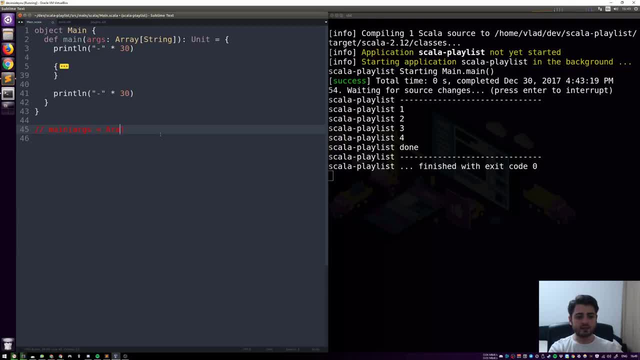 So we have main And the arguments that are coming is an empty area. So both the subroutine and the parameters of the subroutine, the arguments, are stored in the stack, right, And the next thing that is getting pushed is this print line over here, right? 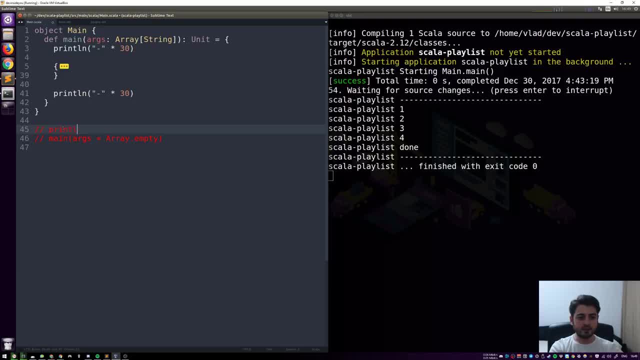 So it's going to be print line, right? And the arguments are the hyphen of the string- Whoops, I'm sorry, The hyphen of the string times 30, right? What is the next thing? Well, the next thing that is happening is: 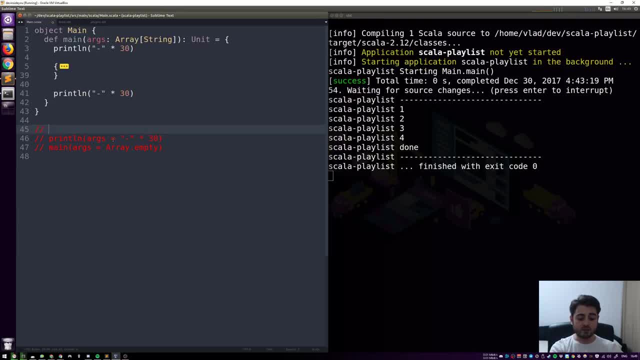 This thing is actually an operation on its own right, So it's just called like this right And it gets called with arguments, and the arguments are a hyphen right And a 30, right. And, by the way, like usually, 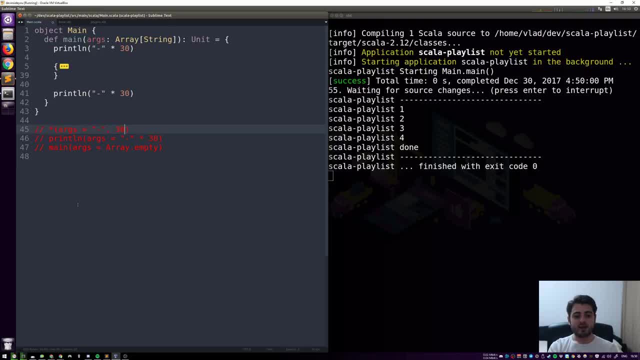 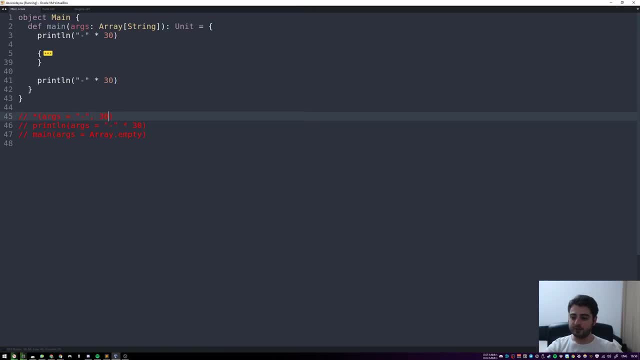 I'm not sure why. I just saved the file. I don't need to rerun anything, right? So usually when people are drawing stacks, then they use a different representation, So they do something like this. Let me copy it because I already got it prepared over here. 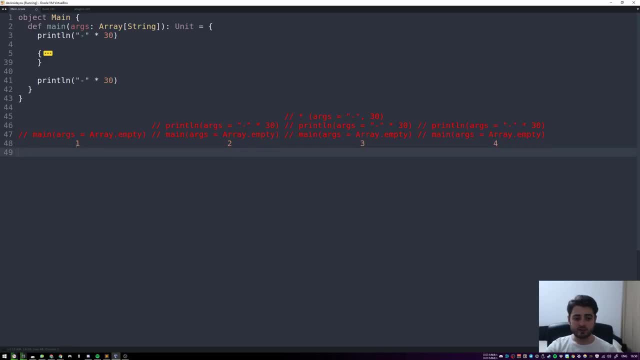 So usually that's what people do, So they just represent the time as in like this. So this is like the first step, second step, third step and the fourth step, because computers are basically clocks right, So there's something that says, okay, do the next thing, do the next thing, do the next thing. 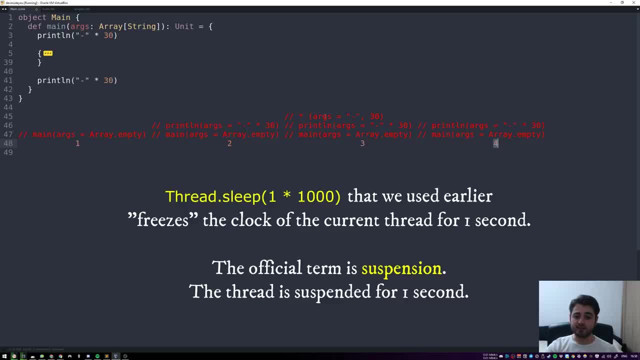 So at first we had the main and the print line got pushed on the stack, then the art got pushed on the stack and then this got popped right, So the stack had a depth. It's called the depth, by the way, the depth of two right. 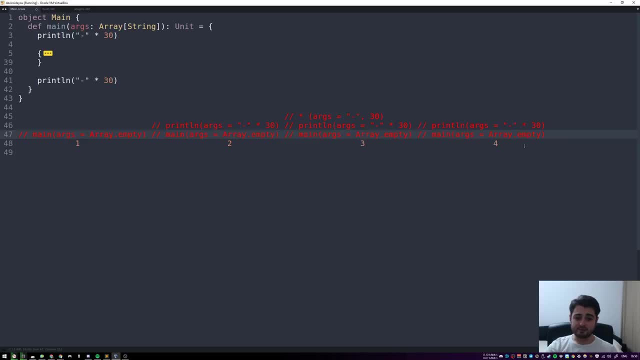 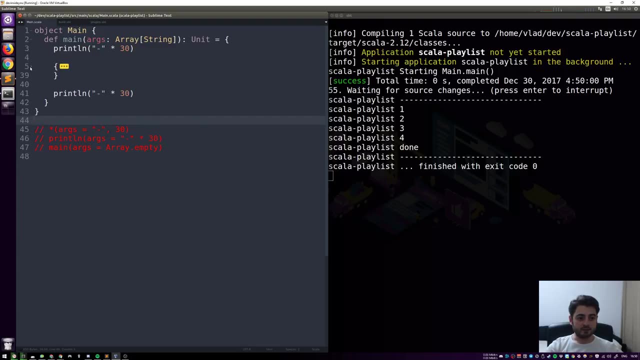 But I'm not going to do it here Because I just didn't have enough space. So let me actually revert that and also shrink sublime again, right? So let me open that thing, that thing, right? So I'm going to collapse method two and I'm going to collapse method one for a bit, right? 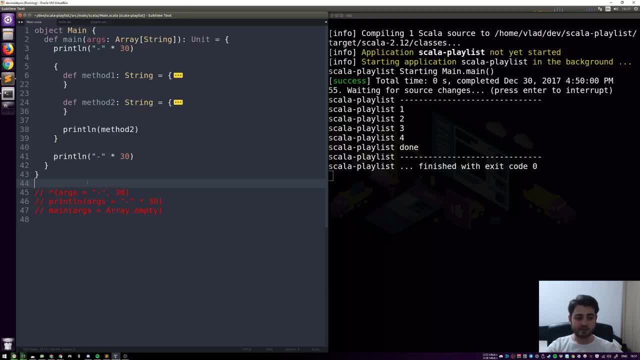 So the next thing that is happening is this one right Print line method. So let's put it down. So I'm just going to keep writing it at the top right. So no, I actually can't, Because this thing got stuck. 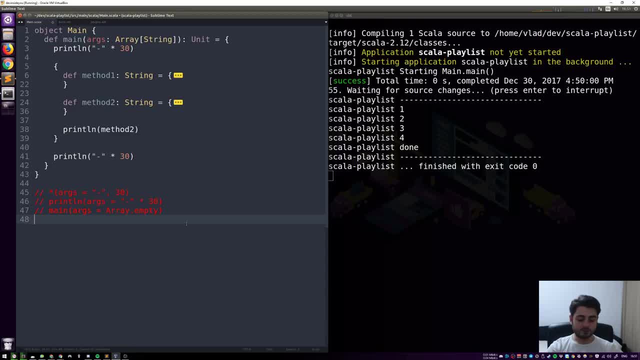 It got popped right. So what we're going to do here is: so this is sort of going to be our time, right? So this is what happened, like at zero, and this is what happened at one, and so on and so on. 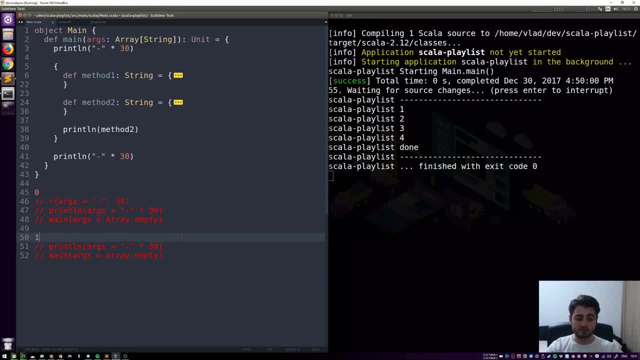 Well, it's actually not zero and one, But you know, like this is sort of like the next relevant step for our discussion, right? So the next thing that got pushed was this thing, right? So we got print line and the args as method. okay. 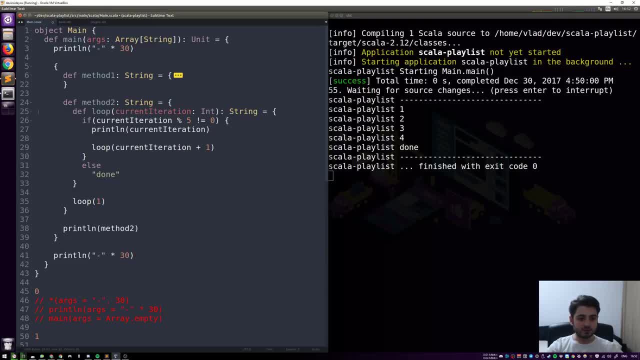 So no. method two: okay. So in method two, let's collapse. loop and the first thing that's happening is loop. was one okay, So let's do it here. So we're going to have loop and arguments. was one okay. 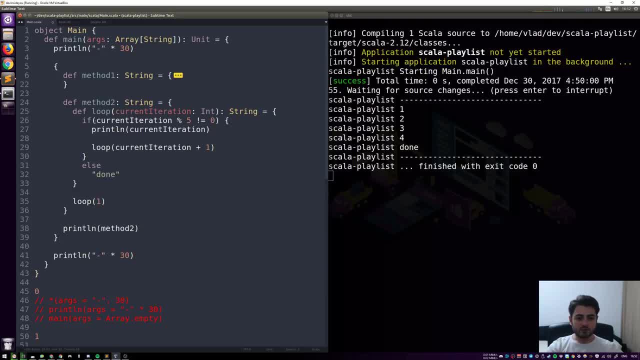 And then we're going to open this and we're going to ignore all of this, right, So we're not going to do this and we're not going to do this print line. The relevant thing is here, right, So the argument was over here. 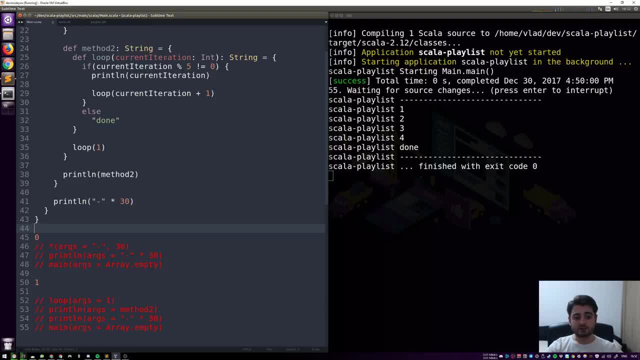 The argument was one, right, So we're going to have. So we have a one over here, right? And the next thing that's going to happen is it's going to call loop was one plus one, So it's going to call loop was two, right. 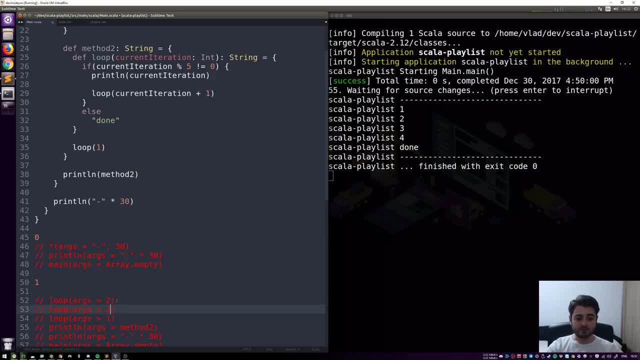 So I'm just going to do this right, And then it's going to keep doing that right. It was a three. It's going to keep doing that. It was a four. It's going to keep doing that. It was a five. 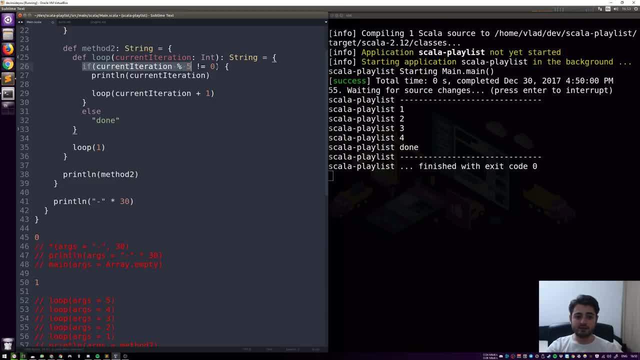 And then when it's going to call, it was a five, it's not going to end up here, It's going to end up here, It's going to be done right, And then it's going to start removing those things, right. 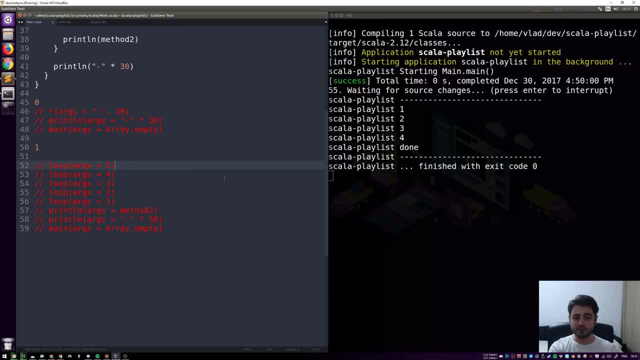 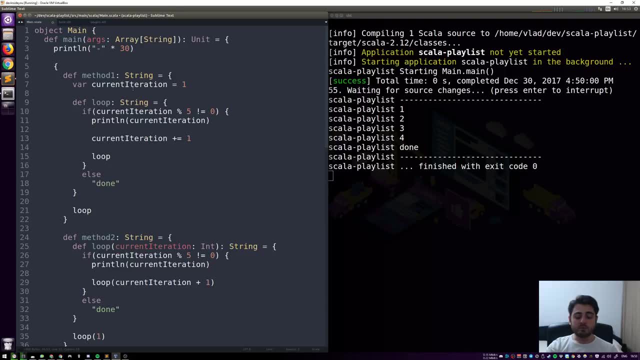 those things. right, it's going to start doing this, this, this, right, and so on. okay, but let's leave it like this for now. so now we see that, uh, in the first example, right, uh, we were managing our memory ourselves, right, we have one thing and we were just changing it all the time in the second, 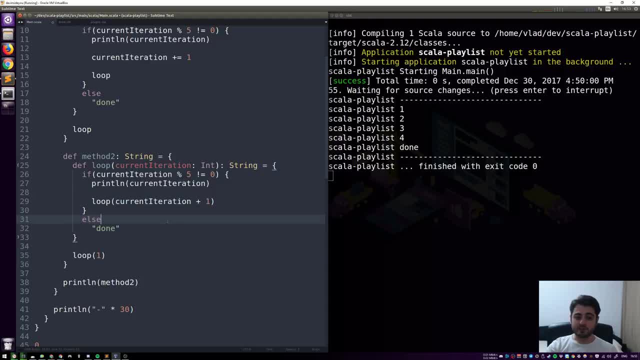 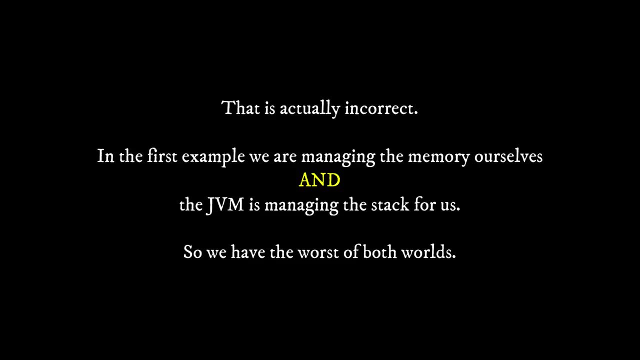 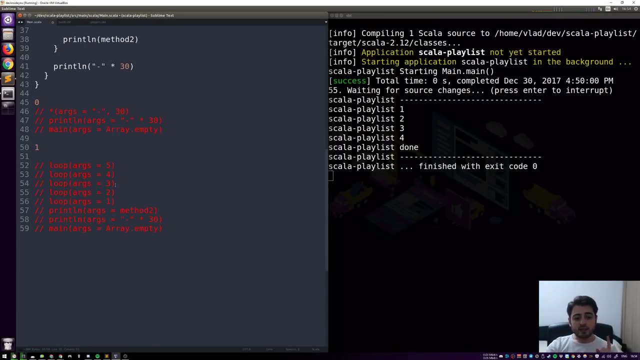 example. uh, our memory gets managed by something else, right, by the stack itself. okay, okay, there's a problem with it, though. right, it did not use only one variable, it used all the five stack frames. right, so it consumed more memory, right, and memory, uh, even though it's cheap, these. 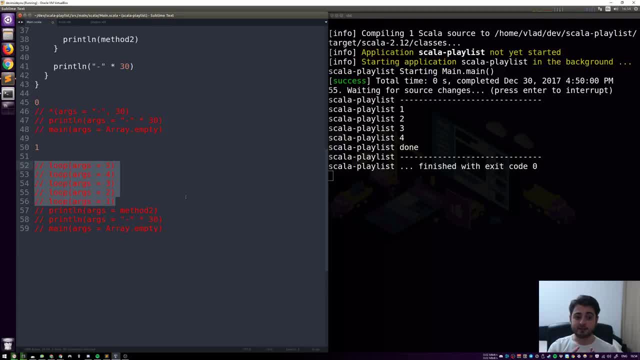 days. it's finite, right? so there's an end somewhere. and in order to demonstrate that, uh, we're actually going to go back to java, i will explain the reason why we're going back to java in in quite a few minutes in the video. um, as of right now, just just bear with me. so, um, we're just going to. 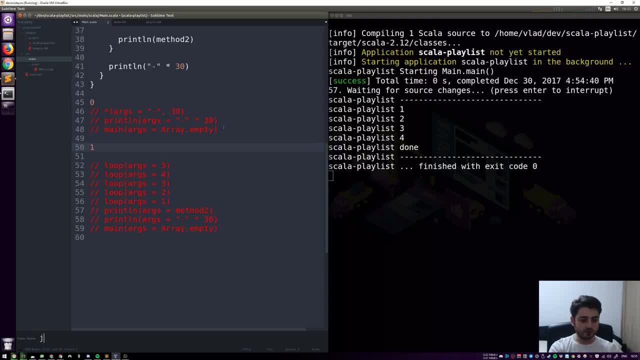 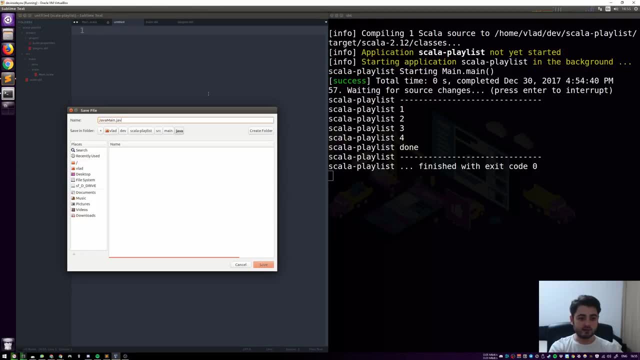 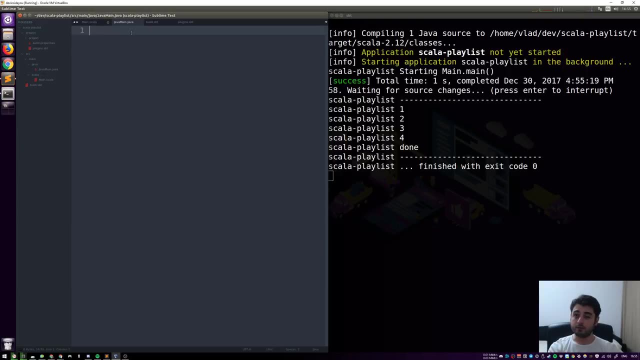 have another folder here here called um java right, and inside we're going to have a file called- let's call it- java main- java right. so spt can also compile java if you have jdk installed, and we have installed it in the video number two, i think. so we're going to have a um public class. 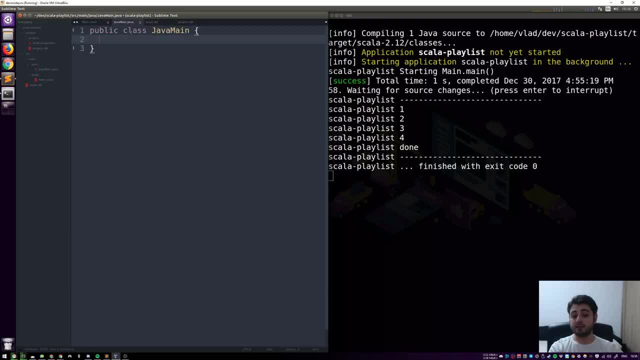 java main because, remember, in java it has to be um called, exactly the same as the file is called, and we're going to have a public static void main. i'm going to string whoops, come on there, we go arcs right, and what we're going to do here is we're going to 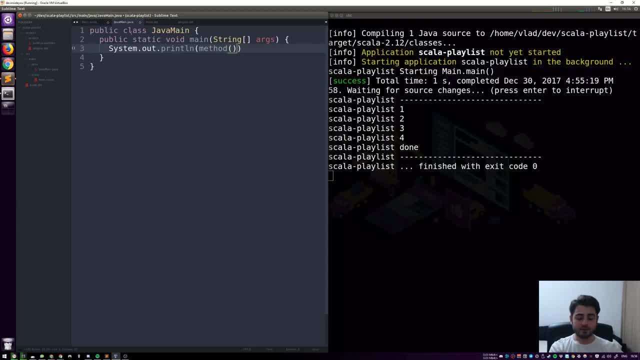 system out inline method, okay, and uh, so remember that thing that we started with in scala, we had method. uh, string equals method, okay. uh, well, we're going to do. we're going to do- a very similar thing in java, uh. so, um, in java you can't have methods inside of methods, uh, so we're just going to have. 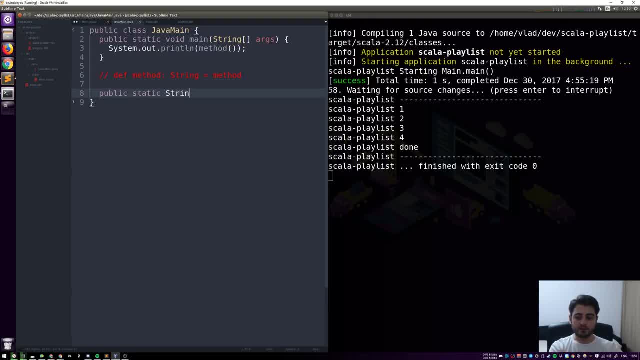 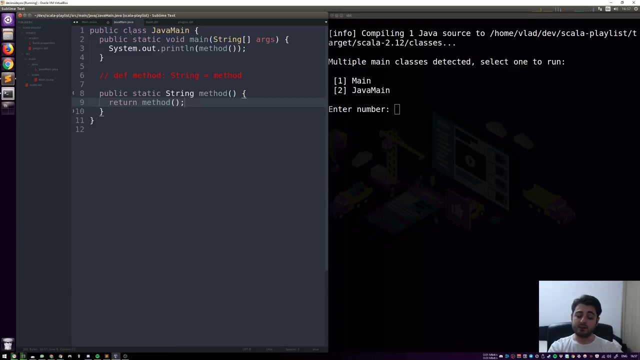 a public static and it returns a string and we need the parentheses and we need this awkward syntax and we need to return um. oh, by the way, we have to give it a name method, okay, and we're just going to return itself. okay, come on, gonna return itself, right. so now, if we save it, um, revolver or spt, they both. 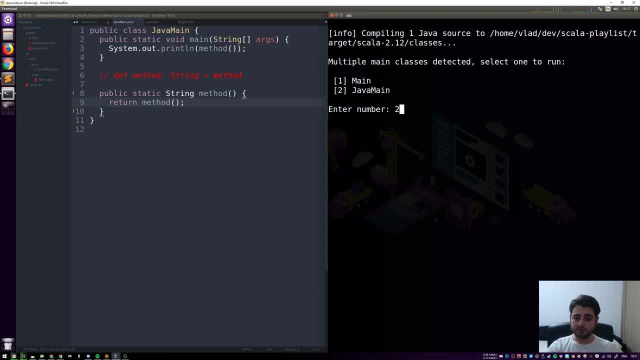 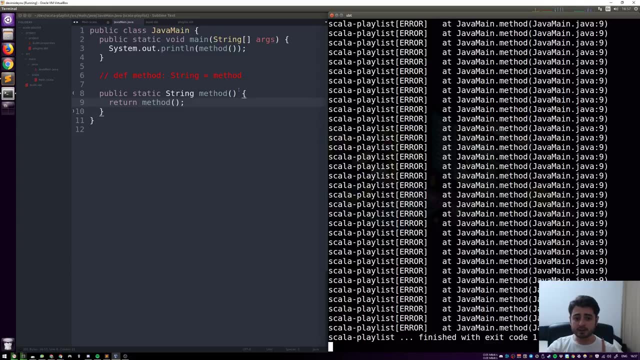 recognize. okay, now there's a different main method, uh, so we're just going to do two, right? so what's going to happen is that? uh, there is there, there's, there is a problem, right. so in scala, remember, uh, it was just just caught in this endless loop, right? whereas in java something is exploding. what is happening is it? it kept. 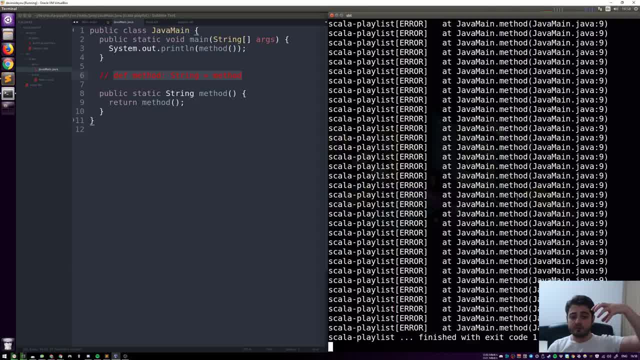 calling itself too much right. and then the stack grew so long right so it was so deep then just consumed all the memory that it had. now it is possible to configure the jvm to just have it to just have more memory, but the problem is still not going to go away, right? because over here 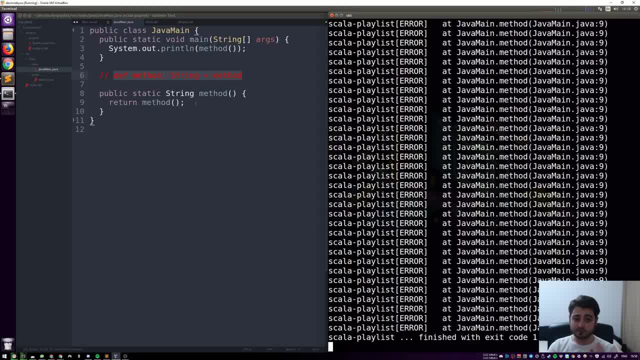 nothing's nothing stops it from calling itself, so eventually it's still going to explode. uh, it's gonna explode, but it's still going to explode, right? so that's the problem with the stack overflow error. there's this whole concept of uh exceptions that i'm going to explain in a different 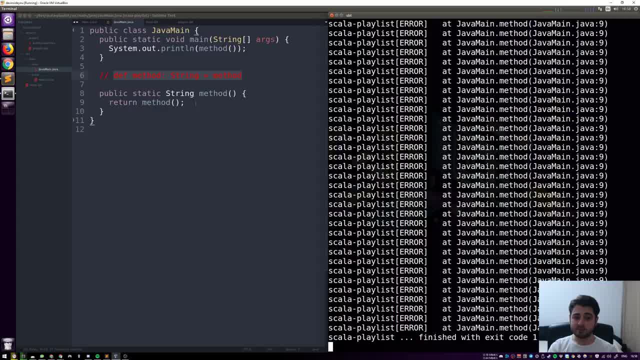 um episode. uh. well, basically we have, we have a runtime, we have the jvm that make sure that we're not going to do anything stupid, right? so whenever it um notices something, something like that, uh, what it's doing is it's basically wrapping a stack, uh, with some some sort of like guards, all right. so 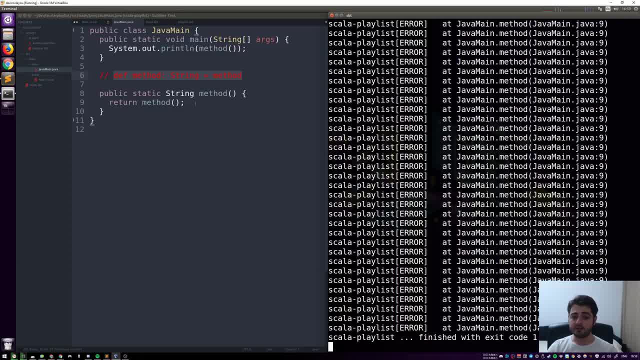 there are things that are always looking at the stack and when weird things are happening, it it's throws a so-called exception and when the exception is not handled, it's running on, it's going to die and, as of right now, we have only one thread, the main thread. 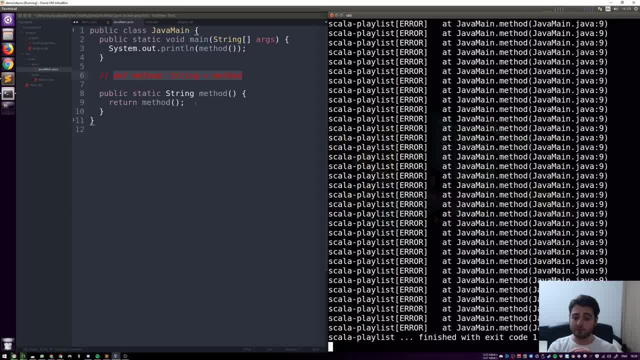 and basically means that that the whole jvm is going to die. so basically the whole, the whole program is going to crash. so it finished with access code one. because it crashed. okay, uh, you don't see that, it's actually, uh, throwing a stack overflow error. uh, because it's because we need. 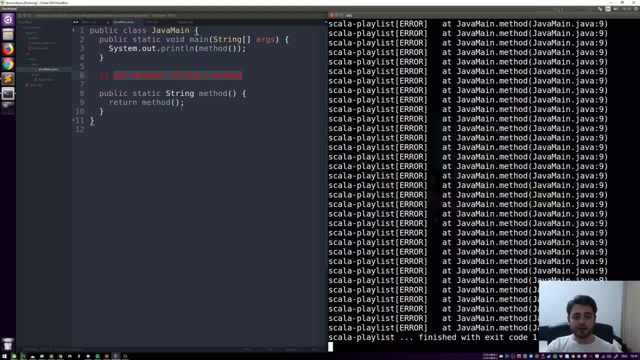 to scroll up like like a lot, right? so in order to demonstrate that, uh, instead of having this thing, uh, we're just gonna throw, uh and we don't need, we don't need this. okay, to throw a new stack overflow error like that, okay, oh, and, by the way, if you have multiple 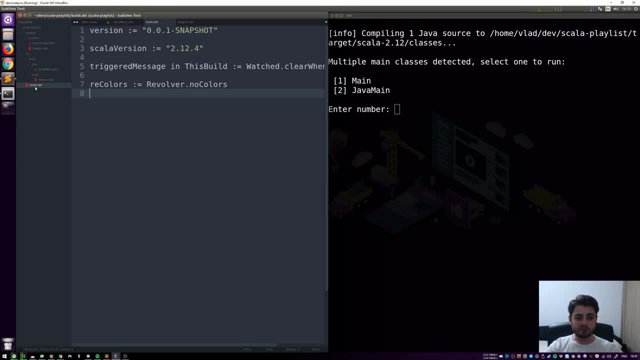 means uh, you can uh go to buildspt right, and you can just uh put in this thing. you can say, um, main class in restart colon equals sum, and then you just give it the name, and in our case, um, let's say java main, right, and then, uh, you would. 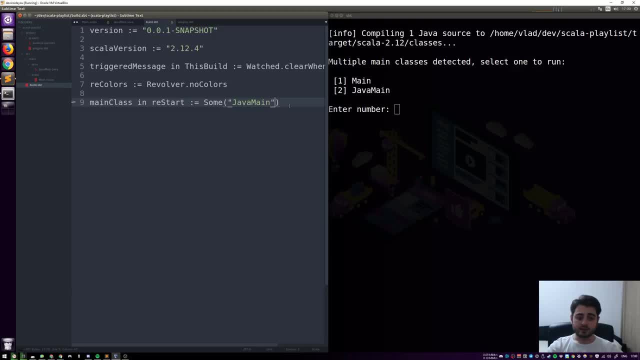 need to reload and it just just wouldn't ask. you just would always run this. so i don't want to have this, right, so i'm just gonna, i'm just gonna remove it again, all right. so, um, as of right now, i'm just gonna, i'm just gonna say two, right, so, uh, what happened now? is it said? uh, exception thread main. 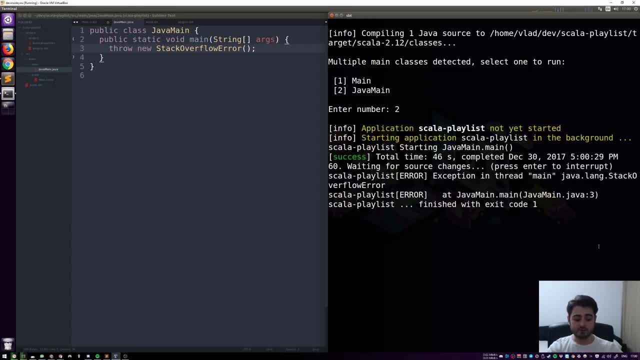 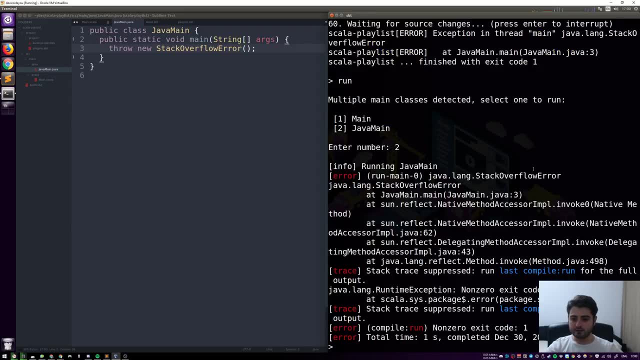 um, java long stack overflow error. and, by the way, if you don't do this without the revolver right, so if we press enter and we're just going to do run and we're going to say java main, then you see, you see, like this stack overflow error and in fact, let me maximize the terminal. 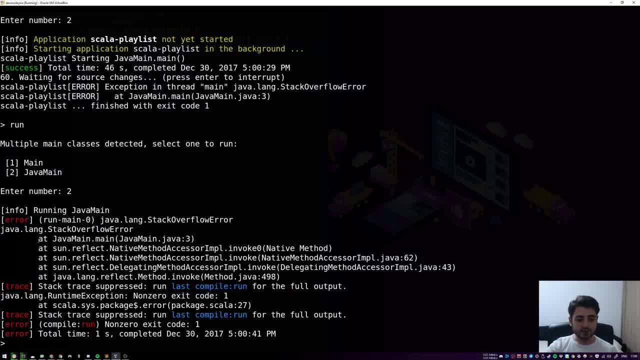 so you see stack overflow error and, um, what you see here is exactly is exactly the stack. it's called the stack trace, right, so it shows. okay, so it called some native method, um, some you know somewhere deep in the jvm- and then it called this one, and then they called that one, and then they. 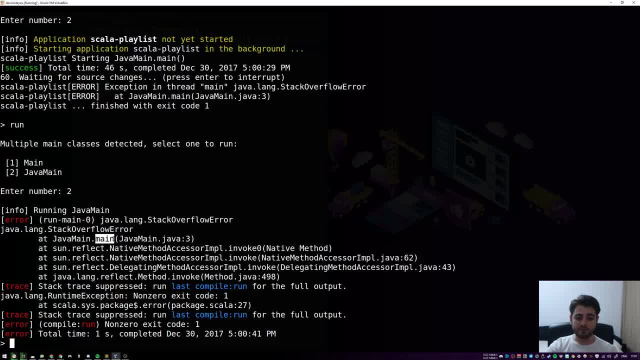 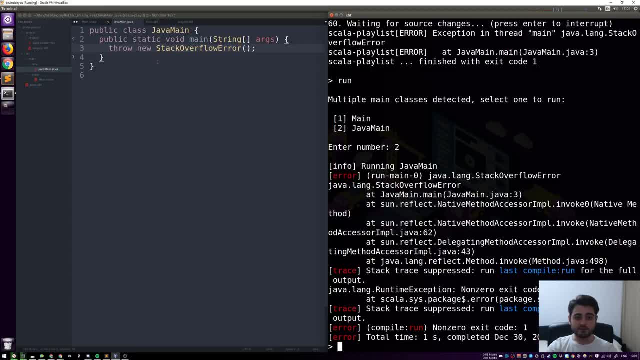 called that one and then eventually it called the main method, right, uh, and it's in the file called java, mainjava, at line three. so if we go back to line three, uh, we're gonna see here. right, so it called main and this is where it exploded, okay, so, uh, what we also see here is: 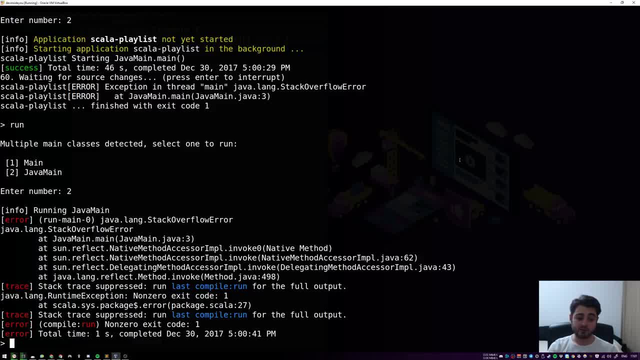 that, um, those exceptions- that again we're gonna have a separate video that talks about exceptions. uh, so there's, there's sort of hierarchical right. so, uh, there can be an exception instead of exception inside of this exception, and so on and so on, and so on. so what we have here is a runtime. 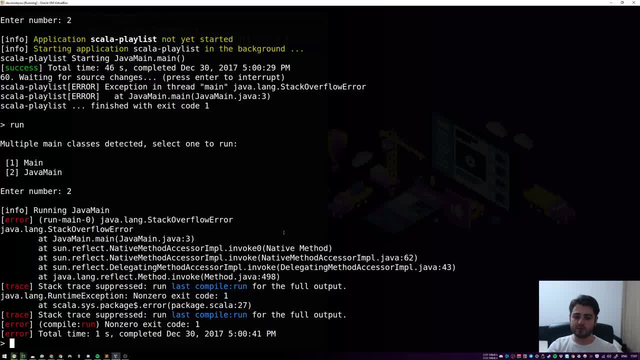 exception and inside of it there's a stack overflow error, right. so spt somehow caught it. caught it as well. so basically, what i'm saying is that if the stack trace is very, very long, then in the end you won't even see this, right, you're going to see this like in the past. you 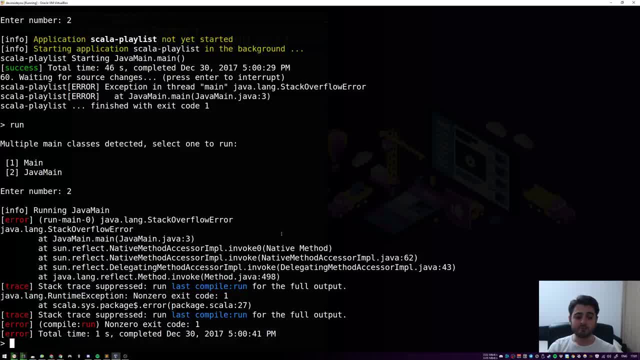 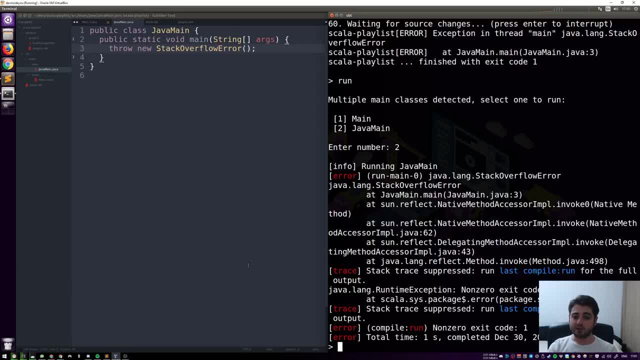 would actually see like at the very bottom. it would say, hey, it's a stack overflow error, right, and by the way, if you google that you're, you're actually going to find a page called stackoverflowcom. it's a website for uh, for questions and answers, and they're not paying. 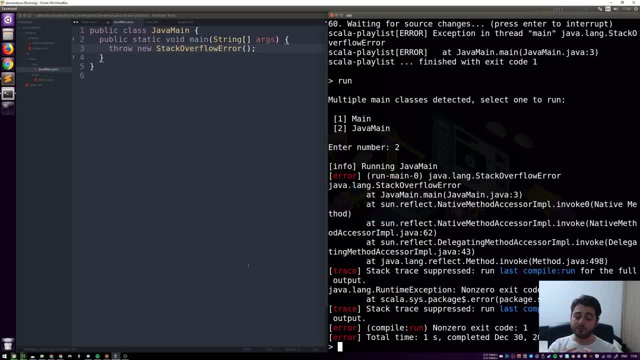 me anything to um to say that? uh, i'm just saying that, if you want to explore this thing a little bit, if you google for stack overflow, you're probably not going to end up at this. so google something like cycle flow concept or stick overflow in java or something like this. all right. 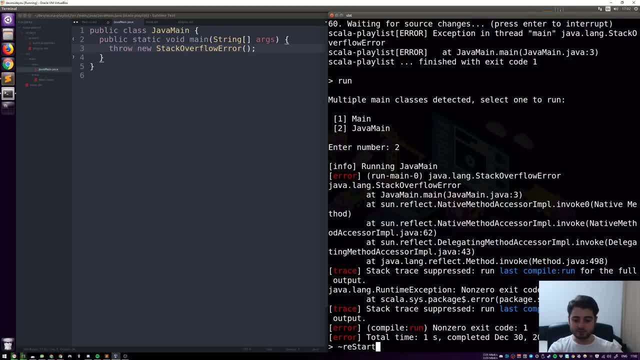 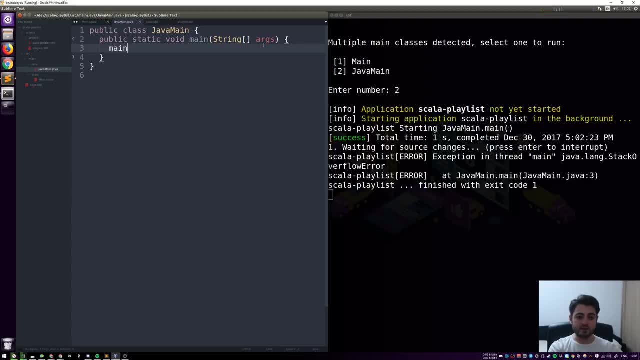 before we can, before we continue, uh, let me go back to um, to this right, and let's just say java, okay, once and um, let's do this. the very simplest way of doing recursion is this right. so this is the very the the simplest way of producing. 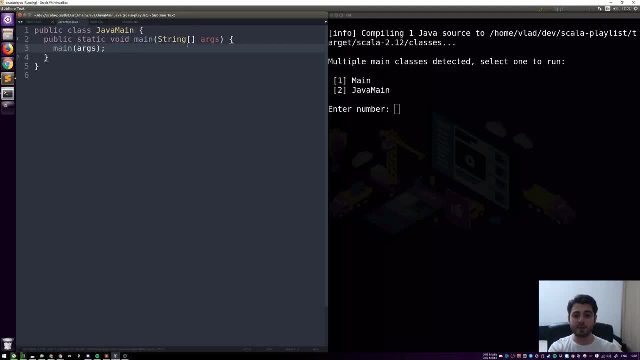 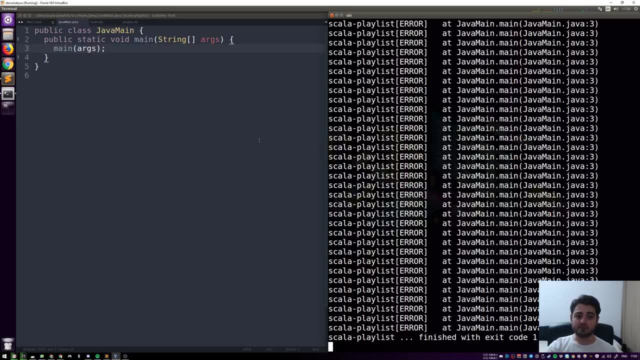 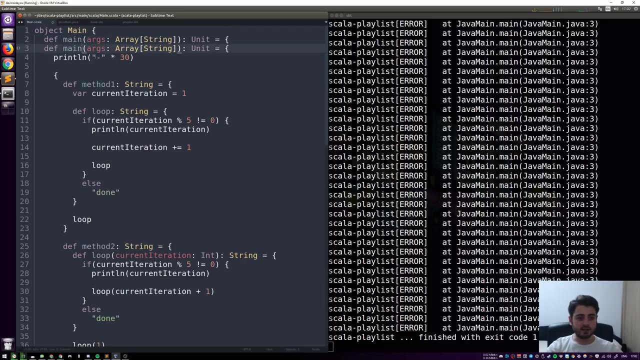 a stackable flow. of course, we've got a semicolon, because java has semicolons, okay, so, uh, let's try this one, right? so this is a stack overflow. this is not happening in in scala, however, right, we've already seen this, but let's actually reproduce it. so let's, um, uh, let's, let's duplicate this line and. 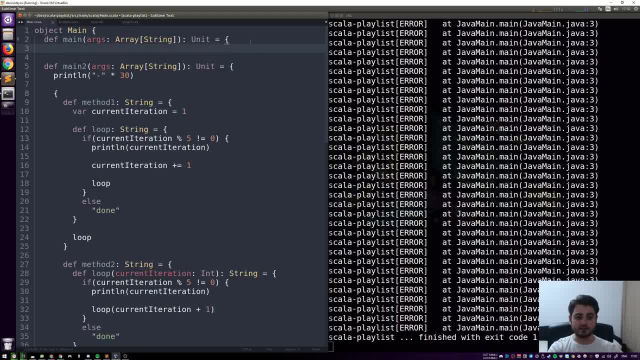 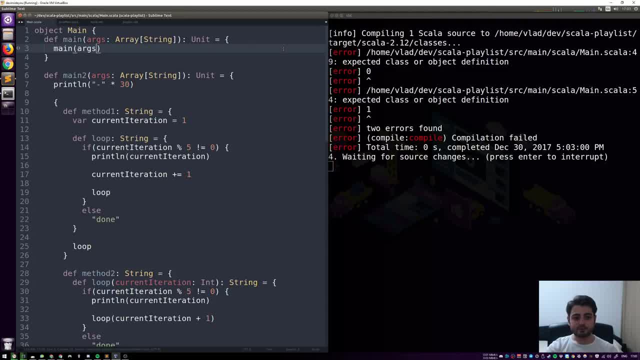 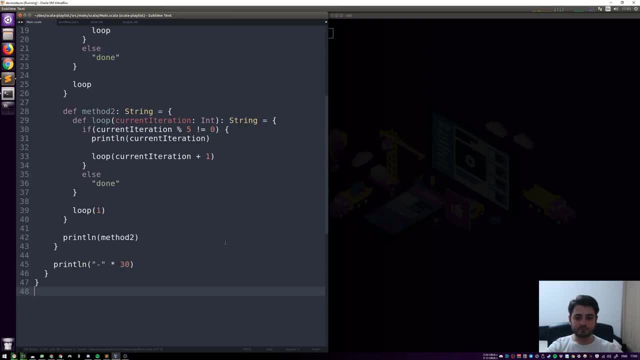 call it main two. so now, spt is not gonna find it, it's gonna, it's gonna only uh find this one and do exactly the same thing. we're just gonna call it main with arguments, right so now. um, oh yeah, we had this zero and one. let's let's remove all of that. yeah, let's remove all of that, right, so now. 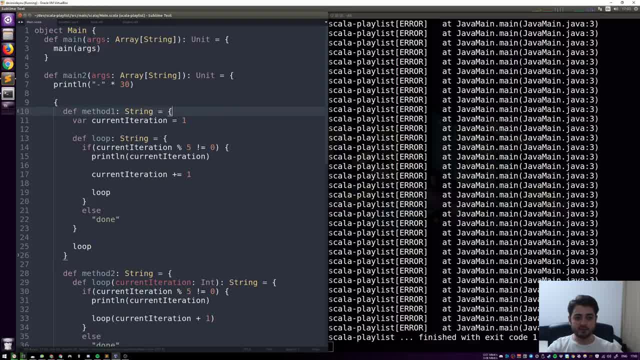 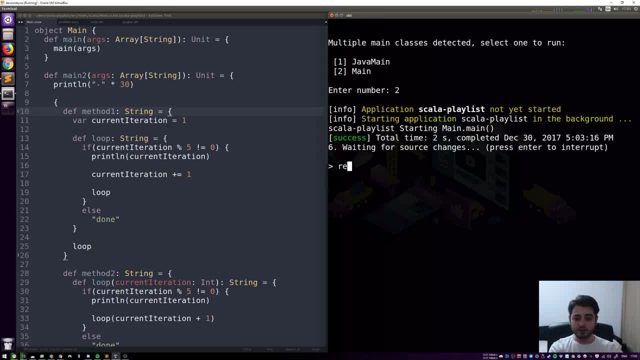 we're gonna. we're gonna do java again, right, i'm gonna save, and now we're gonna do scala and it's kind of like it's just caught up in this endless loop, right? so if we do, uh re status, right, it says it's currently running and you see it based on my cpu, so scala is doing something. 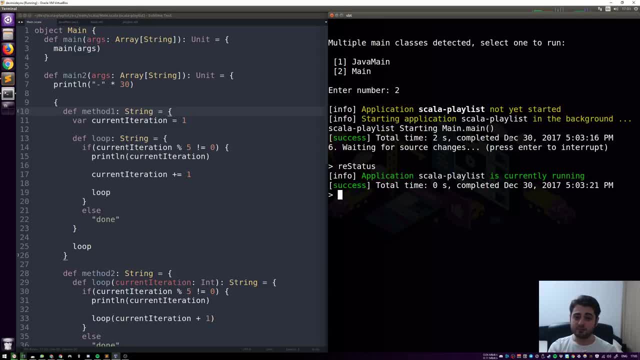 really magical behind the scenes and we're gonna see what it what it is actually doing uh, behind the scenes to make to make it work. so, as of right now, we're done with java. so, uh, we're just going to uh restart with a tilde and let's just go to the java main and just comment it out right, so that 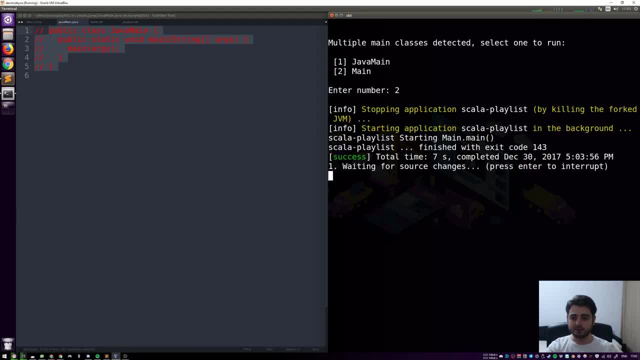 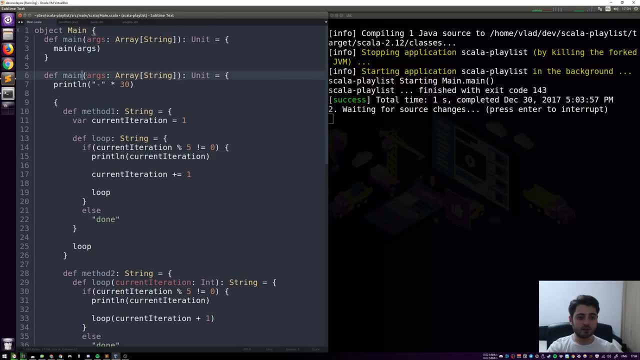 we don't have to, um, to choose the one that we want over here. let's do this one, all right, okay, so now we're back to normal and we have our- uh, let's do this one now. remove that. all right, so we're back to normal and we're back to normal. so we're back to normal. so we're back to normal. so we're back to normal. 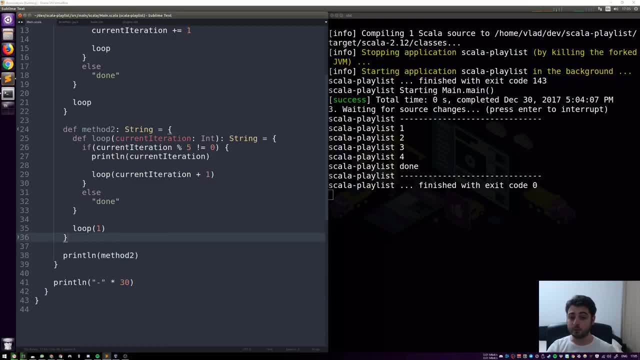 now, before we discuss how, um, what scala is doing, like, well, what is this magic that that is doing? um, a valid question would be: uh well, what are you gonna do if you're not in scala, right? so what are you? what are you gonna do when, when you're in java, right, and it turns out that java has a very 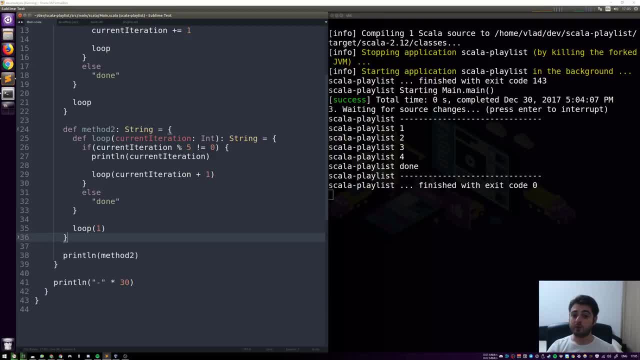 special keyword- and it's like most programming languages have this keyword like- called while. right, that makes sure that for algorithms like this, it does not create this, the stack frame, right. so you don't have to use recursion, you can just use while and you don't have to, you know. 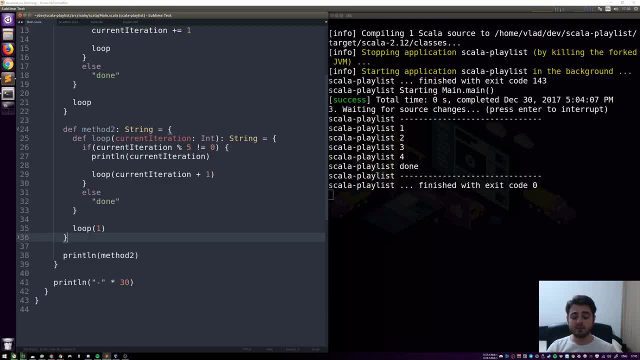 you don't have to call yourself all the time, right. so, uh, one of the main uh design goals for scala was to to remain as uh as java compatible as possible and also to be to be friendly for java developers, because then you know, they were hoping that you know all the java developers would jump. 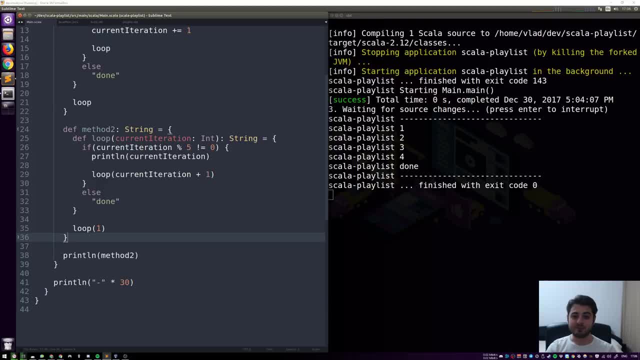 ship, right? uh, they really happen, but, um, this is a topic for another video, right? so, uh, scala also has it has this bio keyword. so you know what it's time for. it's time for method three, right? so let's call method three, and obviously it doesn't exist yet. and for method three, i'm gonna maximize supply. 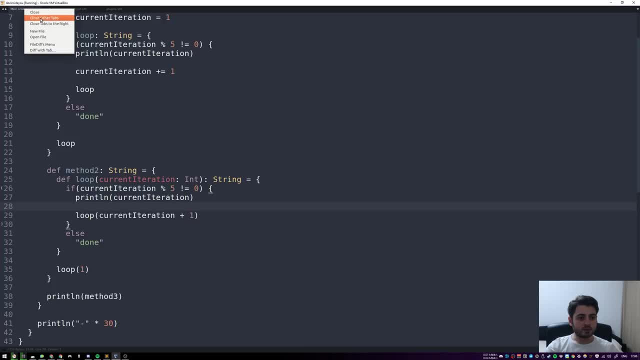 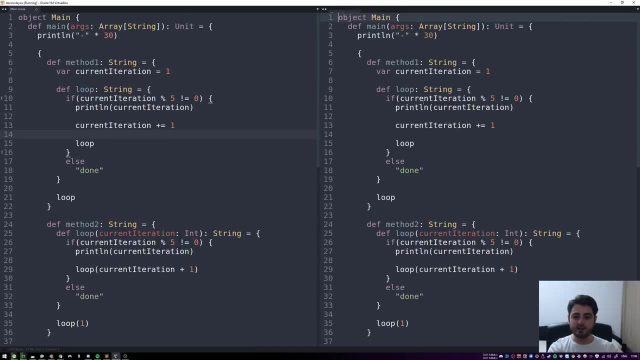 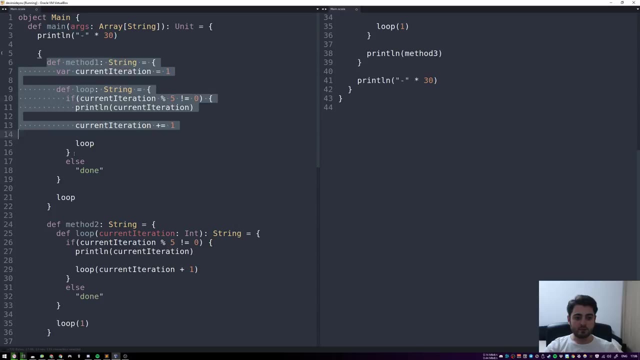 right and i'm going to split it. uh, actually, let me close all the other tabs. let me close all the other tabs. i'm going to split the screen right and on the right i'm going to open the same file right, and i'm just going to scroll down a little right. so, uh, we're going to copy method one. 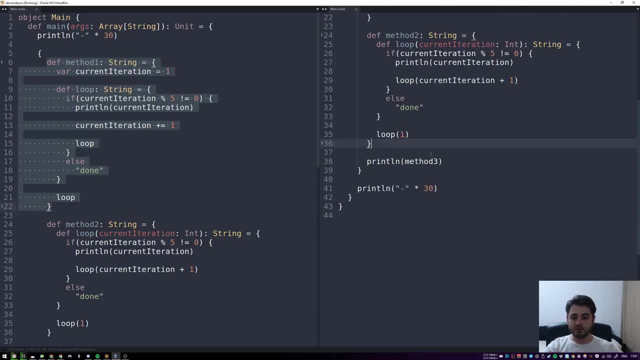 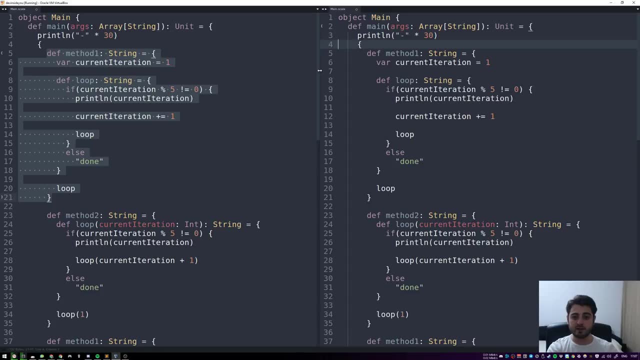 right, and we're gonna. we're gonna put it under method two, okay, right? so see, i'm editing both files, right? so if i scroll up and i do something like this and we're editing both files, okay, so i copied the first method method over here and now i'm going to call it method three. 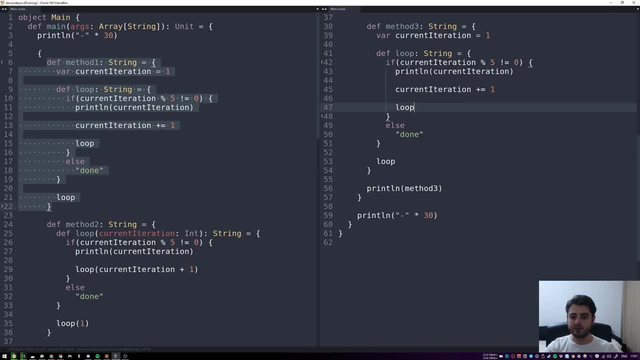 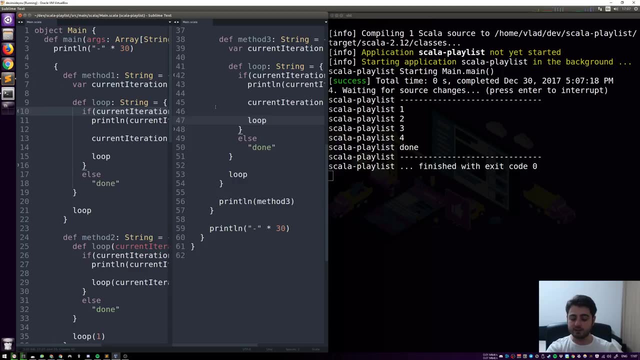 right, and now everything should still work right, because now we're calling method three and the. the code for method three is exactly the same one as in method one, and i'm doing that. uh, actually, let me, let me, let me show you okay. so see, it's actually working. let me, let me save it, so that 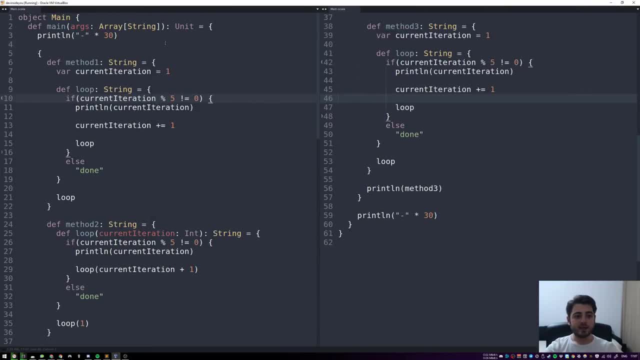 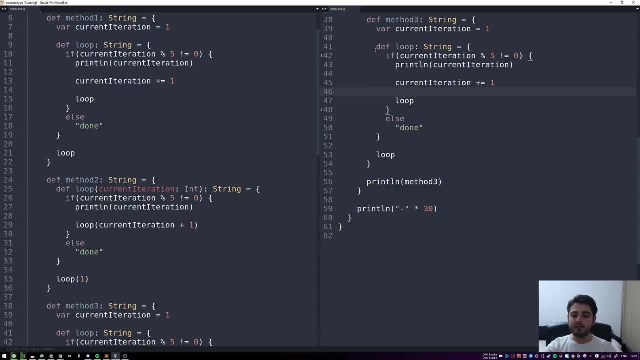 you're. that are your shortcuts. it's actually working. okay, let me maximize it again and i'm going to scroll down this exactly to method one, and we're going to have a method three over here, and over here we're going to have this while loop: uh, so that you just see, uh, both of them at the same level, so that you see that. 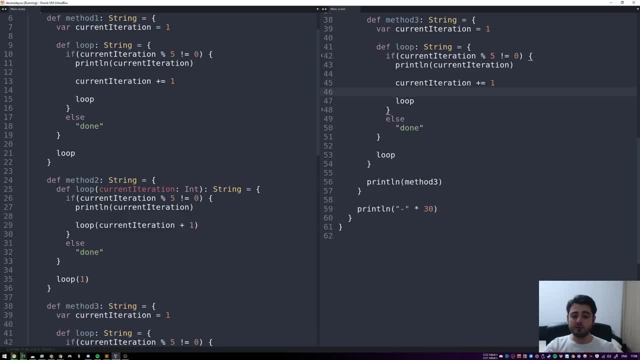 how very similar. uh, they, they actually are all right. so the while loop looks exactly like an if expression, right, but instead of if, we're saying while okay, and a while doesn't have an else, so we're just going to remove the else and basically, when, when while is done, it's. 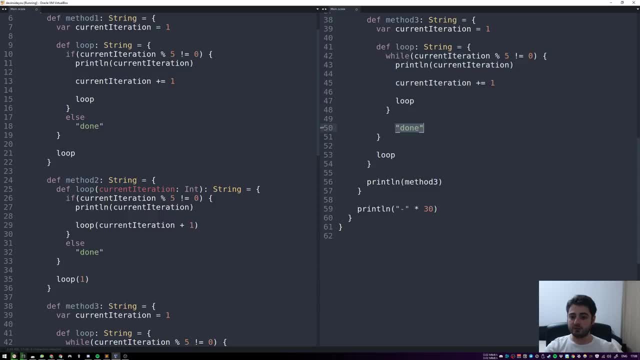 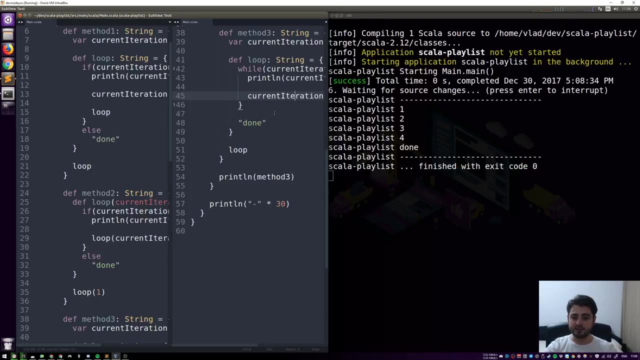 just going to return done, right. so loop is just going to return done, and because we have a while is doing the loop for us, there is no need to call loop right. and if i haven't forgot anything, uh, we're actually already done, right? so see if i just saved it and it ran again, right? so, um, how we're. 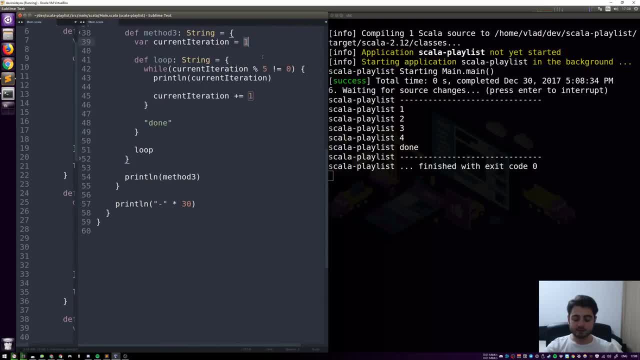 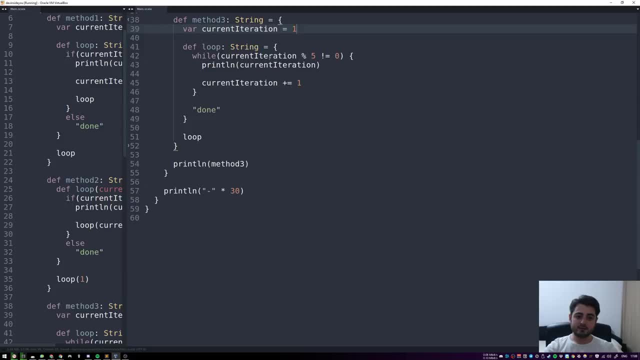 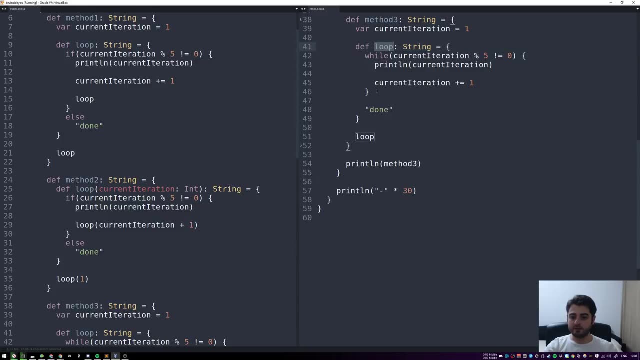 gonna do this. let me see, um, let's run it with zero, it's gonna be done. let's run it with one, it's gonna be done, right. and uh, let's maximize it again and do that, okay. and now, because there's no recursion, uh, anymore, right? so we're just creating this staff and then we're calling it right away. 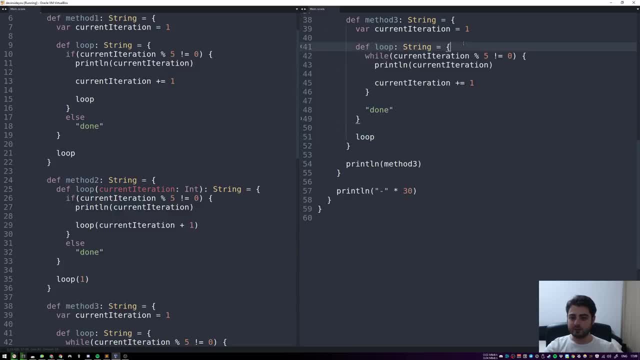 now there's no need to call it right. so we already have a while of. why do we need our own right? so we can just remove this and remove this curly brace. and now we're just going to indent this thing over here and we're not, we're not going to need to call loop right. so this is. 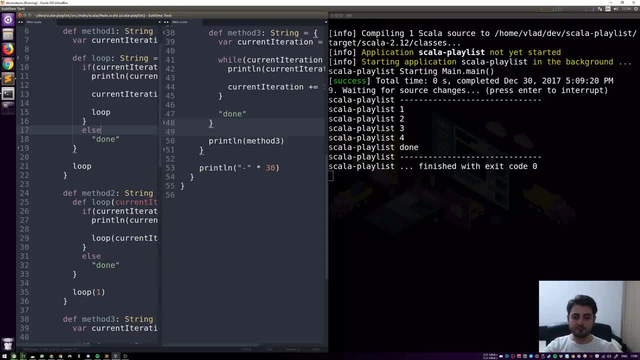 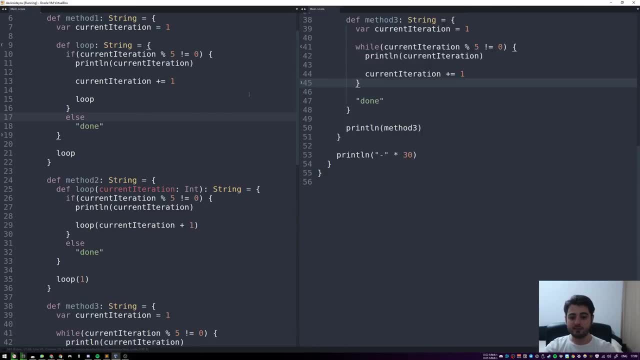 the method three. this is the while loop. exactly the same thing. um, i've forgotten. yeah, i just pressed save and it ran, but you didn't see. so i'm just going to press save again and then it's running. it's exactly the same thing, right? so let me maximize it again so that you can compare it. 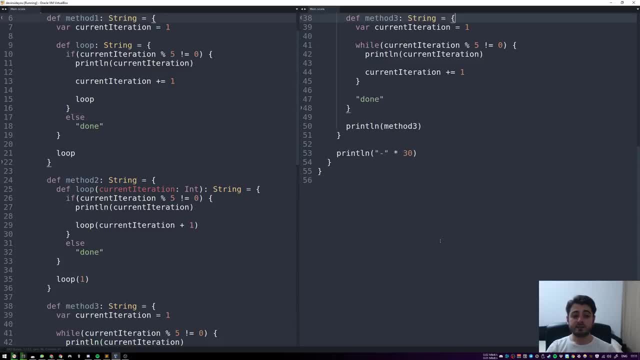 right and, uh, play with it. so what we have here is three different ways of implementing the same thing, three different methods: right, method one, two, three, and you see them all in in one screen. okay, and i'm just gonna say it again: in java you're pretty much stuck. was was only this one. 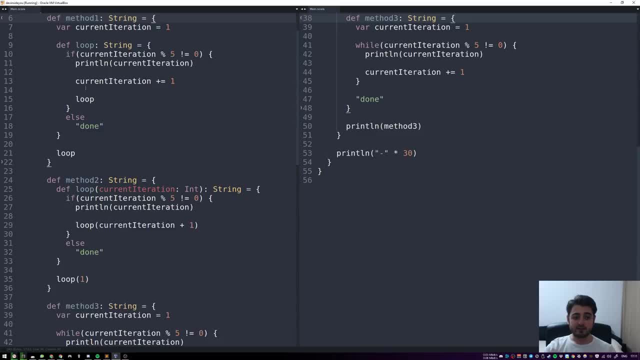 right because, uh, this one just consumes the stack, right, it just calls itself right, and this one also just calls itself all the time right, so it's going to consume the stack. so, if the number, if the number is right, it's going to consume the stack. so, if the number is right, it's going to consume the stack. so 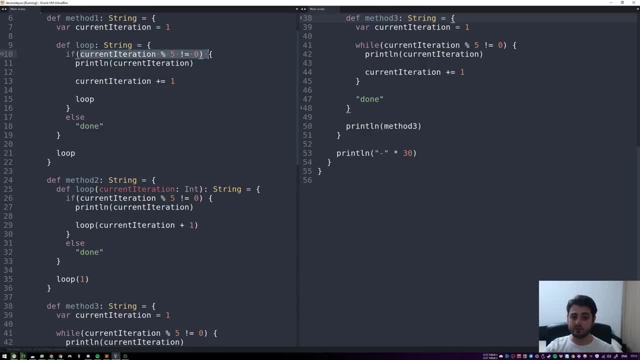 really really, really, uh large. or you know if the condition you know is if there's something wrong with the condition, or you know if you're just going to do this for way too much. the memory is just going to run out, okay. so in in java, you're pretty much stuck with this. in scala, you have a. 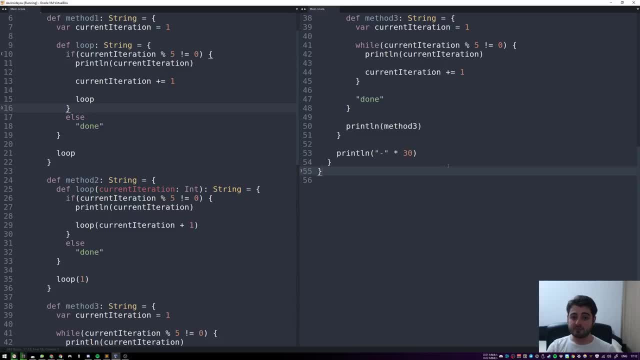 choice we're going to discuss in a second. uh, uh, what exactly is happening behind the scenes right before we continue though? um, just just, just, uh, you know a sidebar, a side note? uh, you can't do this with functional literals. remember, like in the previous video, i introduced the functional 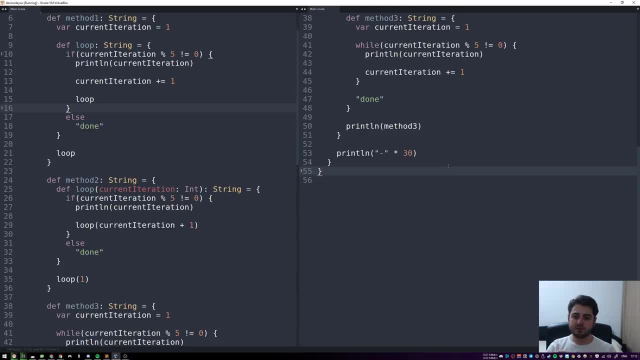 literals and so instead of just devs, so functional, functional literals they can't actually call themselves because there's nothing to call right. so there's no, there's no, there's no point of reference, and this is why they're also sometimes called anonymous functions and they're also called 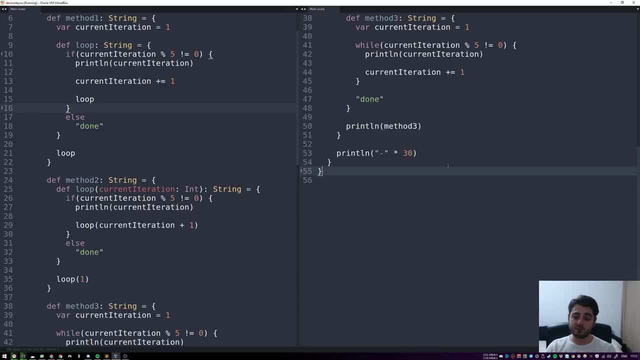 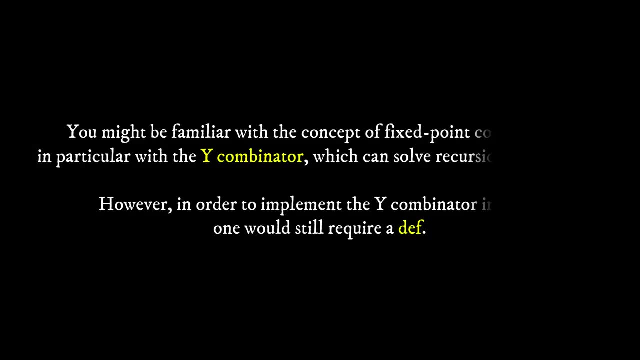 lambdas because they come. they come from this branch of computer science, or actually math, called lambda calculus, but we're not going to talk about them today. it's, this is just just a sidebar, all right, so let's talk about the magic that is happening behind the scenes. 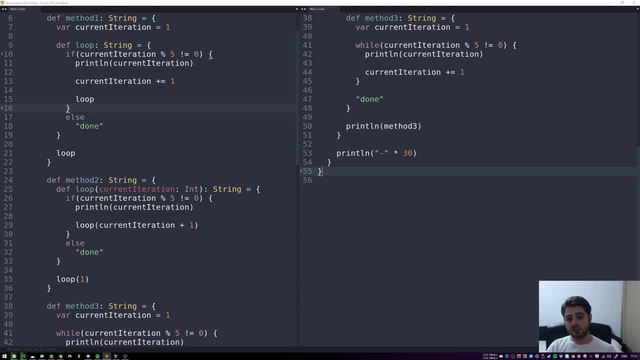 so what is happening behind the scenes is an optimization of tail recursive functions. so what are tail recursive functions? well, if the last thing in a recursive function is either just a value, right so if the function just returns a value, or if the last thing, like in every branch, or or if it. 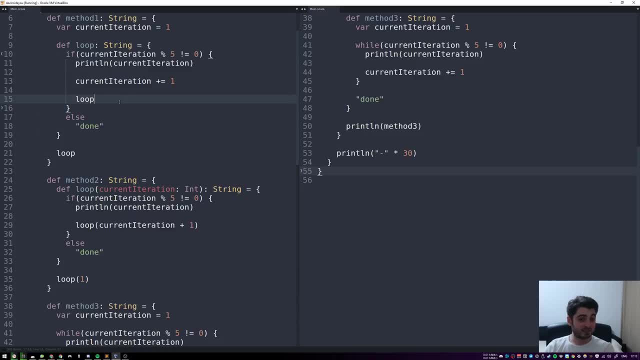 just calls itself right if it's the last thing. so if it's in the tail position, right, because tail is in the back usually right. so if the last thing. so if if the recursive call is in the tail position, it's called tail recursive, and in Scala if the function is tail recursive, then sometimes it can. 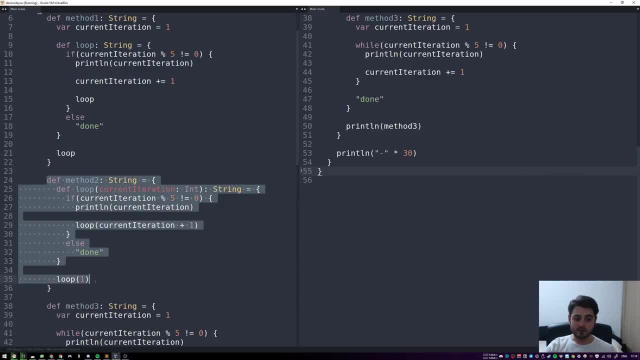 convert this algorithm right or this algorithm into that and, as we already learned, this is very efficient. and, by the way, on the on the CPU, this is converted into go tool instructions, right. the thing is that, because of this, right if it's not the last thing, right if something else is happening. 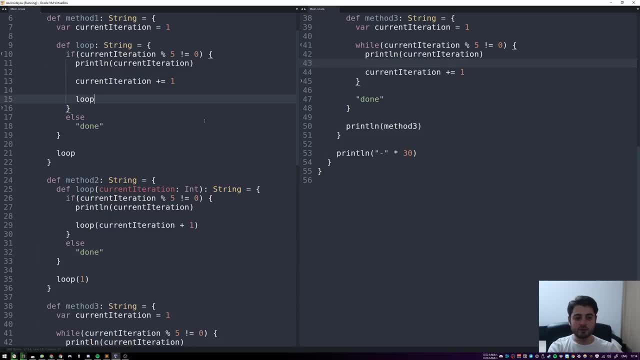 right, for example, um, we're returning a string here, right? so if it would be a loop, uh, plus, uh, I don't know, add something else to that string, right? so this, this, all of a sudden, this would be the last thing that is happening, right, because at the end it would boil down to to go to statement, right, uh, there? 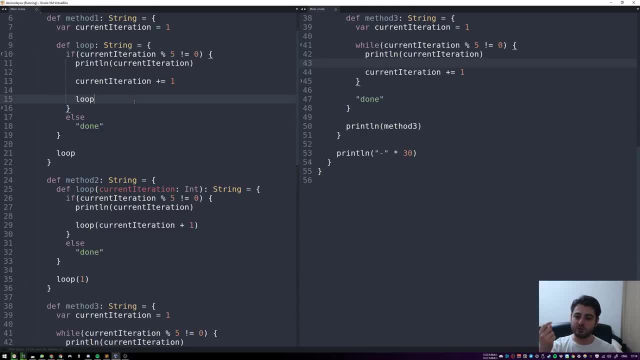 is no way for the go to statement to come back right, because it just doesn't store this, this point of where to go back right. so, uh, in Scala, what you can do to be sure is you can add an annotation right, so you can add an annotation. 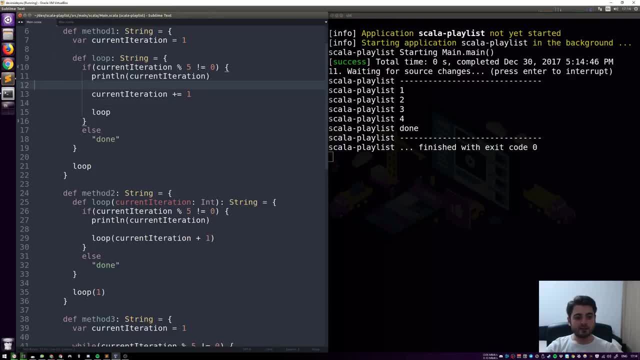 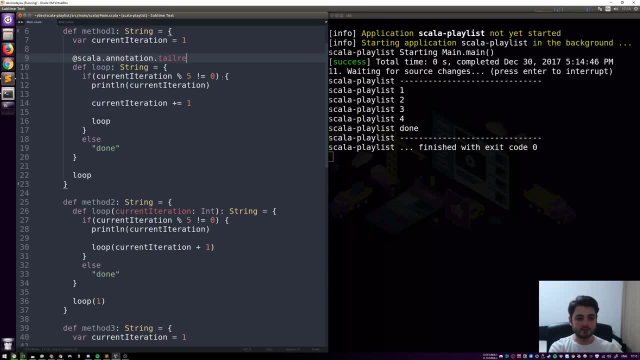 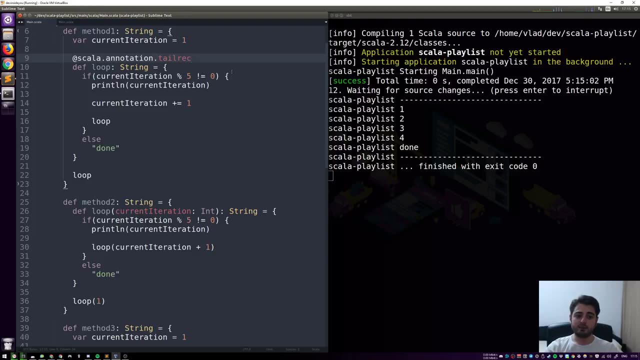 to: uh, let me, let me collapse it. okay, so you can add an annotation to a recursive function. right, you can say here at Scala, oops, sorry, Scala dot annotation tail rack right. and if it, if, if the Scala cannot convert it into a while loop, it will just not get, it's just not going to come, pop uh. 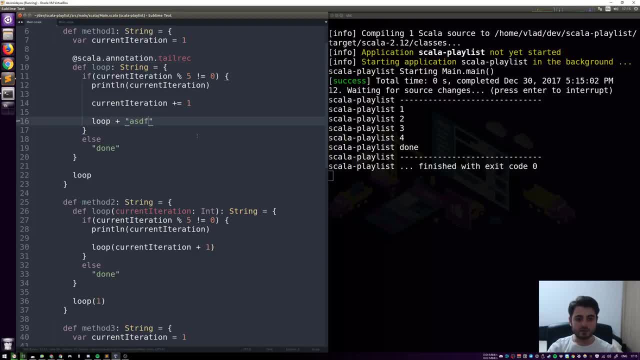 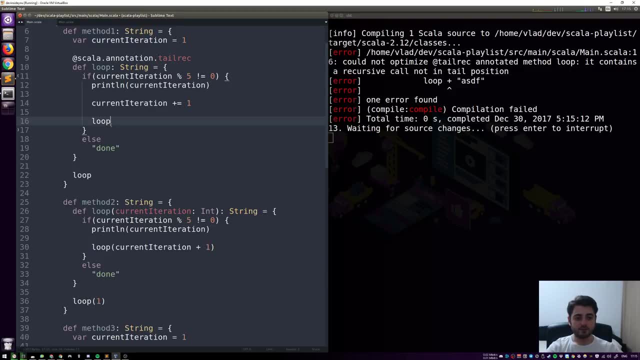 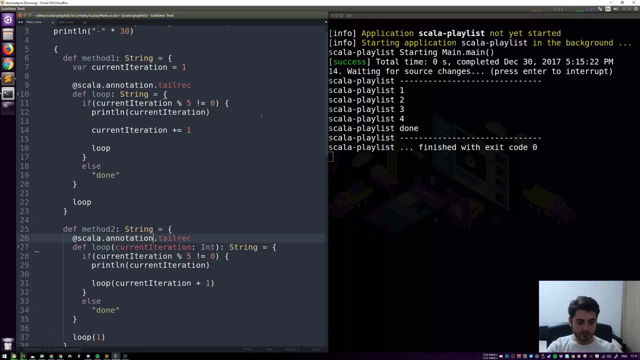 actually I haven't tried this one. I was preparing, but this should not be, uh, tail recursive right? yes, exactly. so now it says it contains a recursive call, not in the tail position. let's remove that, right. so this function is tail recursive right. This function over there, right? It is also tail. 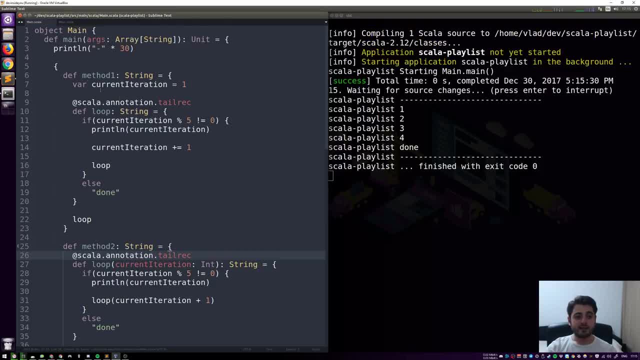 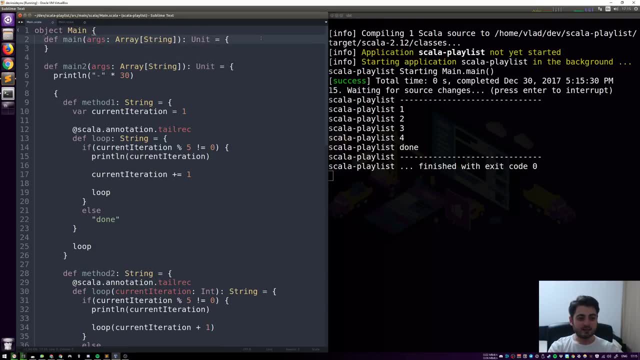 recursive right. Everything is still fine, And the same thing was over here And I haven't tried this in my preparation, but let's just try it right. So we have main and it's just going to call itself. By the way, if you don't call itself, it's also not going to compile, because it's going. 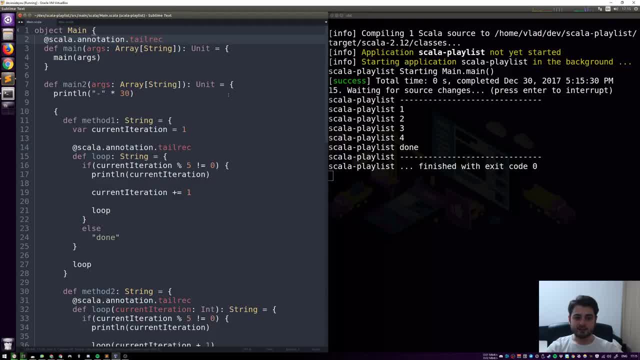 to say, hey, you're using this annotation in a function that is not doing anything, right? So, yeah, so see, it's still fine, It's a tail recursive function, right? And, as I just said, if you just print line hello world, then it's not going to be yeah, it's going to say hey. 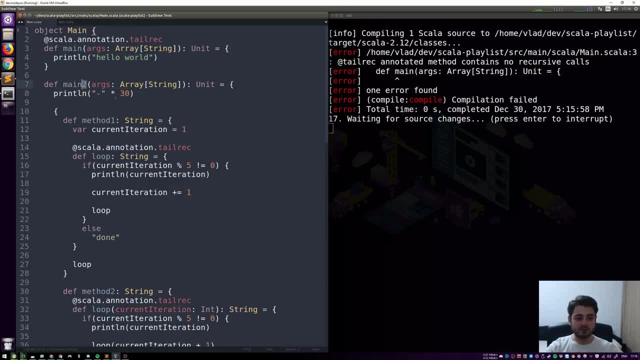 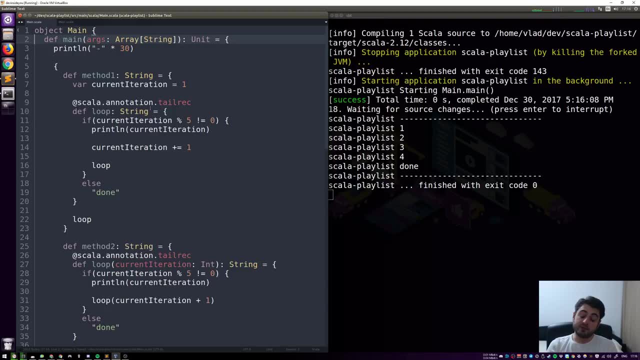 it doesn't contain any recursive calls, okay, Okay, so let me revert that thing to that. So, yeah, so if you're a beginner- and obviously you're probably a beginner because you're watching my videos- you should, when you're playing with tail recursive functions, always have this: 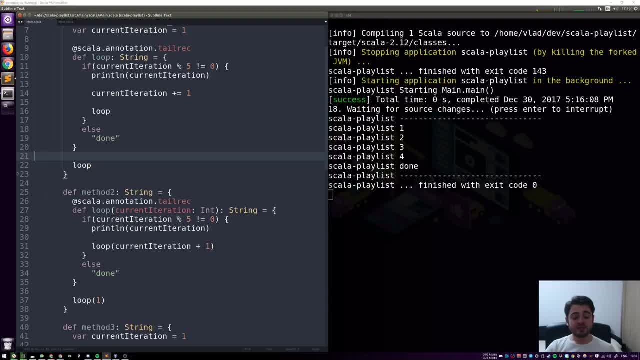 annotation, just to make sure that you didn't make a mistake. All right, so I'm actually going to have to wrap it up and we're going to have a part two of this video. Before I leave, let's sprinkle a little bit of computer science knowledge on this topic. 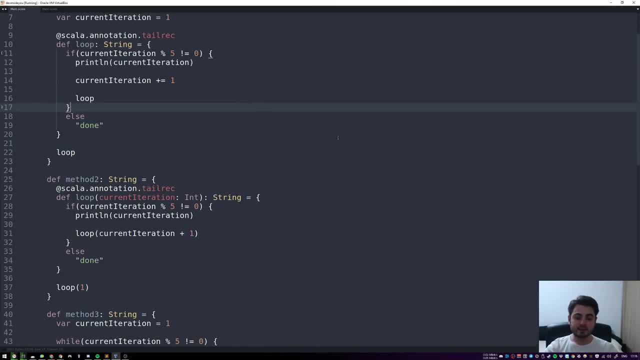 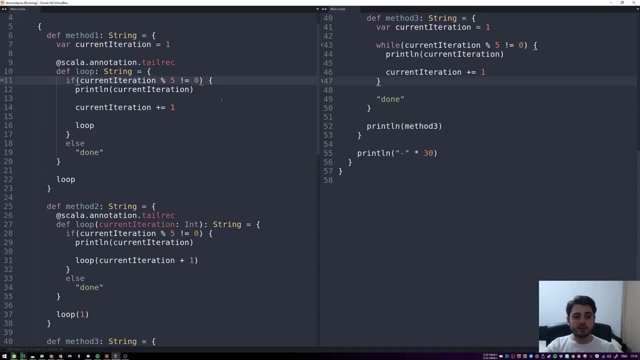 right, Let me make some mess blam again like this, okay, And let me get into the split again and to have a while loop over here, right? So question number one: is it always possible to convert a recursive algorithm into a while loop or, the same way, a while loop into a recursive? 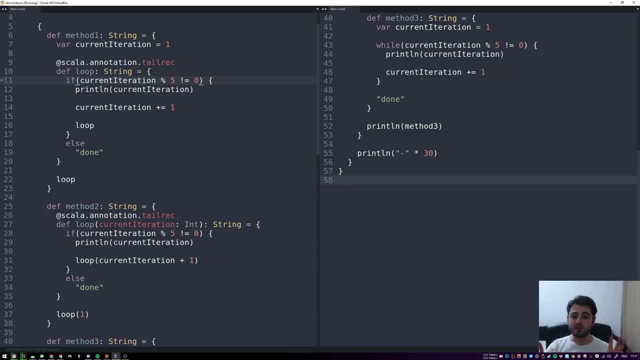 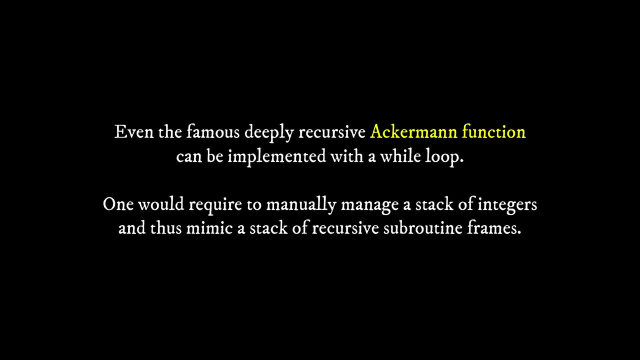 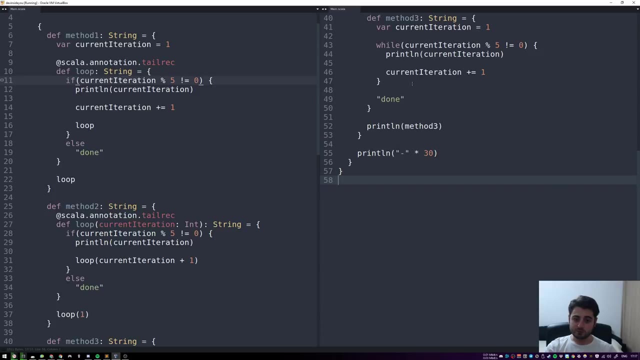 algorithm And the answer is no. So if you're a beginner and you're using this annotation, the answer is yes. So they're called isomorphic right. So there's always a way. However, is it always possible to convert a while loop into a tail recursive function?